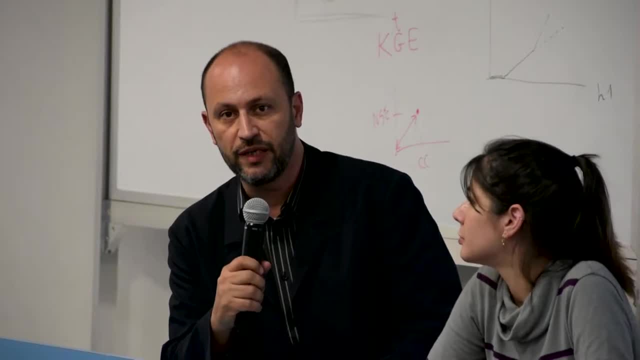 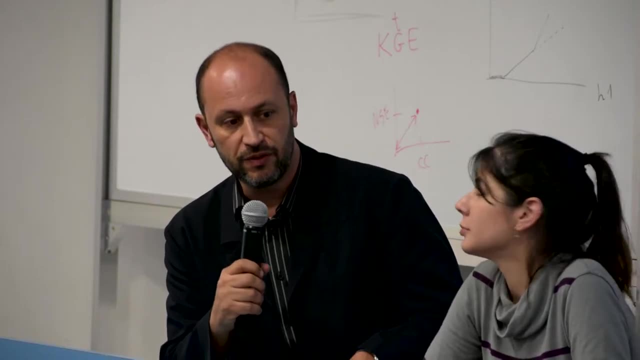 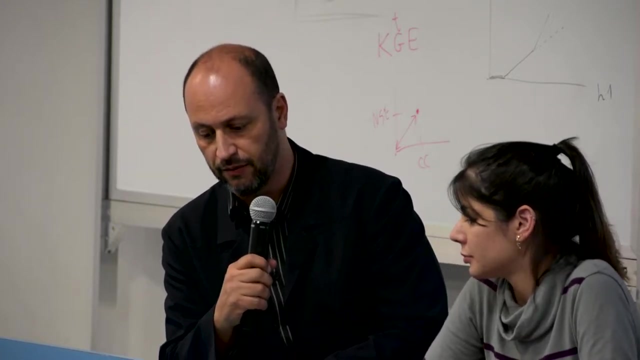 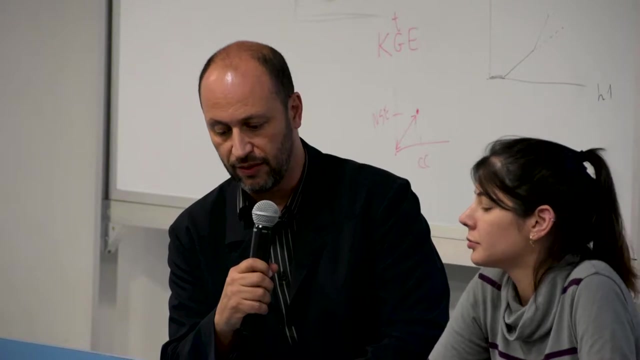 in this third module, our visiting professor, Professor Dimitri Solomattini, first time in our campus And also for this opening, we invited people representing different institutions and units of the University of Sao Paulo campus in San Carlos. Well, first of all, our director. 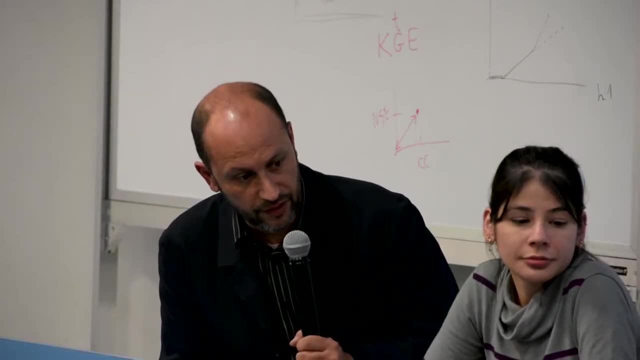 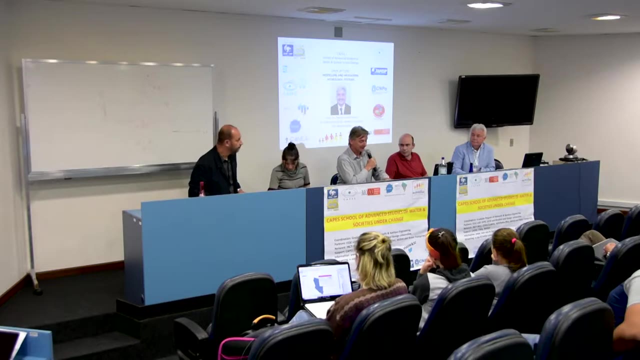 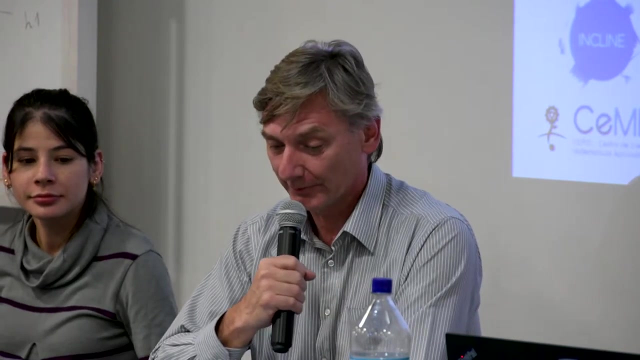 Juan, who is bringing his first words. Thank you for coming, Professor. Thank you, Professor Mangiondo. Good afternoon everybody. It's a great pleasure for us at the Engineering School of San Carlos to welcome Professor Dimitri Solomattini, who is the 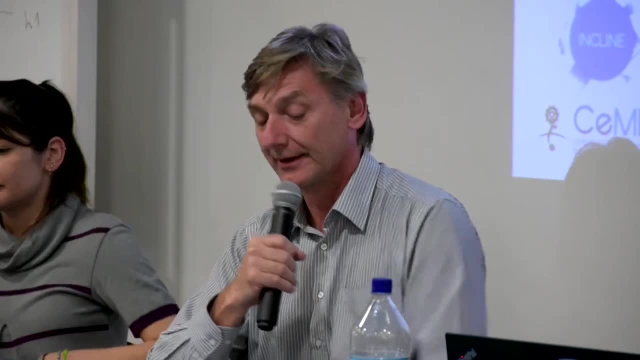 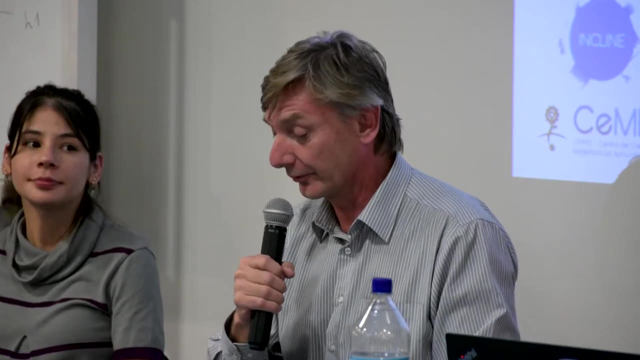 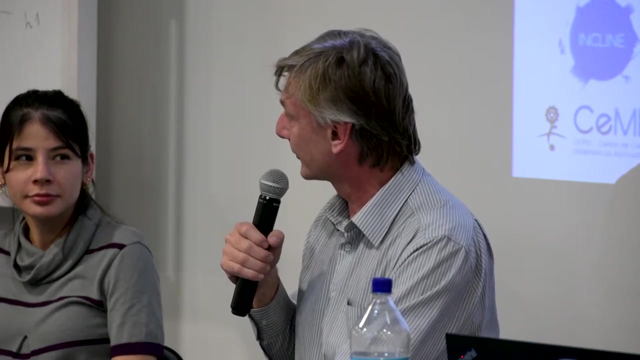 head of the Hydroinformatics Chair Group. I would like also to congratulate Professor Mario Mangiondo. Thank you, Professor Mangiondo, for the organization of a new lecture of our advanced school in hydrology and society under change, And it's really a great pleasure for our engineering. 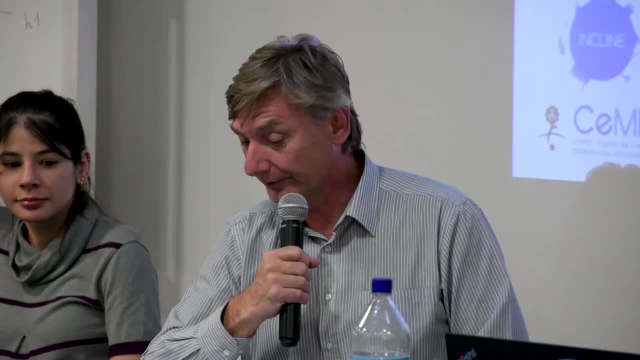 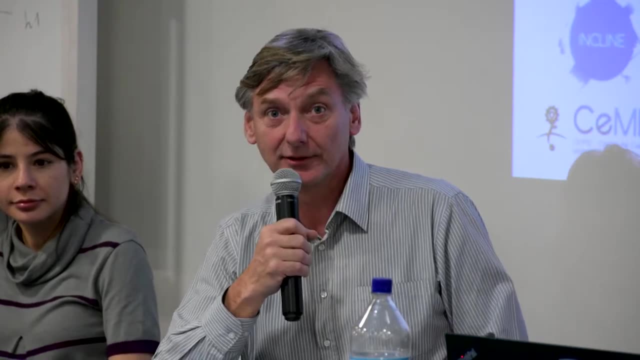 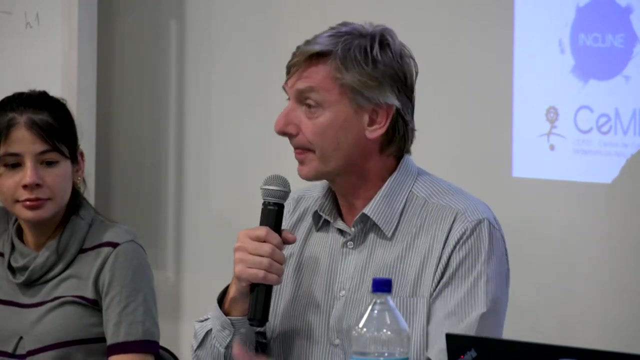 school to have so many researchers from all over the world coming to San Carlos and sharing the knowledge with our students, and even through the internet, through this transmission. So thank you very much. I would really like to congratulate all of you and welcome all of the students that. 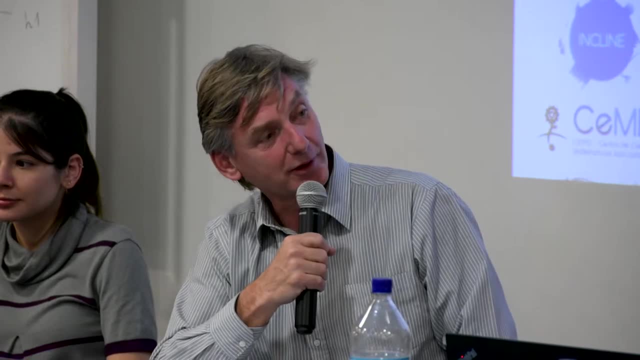 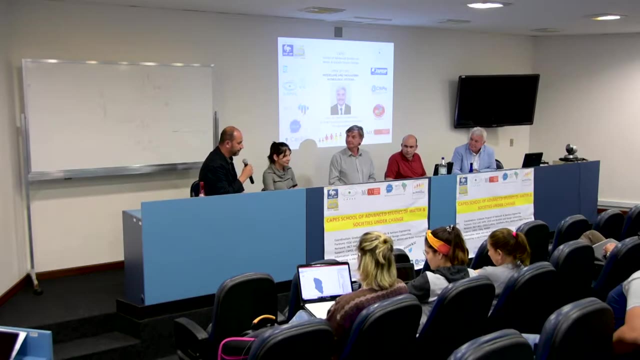 are having part on this lecture. So welcome, Professor Dimitri. Thank you, Obrigado, Professor Edson Velland, director of the School of Engineering. Also, this event is promoted by CAPES and also partially by FAPESP and CNPQ and also several interdisciplinary 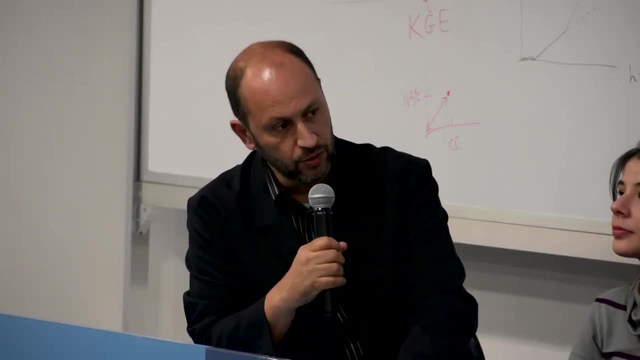 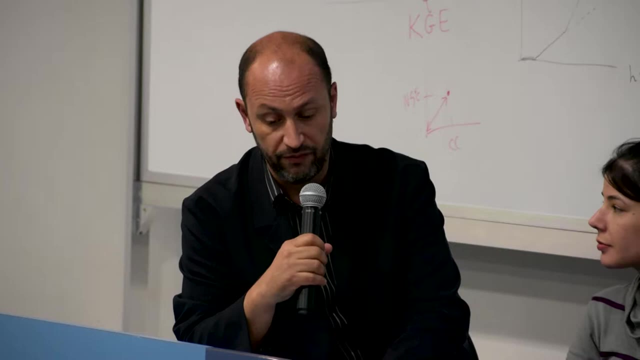 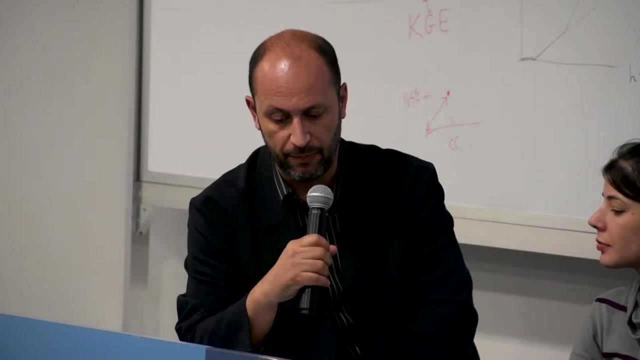 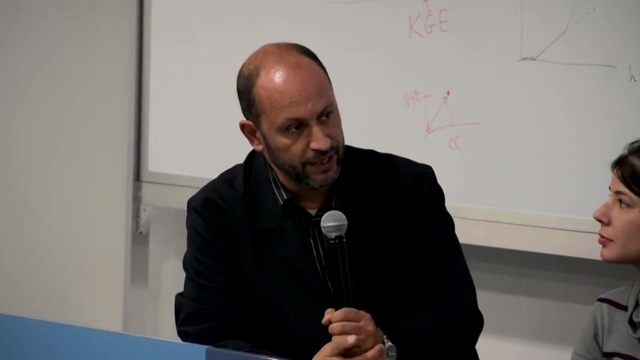 groups and for the academy. One of these groups is the Research and Innovation Center of Applied Mathematics for Industry, the CMA-ICPIT, hosted by our Institute of Applied Mathematics and Computing Science in this campus, And also Gustavo Faria is on behalf of this center. 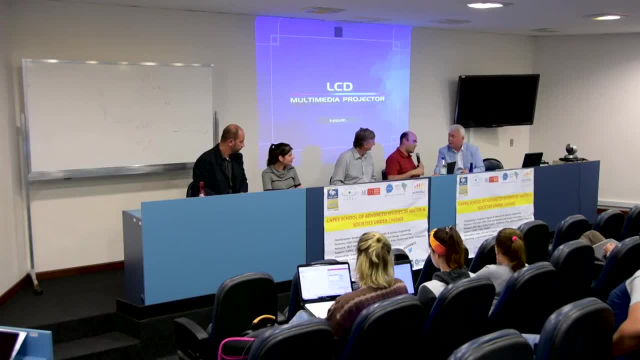 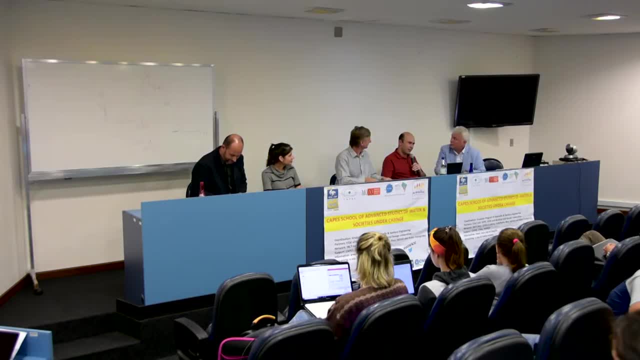 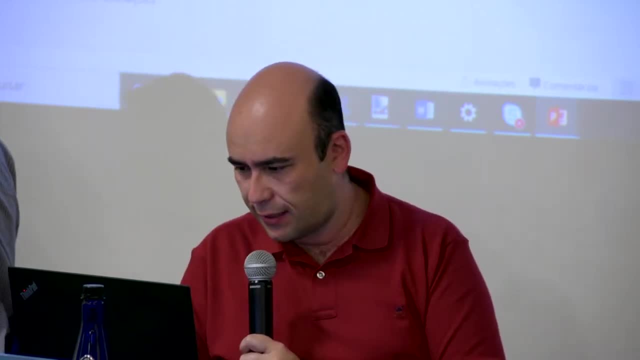 University of San Carlos University of San Carlos. University of San Carlos University. I'm giving you a chance to speak quickly, So I couldn't speak so fast in English about the CMA- and I think it is, but my presentation is in English so I think it will get easier to understand. 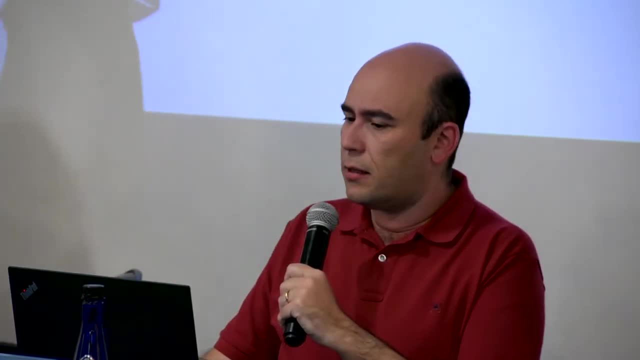 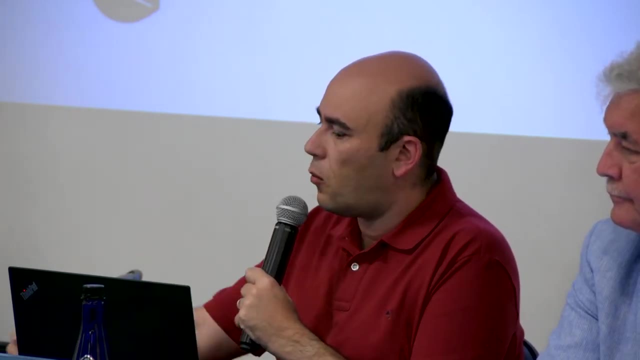 I'm going to get down there to see the slides. Perfect, There is. here in the campus of San Carlos, we have a CEPID, right? Actually, there are three CEPIDs here, right, Which is the largest project that can exist at FAPESP. 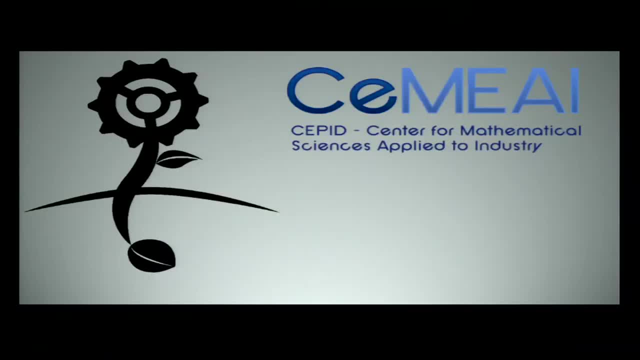 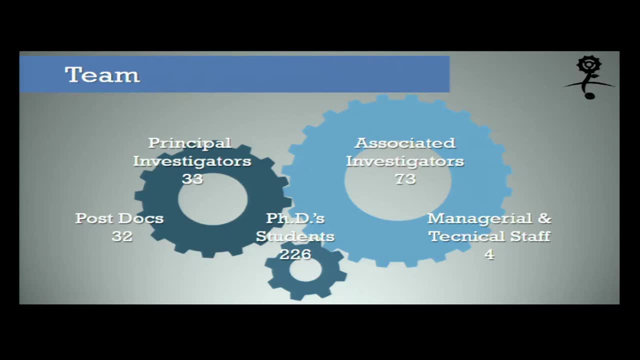 There is one here at the Instituto de Ciências Matemáticas e Computação, and there are two in Physics. I'm going to talk about this one. The team is made up of 33 professors who are Principal Investigators, who are the main researchers, and 73 associated researchers. 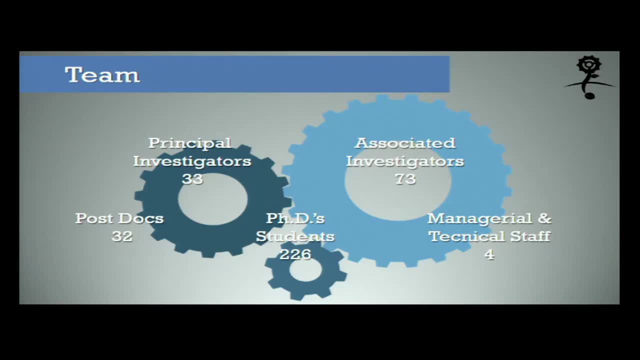 Among these researchers, we have two here, Professor Mário Mediondo and Professor Edson Wendland, who are also CMEI researchers. We have these numbers of postdocs, of PhDs. they vary every day new ones arrive, some leave. 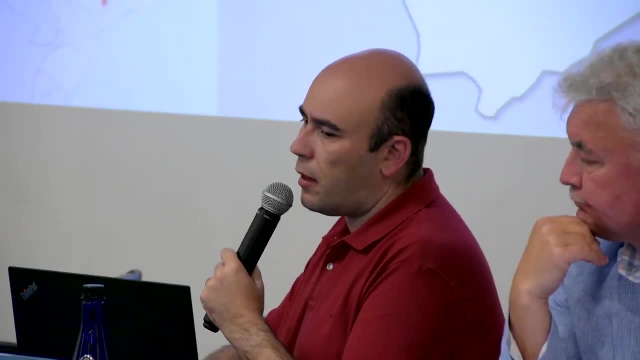 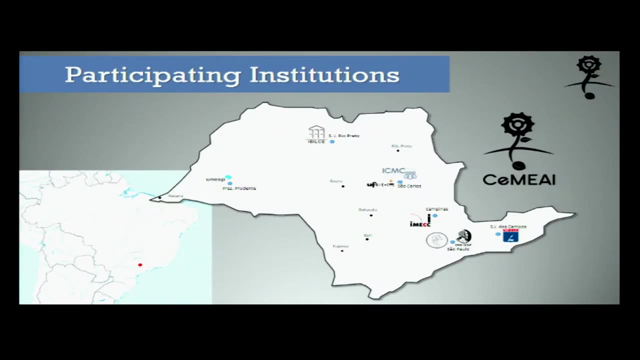 so it's more or less this average that we have. It is spread throughout the state of São Paulo. the headquarters is here at ICMC, but we have professors at ICMC, at Federal, at UNESP, in Bauru. 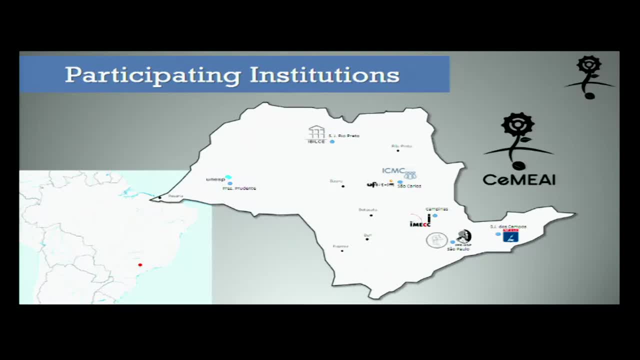 in Rio Preto, in Botucatu, we have in São Paulo, at Poli, at IME, we have at IAE. The current president of CNPq is a researcher at CMEI, at UNICAMP, at IMEC. 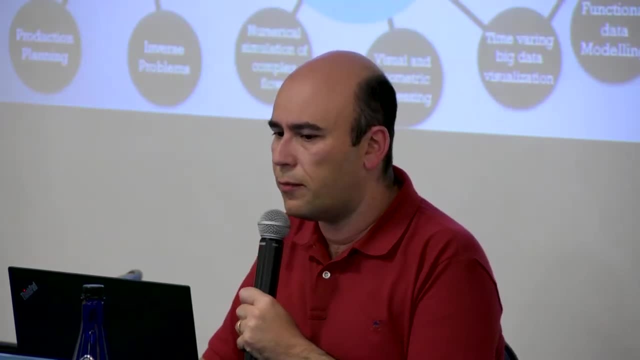 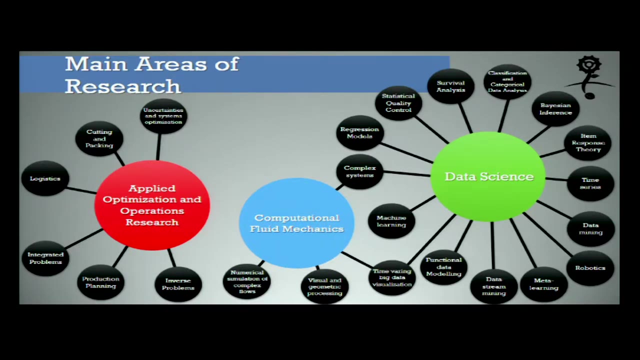 so we are spread throughout the state. The main areas of research at CMEI are these three: the area of optimization and operational research. so we have several sub-areas Within this. I will not go into each of the little balls because otherwise it will not work. 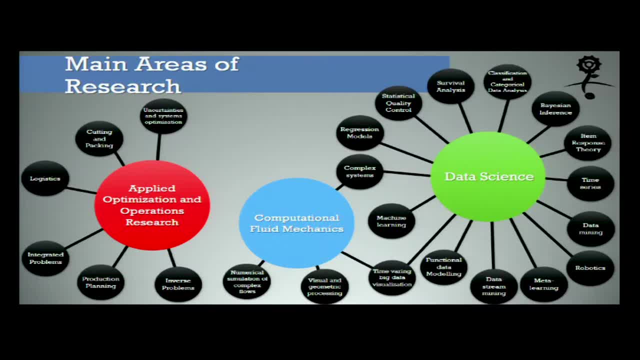 We have the area of computer fluid mechanics, which makes simulation of scoring and so on, and we have a large area now of data science. Why is this area so large? There are two reasons. One, because there were two areas before that ended up joining, which was an area of risk analysis. 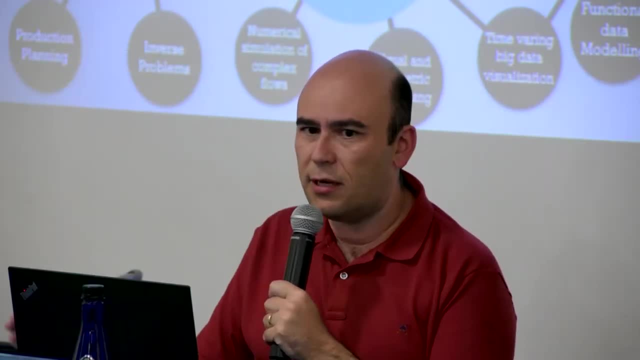 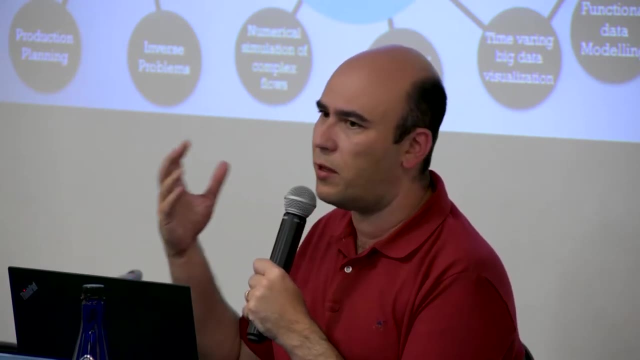 where the statistics and the area of artificial intelligence are, but as there were two areas before that ended up joining, which was an area of risk analysis, where the statistics and the area of artificial intelligence are, but as there were two areas before that ended up joining, which was an area of risk analysis, 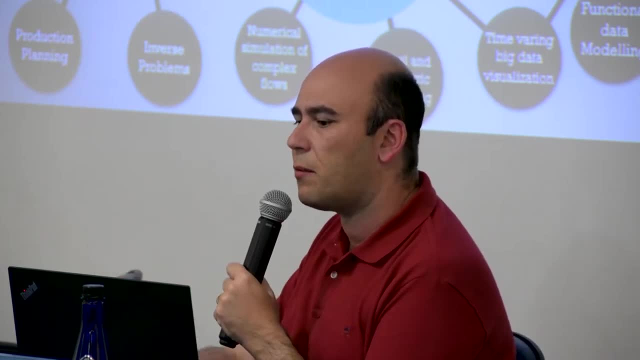 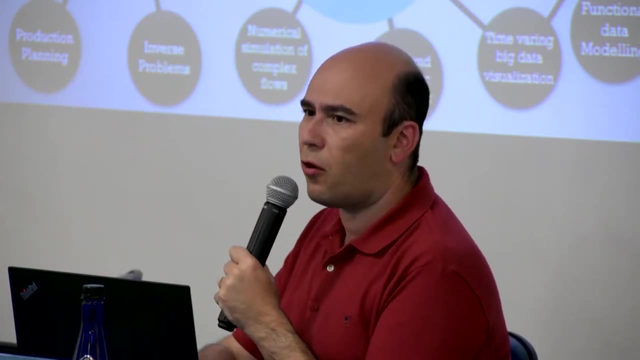 we ended up joining this on a large data science group, which is also something that is in vogue. we ended up joining this on a large data science group, which is also something that is in vogue. To help this research, we have a supercomputer for researchers to use. 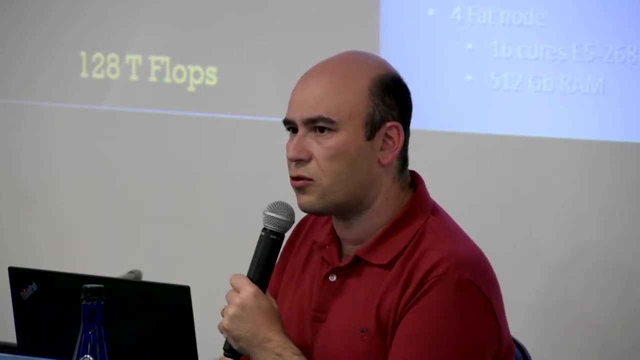 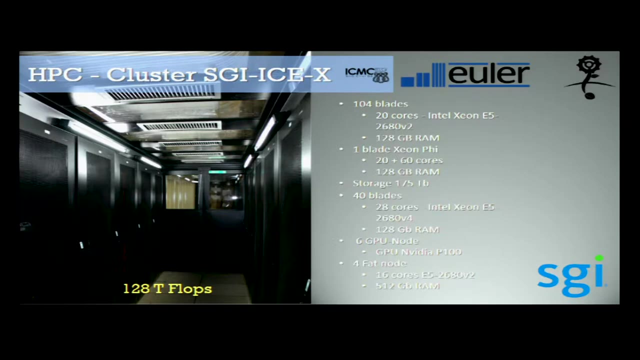 in fact, others out of CMEI may also use it, and we developed this갈. This computer is the second with the highest performance in public universities in Brazil. It will be doubled. this is its capacity, and when it is doubled, it will be the number one. 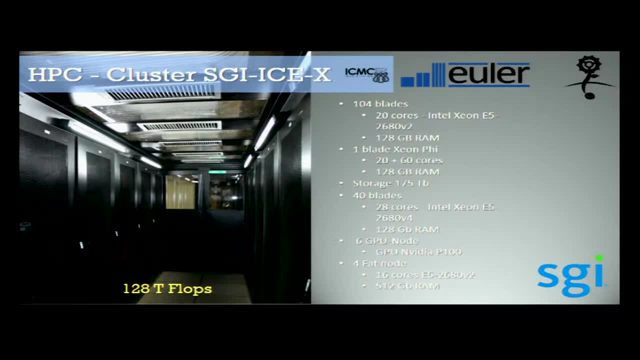 The number one equipment today from Petrobras is very new. it has just been installed. The number two from Petrobras, I think it was 260 teraflops, Just so you have an idea. the most powerful equipment in Brazil today is this new one from Petrobras. 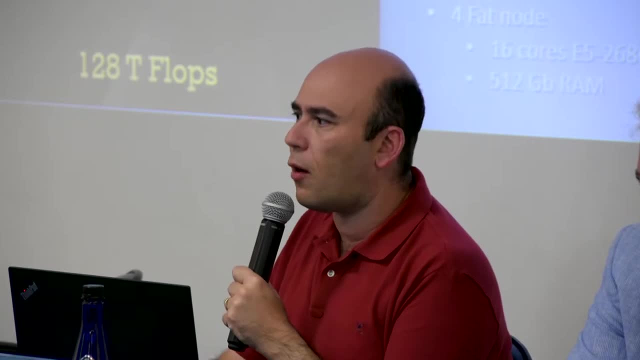 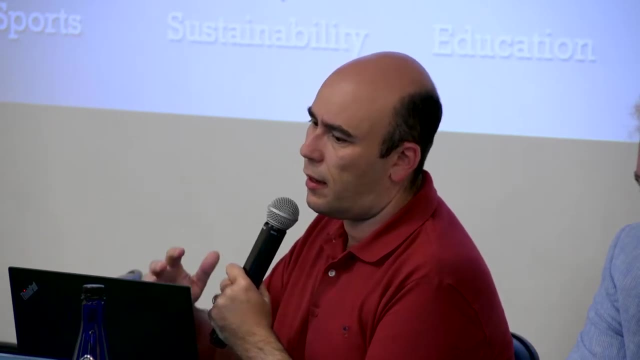 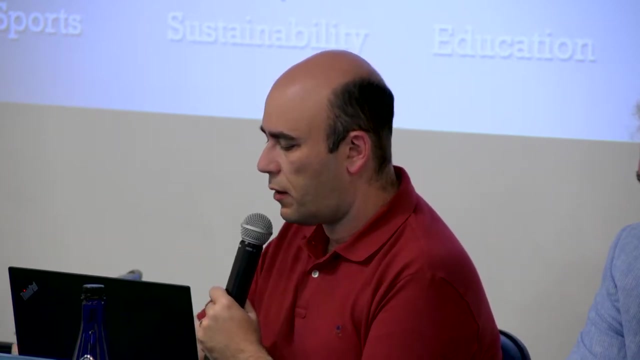 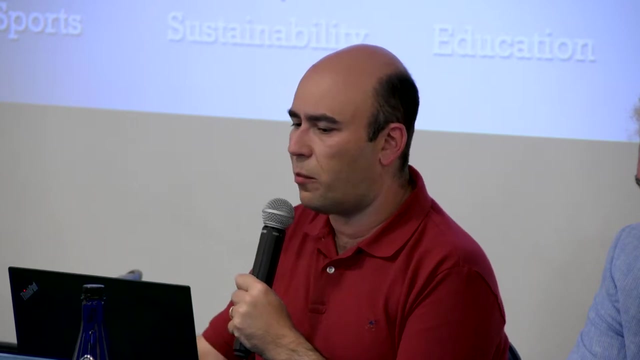 What they are replacing is what we will have. So it is something very, very important for research And the CMA has those areas of research but it has the areas of study where we look for business problems. So it goes from the industry, the base industry, the manufacturing industry, 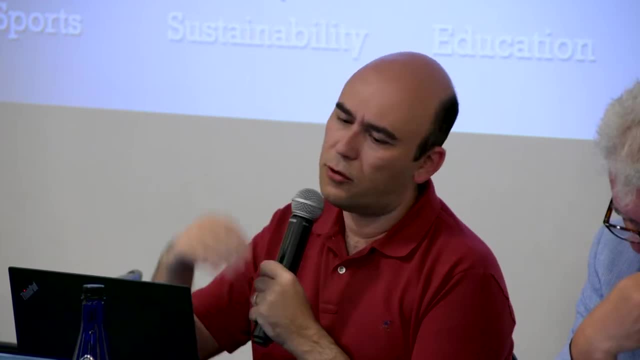 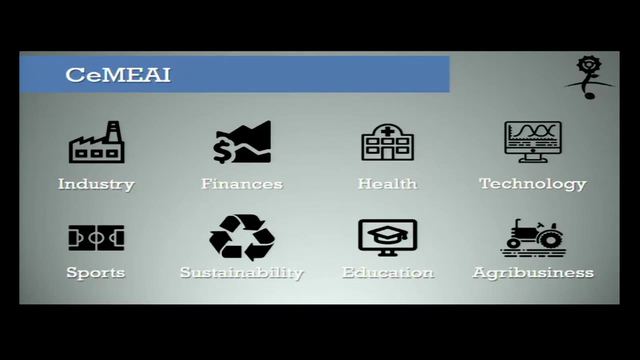 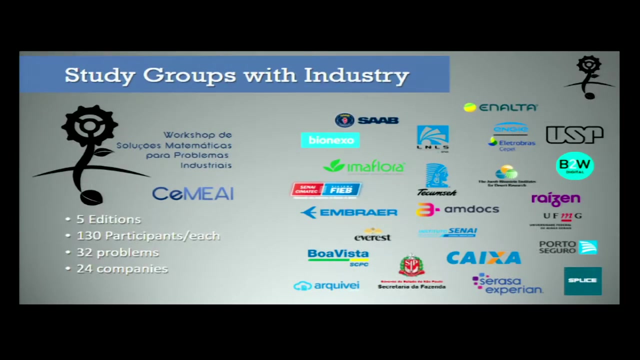 the industry with the little fireplace, as well as the financial market. health, We have some projects with technology companies: sports, sustainability, education, agribusiness And- one thing that I think is interesting for you- we have an event here. 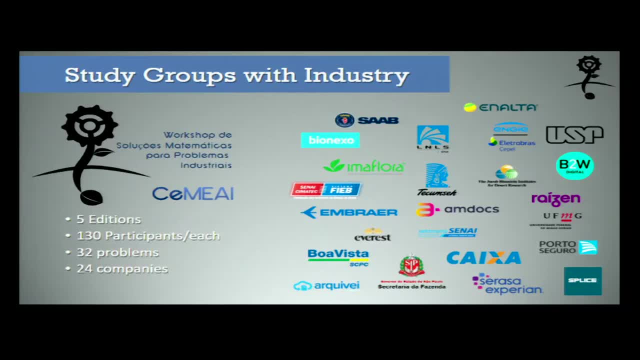 which are the study groups of industry. What is this? We bring companies. there are usually five or six companies. they bring a real problem and it stays for five days more or less. it is 20 to 30 participants per problem to solve the company's problem. 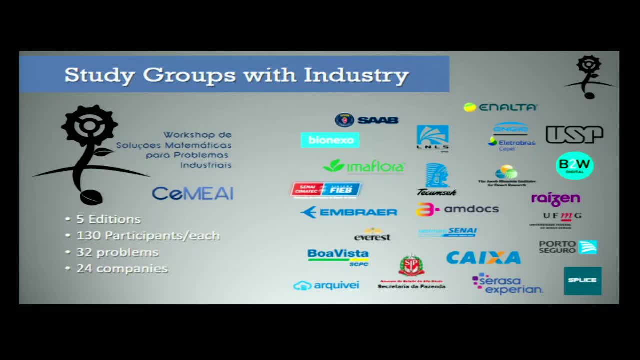 It is very interesting because it is a well-applied problem. There are people who compare it with a hackathon. I think the main difference for a hackathon is that a hackathon is a dispute between groups to see who will make the best solution. 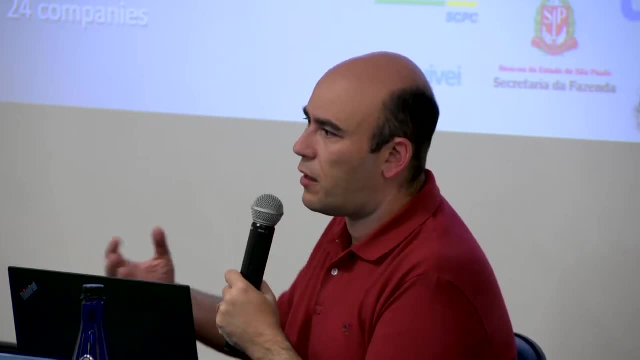 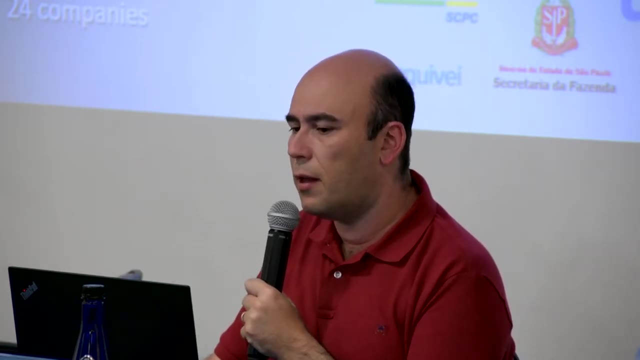 In this case, it is not to present a solution. sometimes there is more than one approach, so there is more than one solution, which can sometimes be added or not, but it is a way for us to relate to companies and they know the work. 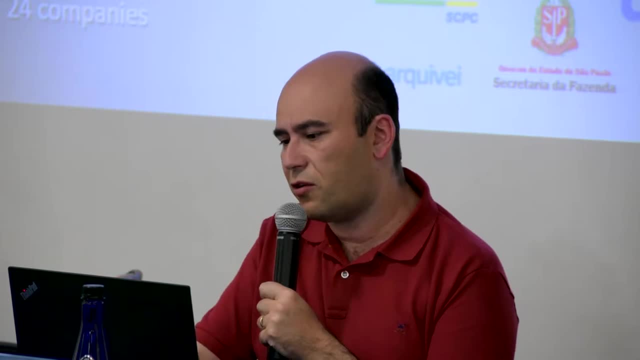 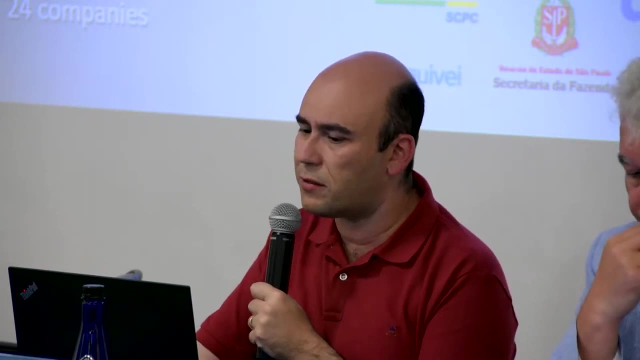 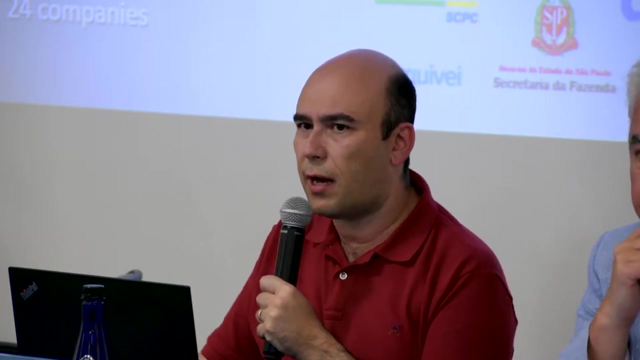 and the research that is done at the university. As you can see, we have giant companies there: Raizen, for example, which is the fourth highest-paying company in Brazil. We have Embraer Caixa. As we have smaller companies, sometimes local startups. 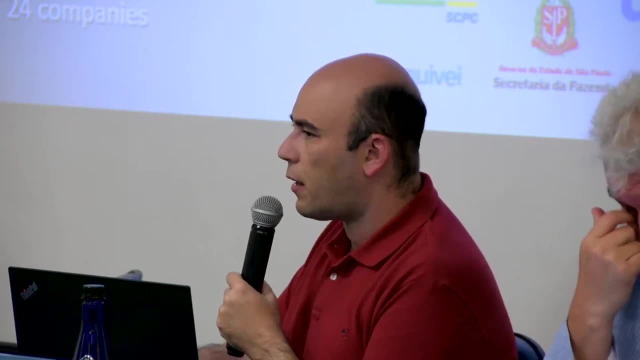 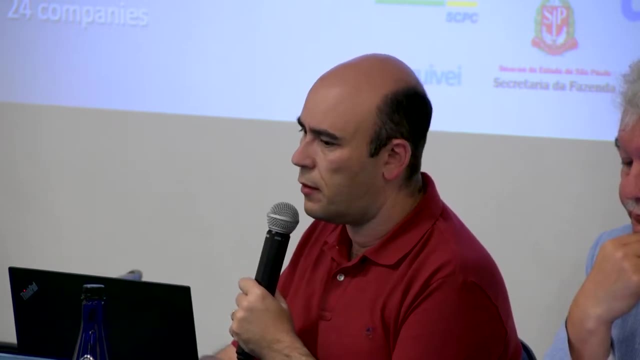 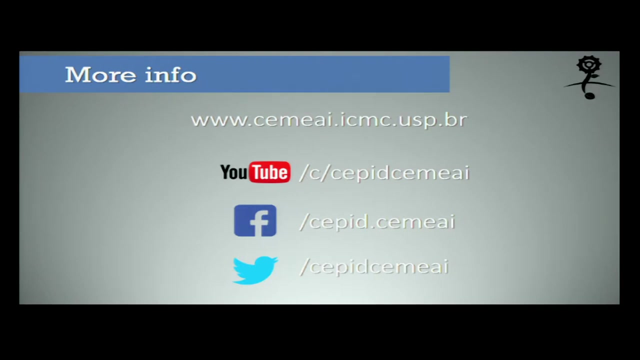 we also work with them And the participation of post-graduates mainly is fundamental for the success of this event. I had to be very brief. This is a summary of a longer presentation where we detail the areas. but who wants more information? we have a lot on the site, on YouTube, on Facebook. 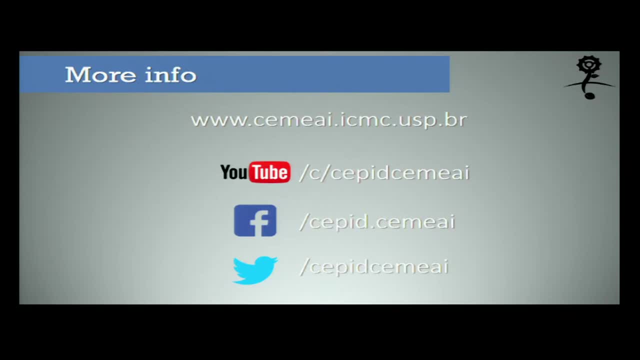 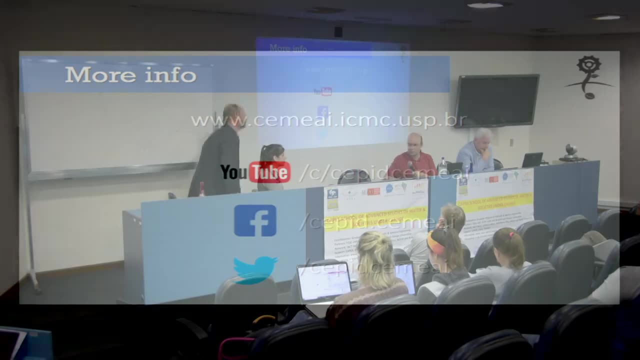 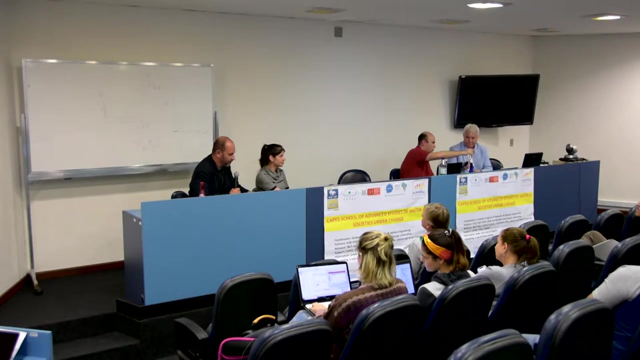 so we put the projects. We have videos with the projects where we try to explain in a simpler way the work that is done. So I think that's it. Thank you, Gustavo. Thank you Also. I would like to thank Maria Clara Faba on behalf of our students. 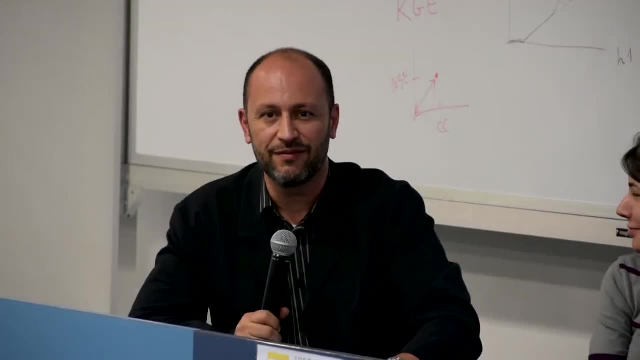 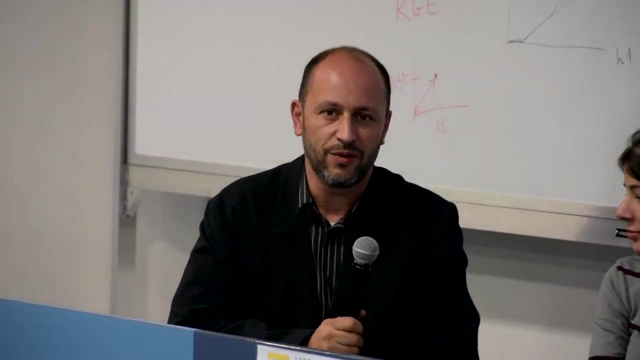 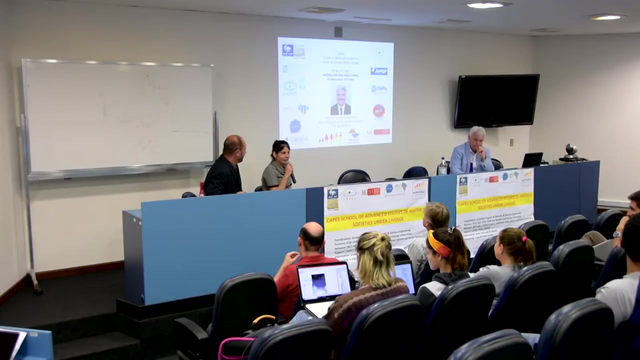 because our clients, our customers, first of all, are our students. So Maria Clara is also hosting, co-hosting, this course as part of her PhD. So your words. So I just want to say thank you for you, for University of São Paulo. 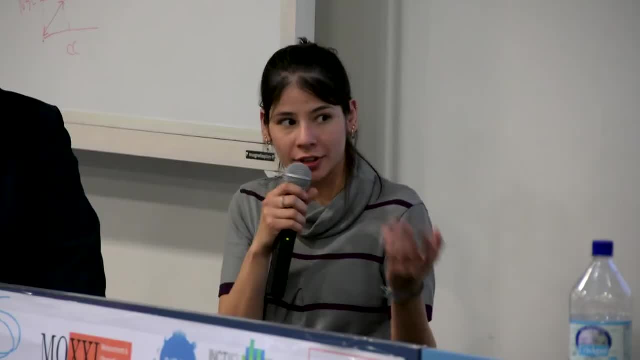 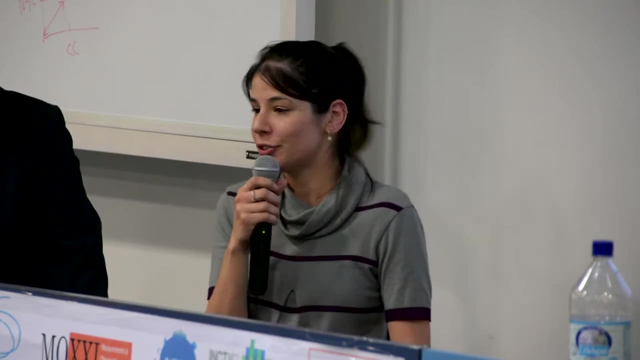 and CAPS to give the opportunity to Professor Dmitry lecture to the students here And mainly, thank you for Professor Dmitry to accept to come here and enlighten us a bit more about modeling and hydroinformatics. Okay, Thank you, Maria Clara. 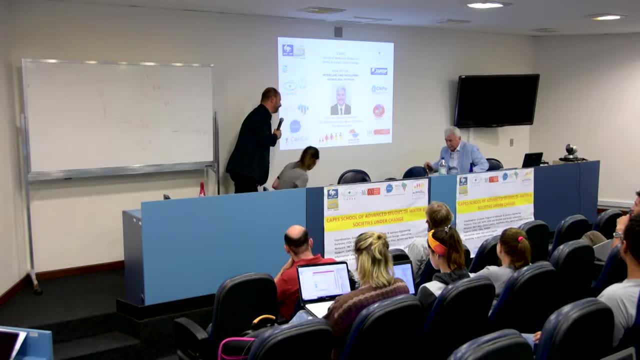 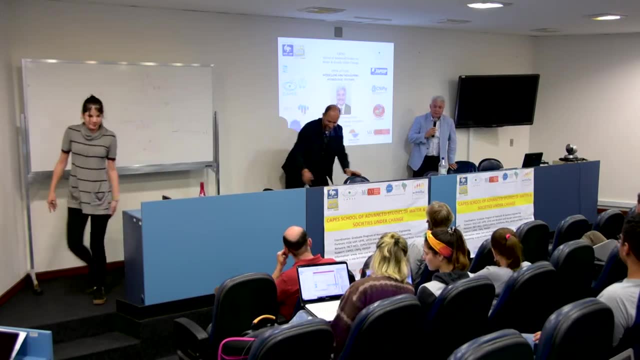 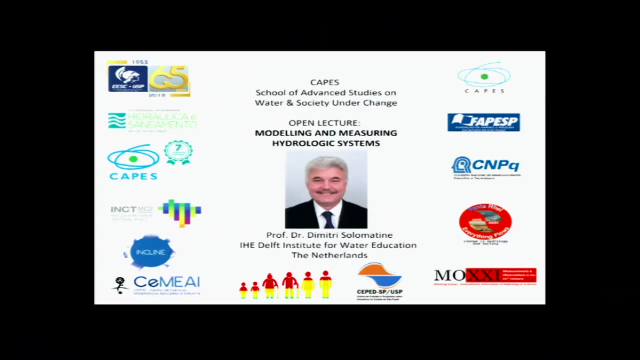 Thank you, Dmitry. The floor is yours, So thank you for coming and the open lecture is open. Colleagues, I feel embarrassed to see this slide because you put my face in the middle of so many different organizations. By the way, microphone is working. 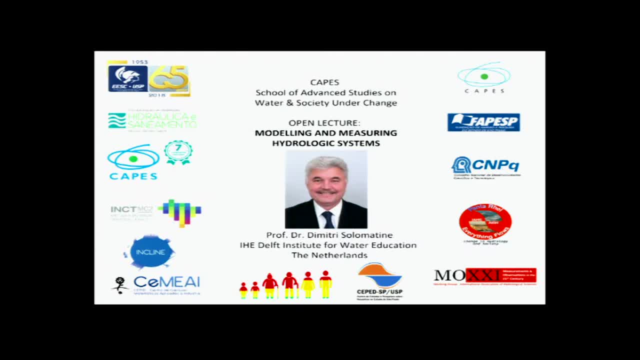 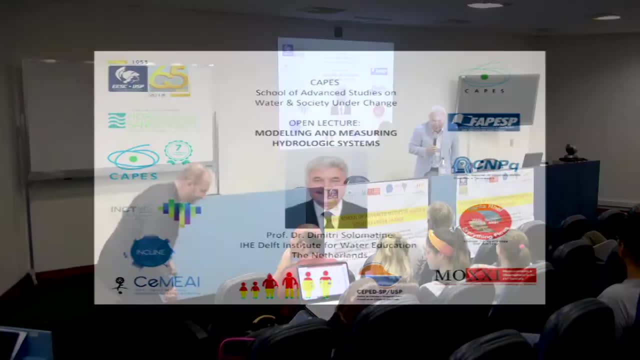 I don't think so Yes, it does. And now it's okay, Same, All right. Thank you very much, professors, for coming to this lecture. It was a bit unexpected, so I'm not sure I'm prepared well. 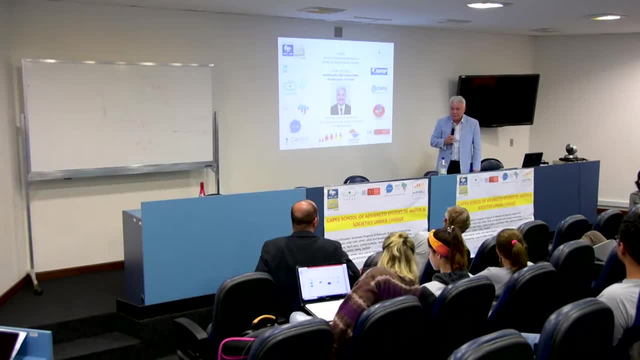 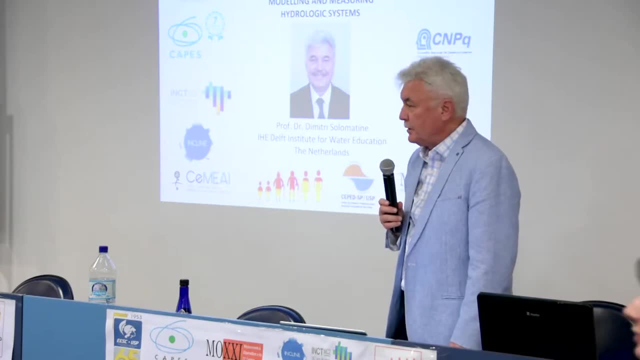 But I put some slides together And, Professor Mendiondo, thank you for inviting me. I really appreciate this opportunity to visit University of São Paulo, which appeared to be the best part appeared to be in São Carlos, So thank you very much for this opportunity. 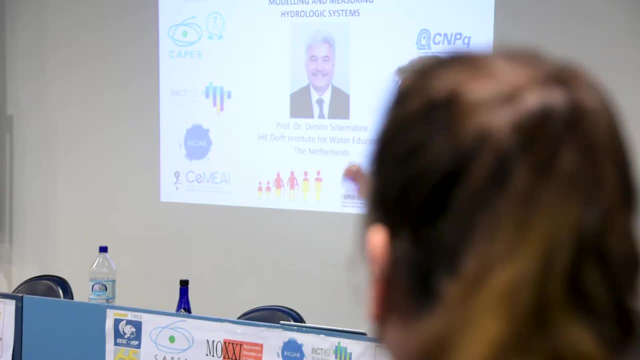 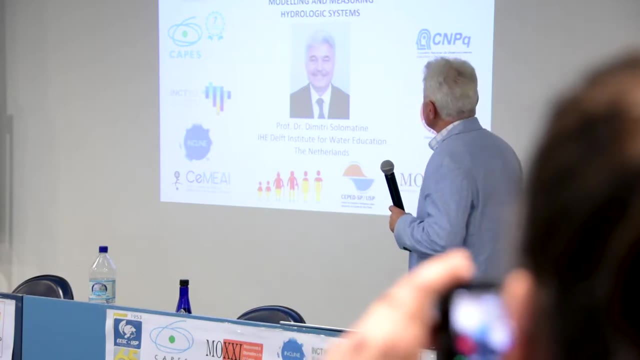 So actually, I see I looked at this slide for the first time five minutes ago and I tried to find out what attracts me in this slide. It's not the center, of course, But I like this symbol of chaotic behavior of a certain system. 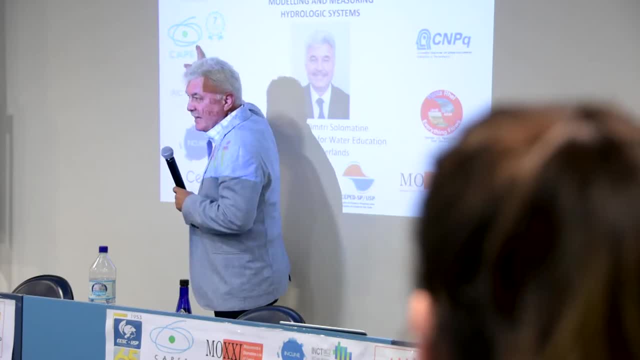 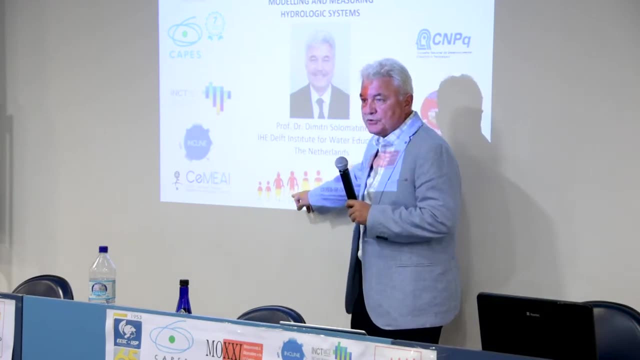 as if it's an attractor, and this is, you know, sort of predictive chaos a bit. This is what I like, This is what we do in life, And also I see my role. So I'm this person here who came to teach this other younger generation. 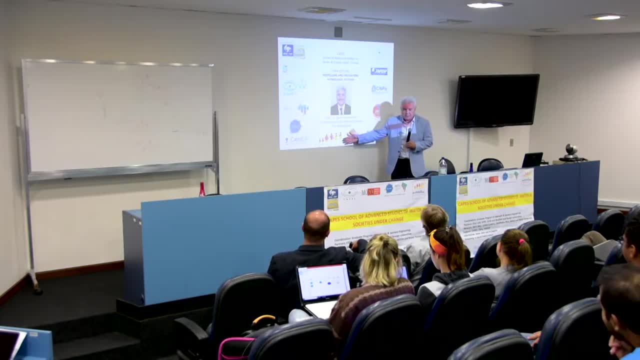 So I liked it a lot. I'm not sure what this symbol means, but perhaps it means elderly people giving you know knowledge back to young generation, And I'm sure young generation would pick up all these ideas which we are presenting here. 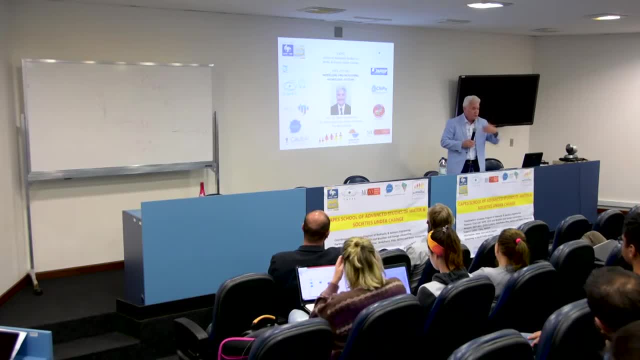 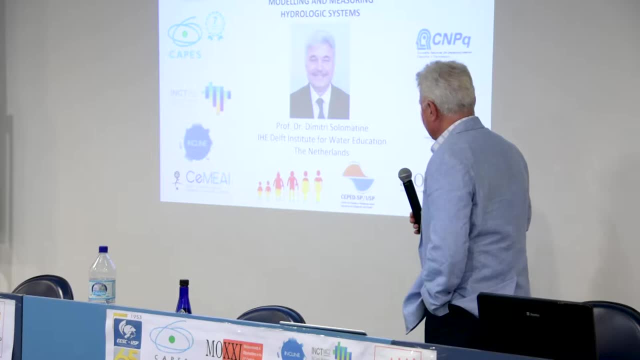 and develop them further, And that's really what charges my battery to communicate with the young people. So really great. So thank you very much for yet another opportunity to come and to talk to the growing researchers, master and PhDs Right. 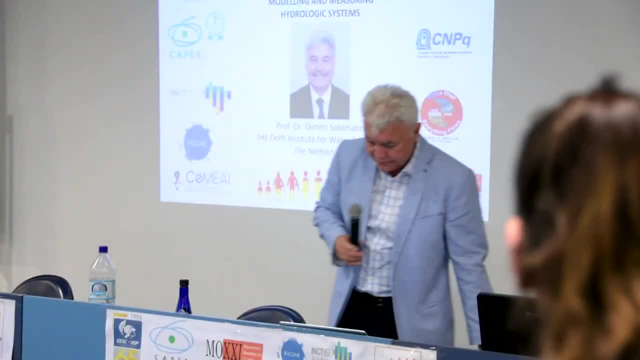 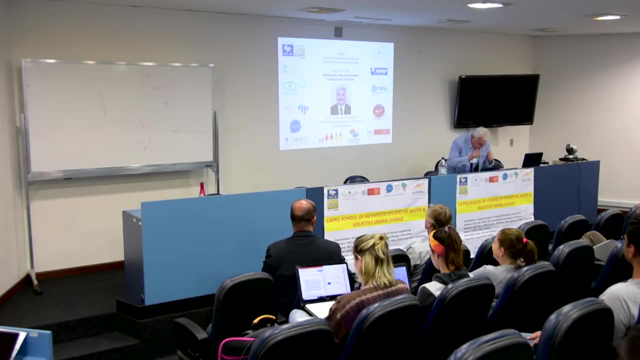 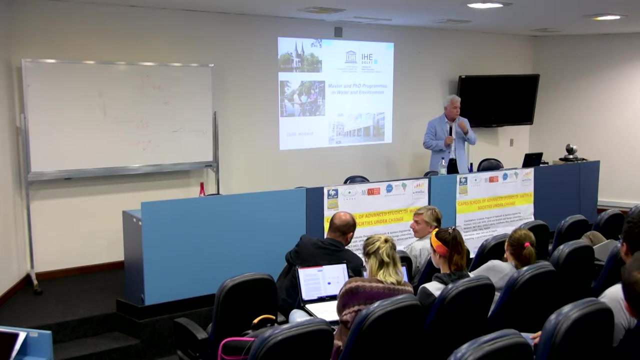 But my role now is to talk about hydroinformatics And I would now switch. Sorry, I put my microphone and switch to something else. Several words about our institute. You can consult education training guide. Come to internet. You'll find a lot of information on YouTube. with all these channels. 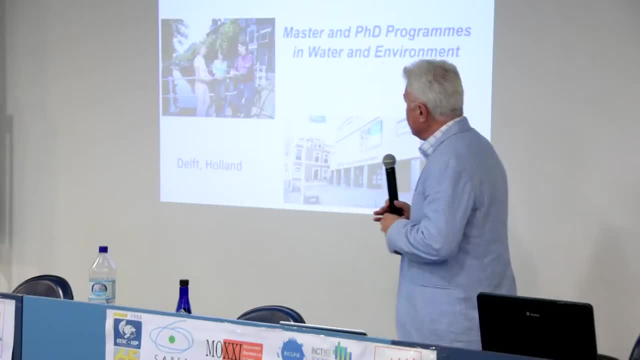 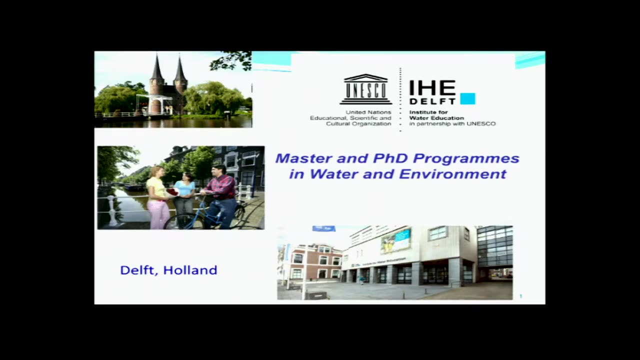 reminiscence of students, what they did, and so on. So we are located in Delft, in the Netherlands. So you see nice places in the Netherlands. This is our new building. I'm not sure I like it, but okay, fine. 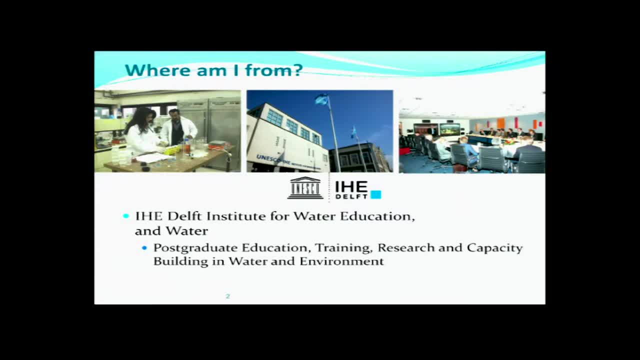 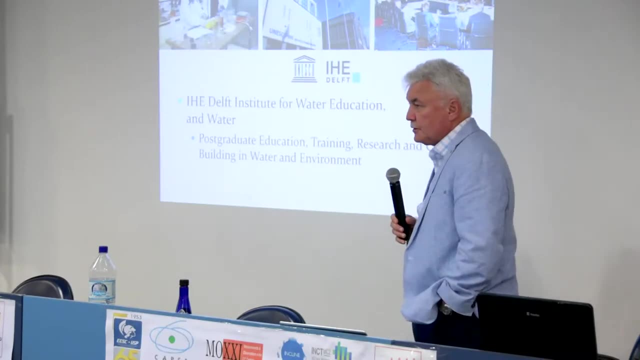 At least good people work in it. So we are postgraduate education, training, research and capacity building institute working in the area of water and environment. We don't have bachelor programs. We have 200 people in the institute overall and around 100 academic staff. 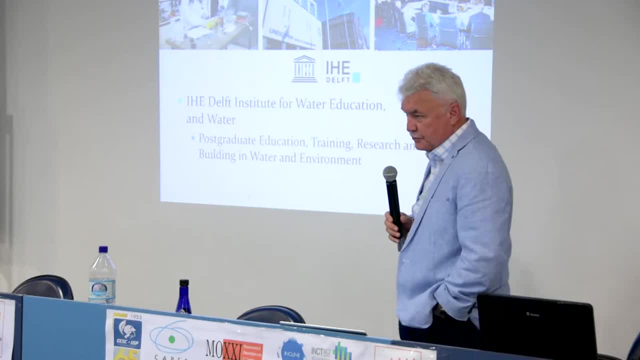 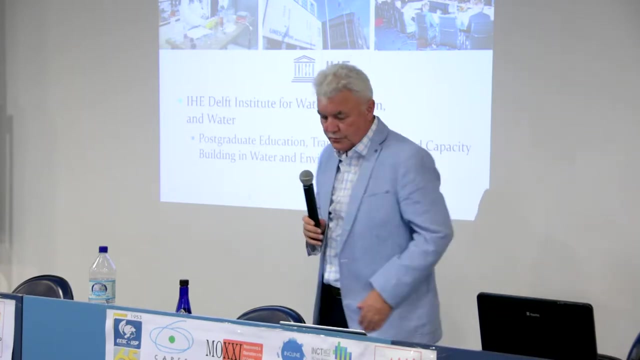 We train every year. We have around 200 master students, starting every year 200.. We have 120 or 140 PhD students at this moment And overall we train 700 to 800 people. also, if we include short courses and so on. 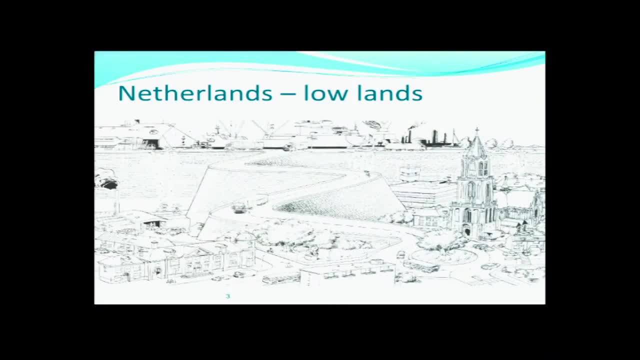 So we have a lot of alumni: 15,000 alumni around the world. We train people from developing countries or countries in transition. I shouldn't say developing countries, I should say maybe non-Dutch, because we don't have Dutch students. 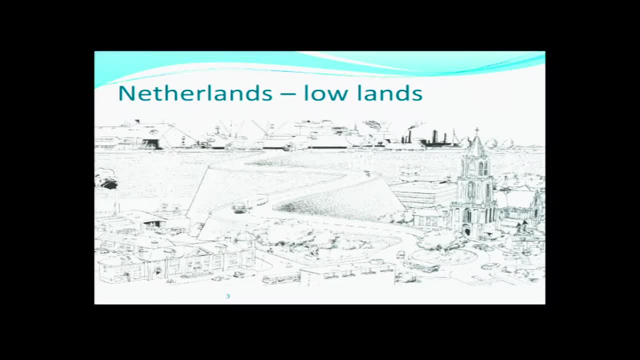 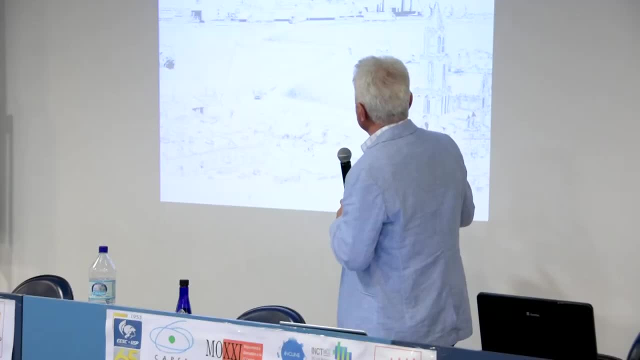 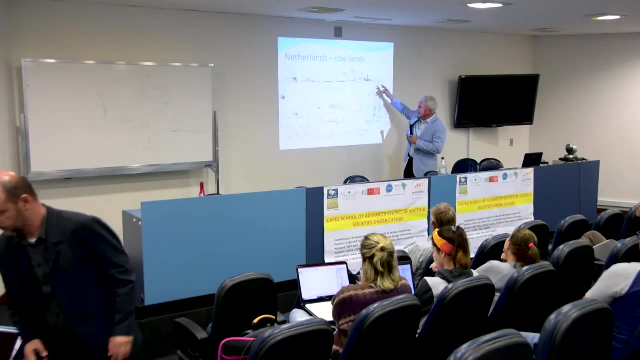 But we have students from all over the world every year- 65 countries, people coming from 65 countries- Netherlands, low land- So maybe that's why this institute is in the Netherlands. It's a large transportation hub. We have largest port in the world- Rotterdam. 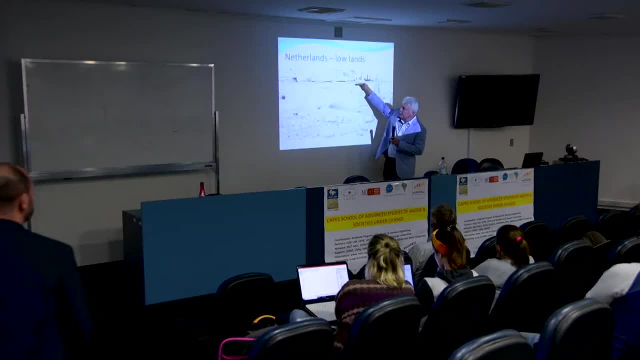 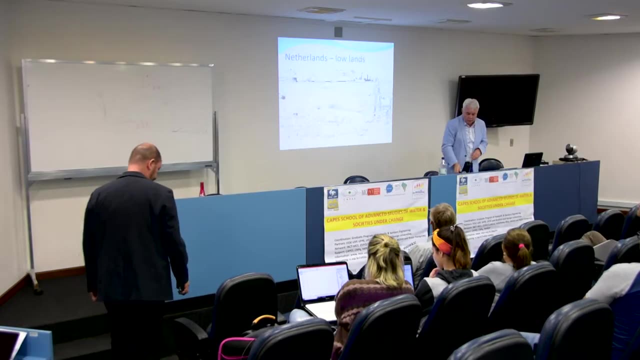 We have a lot of infrastructure but also a lot of water problems because water stands that high. You maybe know that- why Dutch are so tall. You know Dutch people are very tall. They look at the sea like this. you know That's why they grow so high. 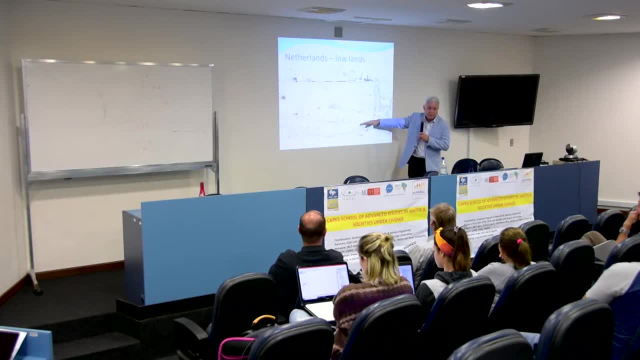 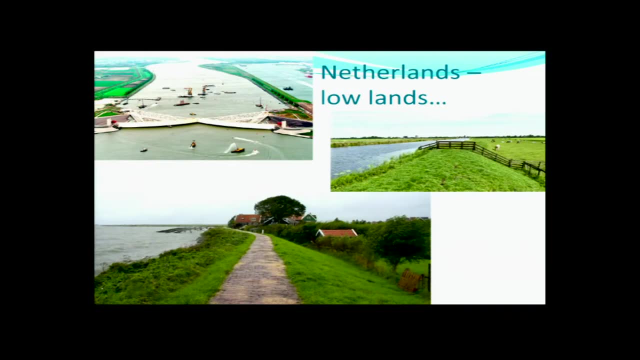 You see, the Dutch industry is located below sea level- one-third of the country- And most economic activity is below sea level. So if something happens, then we're in trouble. So this is largest storm surge barrier in the world, I think. 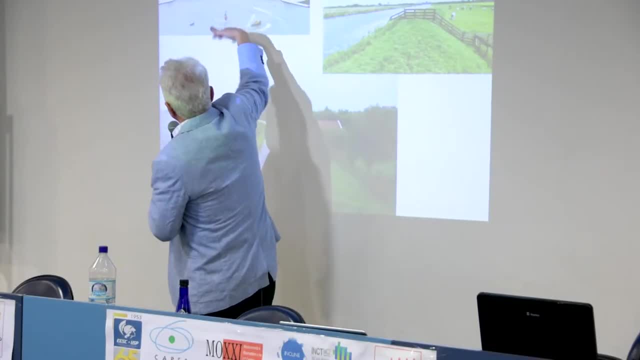 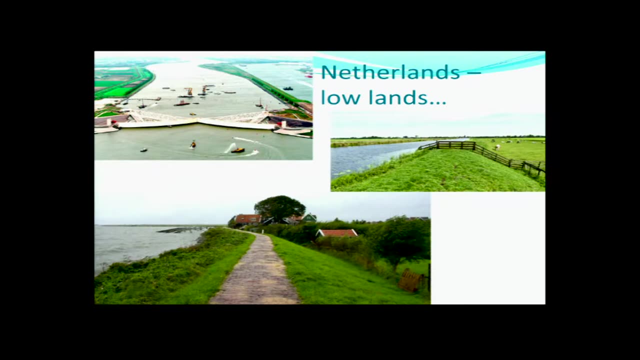 It closes entrance from the ocean this side to enter high waters, surge waters into the Rotterdam harbor, So to prevent floods And it's 10,000-year protection from coastal flooding. And you see, the houses are below sea level. 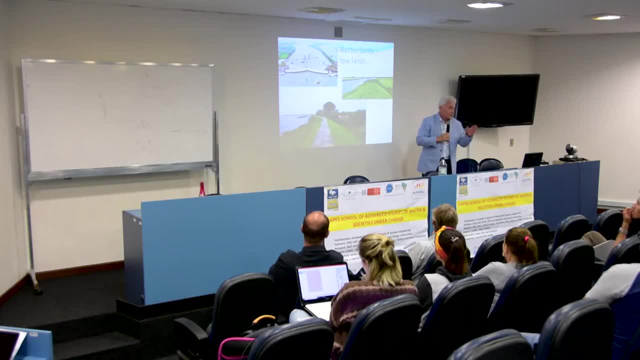 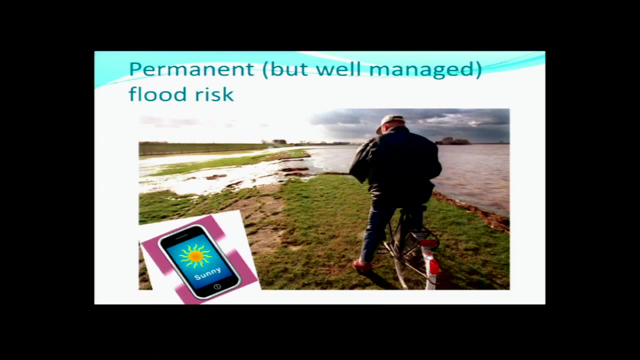 So these pictures you see when you ride the bike. Maria Clara could tell you that it's really wonderful landscapes, But you see what may happen. Sun is shining but lake is breaking, You know, flood waters. This is citizen observatory. 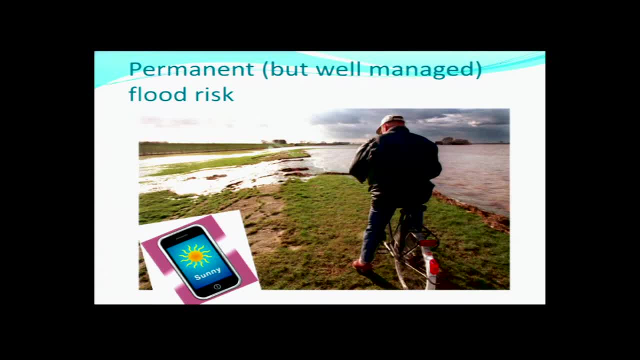 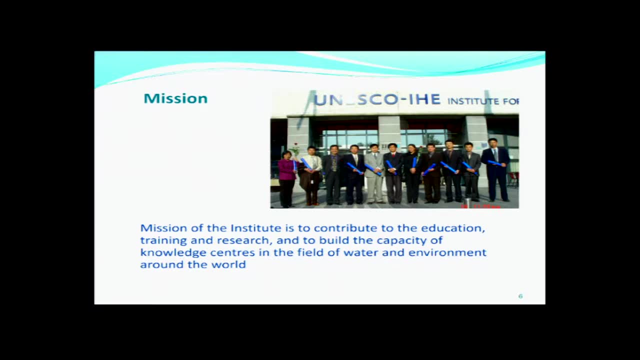 Again. Maria Clara would give PhD defense on Friday, So all come, you will know more how to collect data about environment. Dutch know how to do it. So our mission in the institute is to contribute to education, training and research. 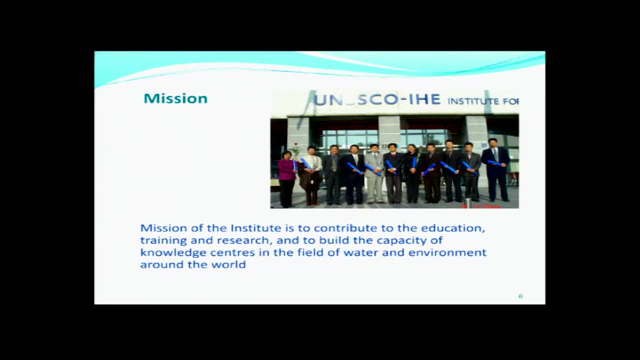 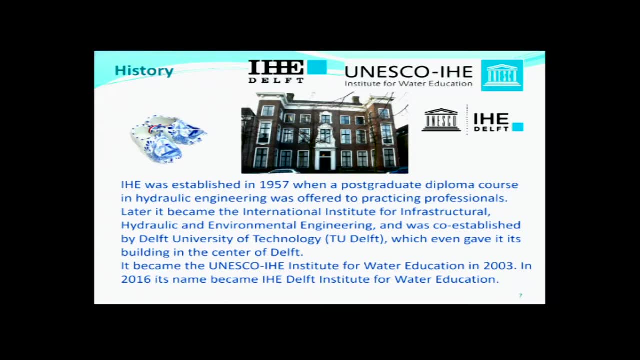 And build capacity of different knowledge centers around the world. Okay, We were established in 1957. You can read history, I will not go into it. But Delft University of Technology has played some role, But mainly Dutch government who reacted to the request of ambassador of East Pakistan at that moment, Bangladesh now. 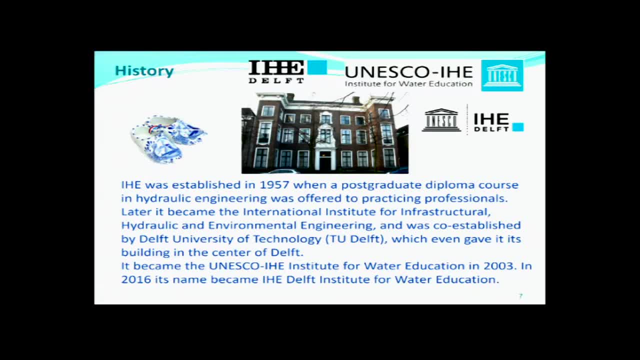 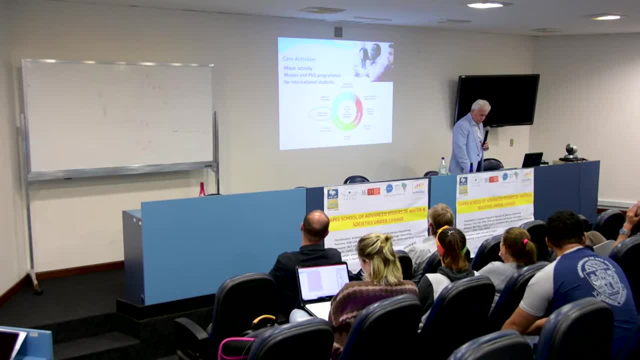 When there were catastrophic flood, they asked help from Dutch engineers to train their engineers, And this is what was happening, And since then we grew quite considerably And we are now postgraduate institute, So our main activity is master program. It's last 18 months. 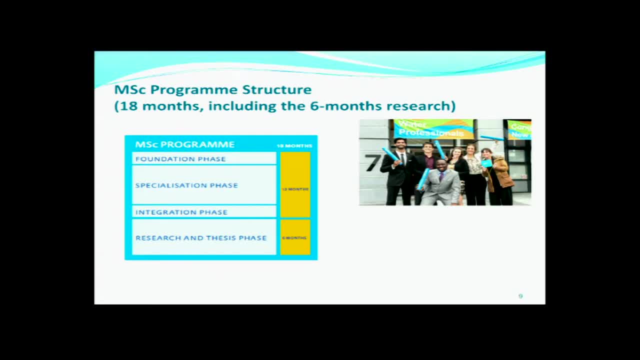 There would be new options for 12 months and 24 months, But currently it's 18 months. So we have specialization, We have the training phase and master research and thesis part. This is most interesting part, Of course. this is where people show their creativity. 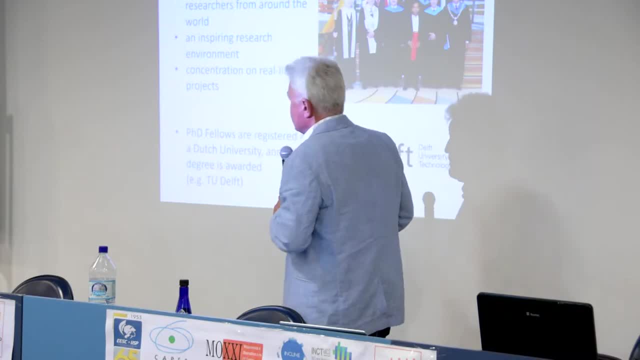 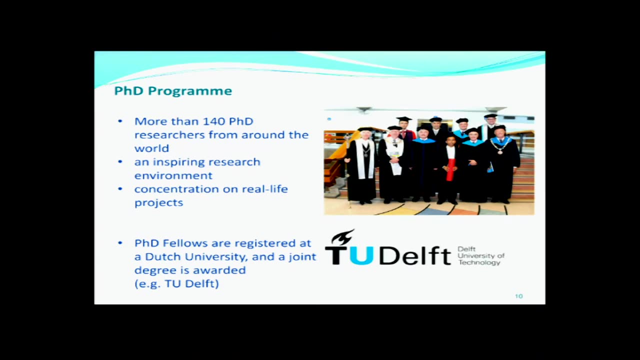 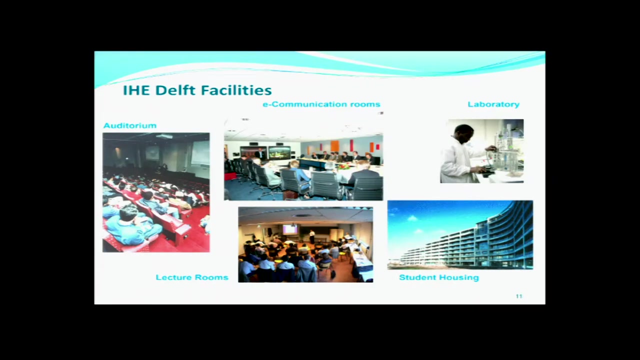 We run also PhD program. We cannot award degrees by law In the Netherlands, only universities can award degrees. So we work together with Delft University of Technology And we award PhD degrees. We have quite wonderful facilities, So students feel quite happy. 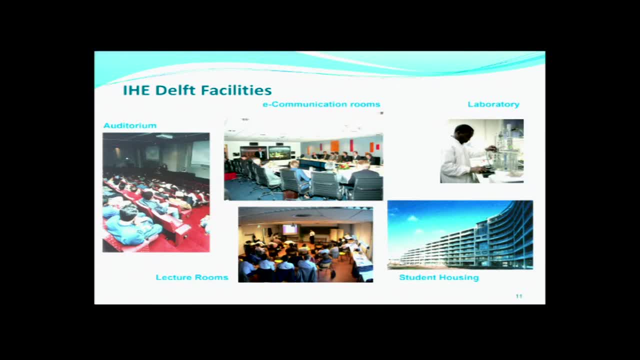 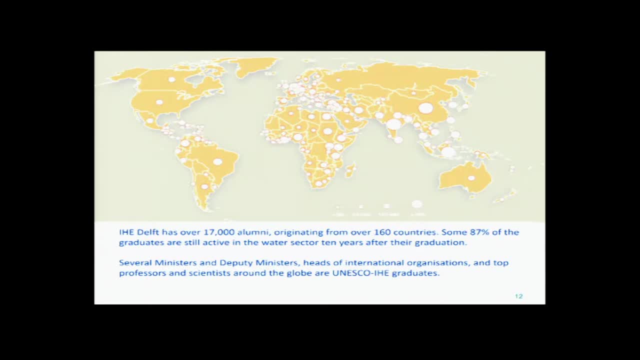 Hostel, where they have separate rooms for each 20 square meters. So it's reasonable. Now we have 70,000 alumni around the world from Brazil. You see quite a big circle here. So quite many people were trained from Brazil as well in our institute. 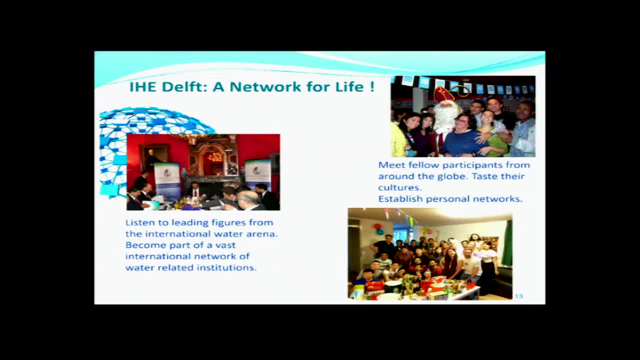 And what is most important maybe is network for life: Not only knowledge, but also connections, acquaintances, new experiences that you come from. Don't drink. That's Campirinhas here. Maria Clara is somewhere here. Have you been to this party? Hydroinformatics party. 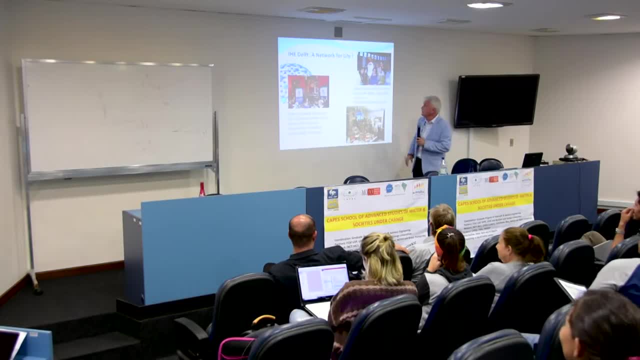 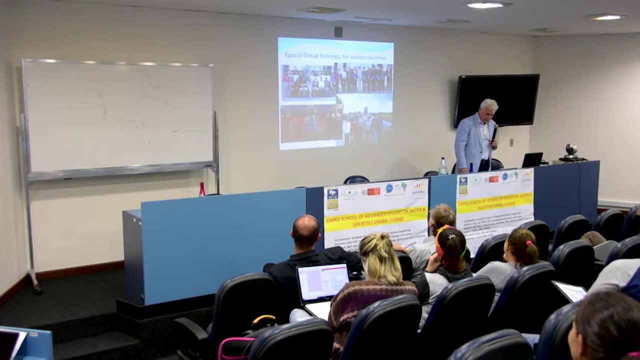 No, No, no, You were studying hard, I know, So you were not there Anyway. so people learn each other and it's friendship for life. Really, that's one of the most important components of this. We also organize special group training, short course and so on. 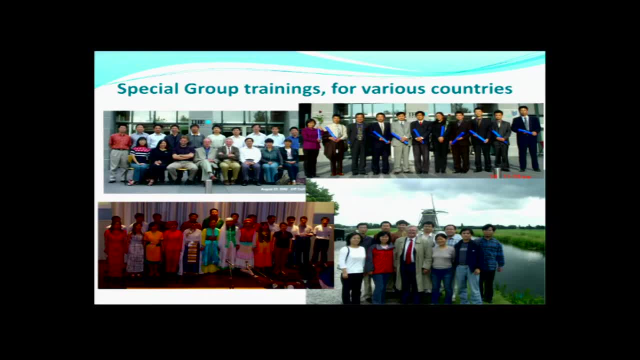 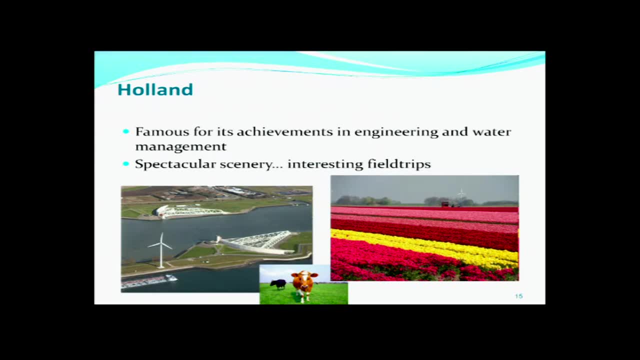 So you're welcome to apply. We have 70 short courses, also online courses, special group training and so on, So you're very welcome to apply. Okay, Holland, Nice place, Come to visit. Tulips, water cows, bicycles, high-speed trains. 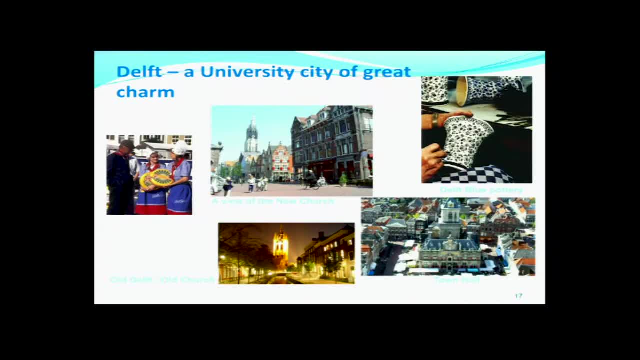 Paris is three hours from Delft. Delft, really nice city, like your city, actually Very large technical university and IHE, of course, Many students, A lot of cheese, beer, nice people and nice architecture. And Delft Blau if you want to buy. 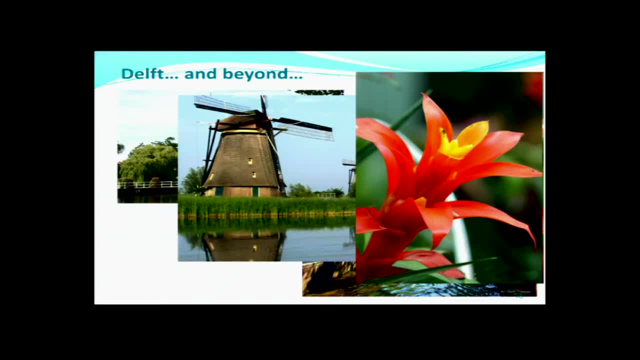 So that's about our institute in general- A bit of appetizer. So now let me switch to a bit more technical presentation about any questions. Any questions about IHE? No, Okay, Come to Delft, I'll tell you more. 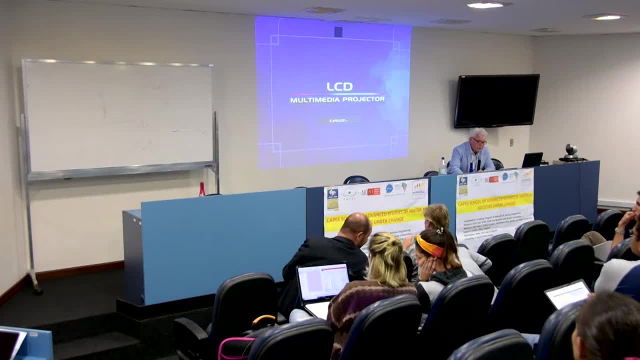 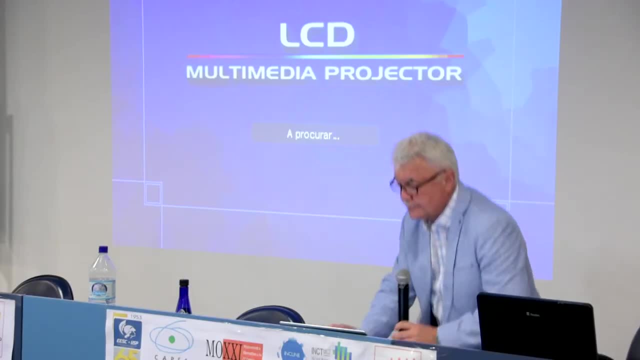 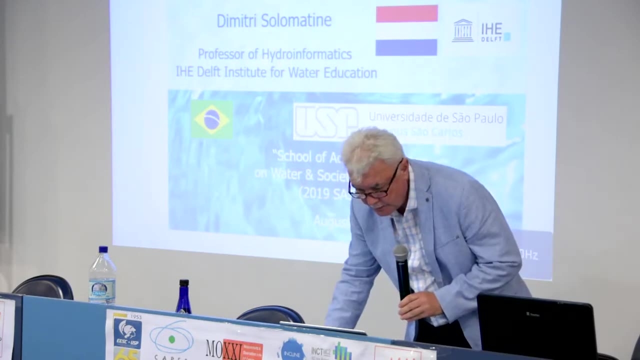 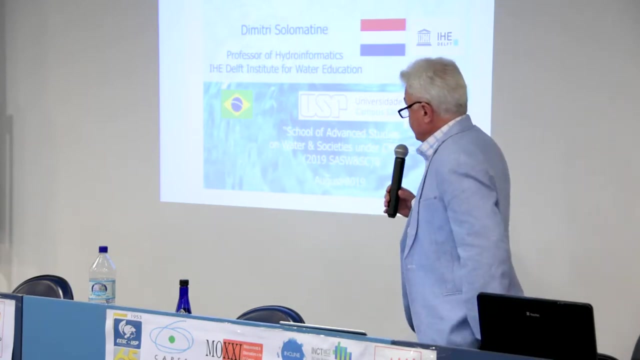 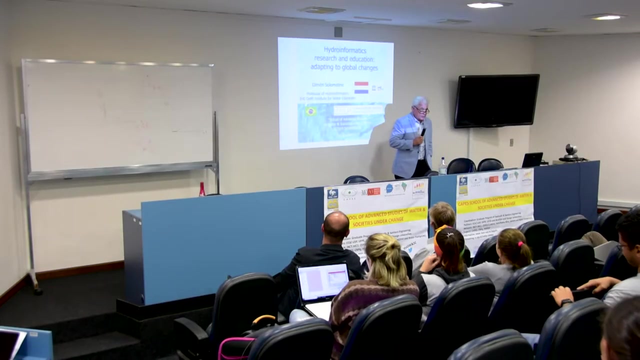 All right, So let me close this one And we'll switch now to this. So I'll talk a bit more about education and research. And everybody says climate change, global change, So I was asked also to put in perspective. 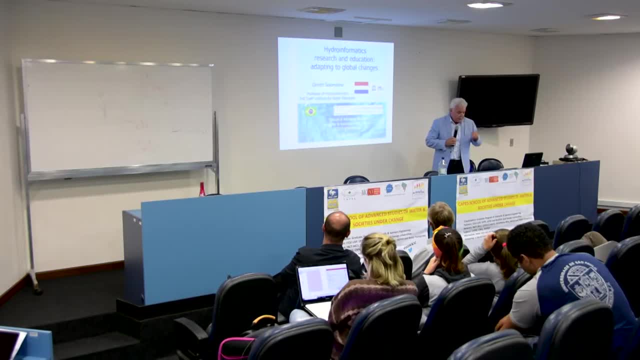 And indeed we have a lot of global changes happening And it's important that we have also appropriate tools to react to these changes and to forecast the impact on society. So hydro-informatics started in Delft, in IHE Delft actually. 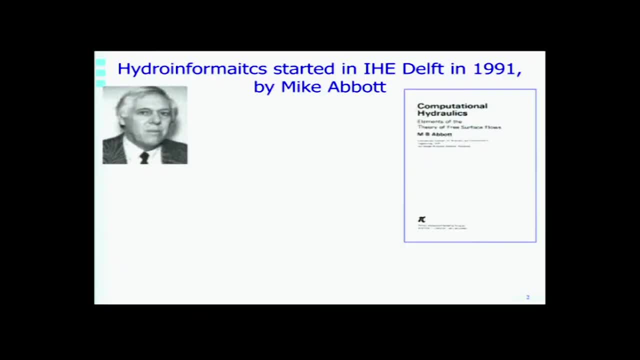 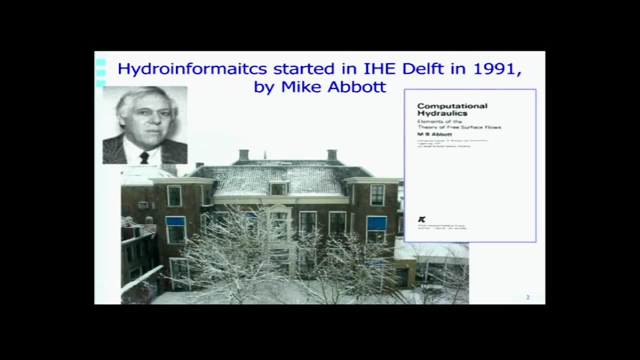 That's where Michael Abbott, professor of computational hydraulics at that time, He coined this term. This is our building in winter And he is an author of quite widely spread book, Computational Hydraulics, published in 70s, 90s and so on. 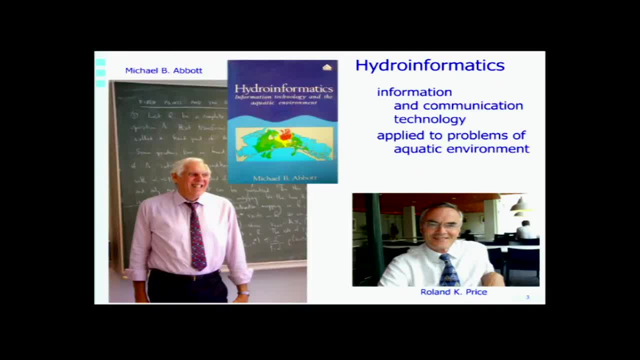 And at that time he decided that information technology is the right way to look at things And he connected hydro, water and information technology together. So we define hydro-informatics as information communication technology applied to problems of aquatic environment. Quite general thing. 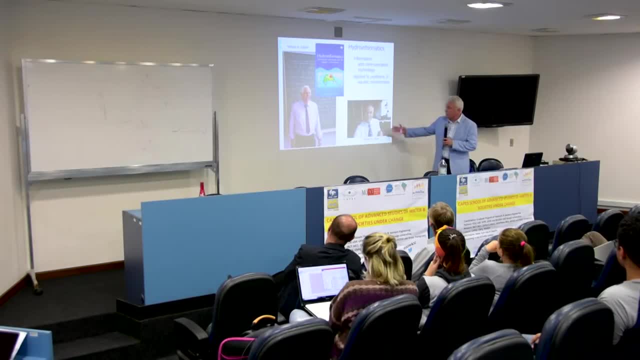 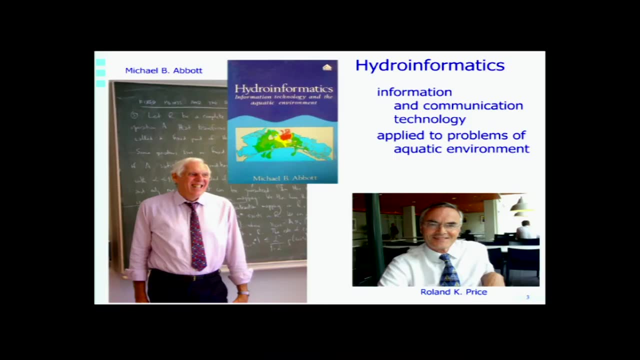 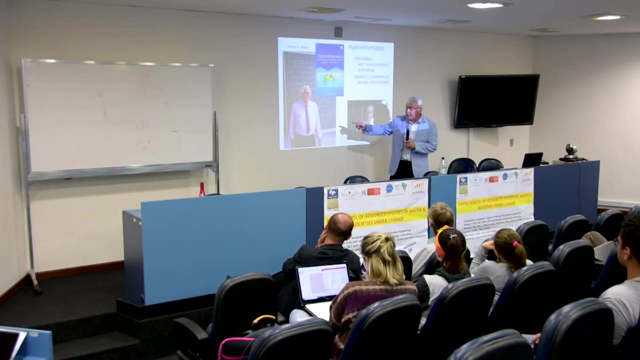 But I will give you a bit more details in a second. So Roland Price replaced him when Mike retired in 1997.. He, by the way, was also organizer of the computing center of Danish Hydraulic Institute. It was him Mike 11,, Mike 21,, and so on. software is because of him, Mike. 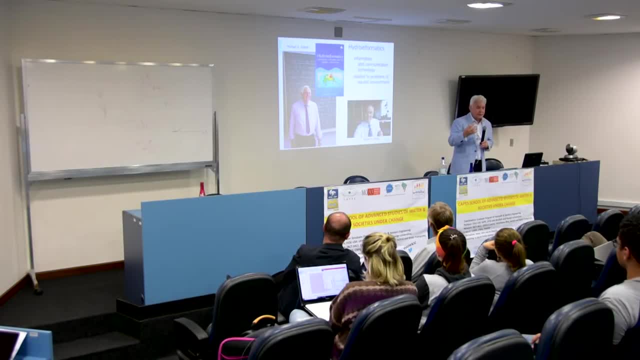 So he is actually, was and still is a visionary who understand what will society look like in 15,, 20 years from now, and not in the future. So he is not talking about now, He is always talking about the future. So that's what many people learned a lot from him in this area. 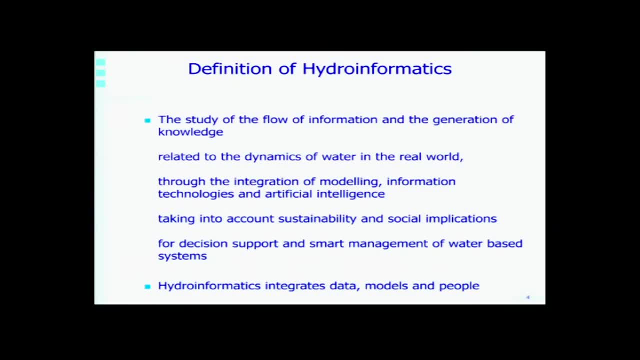 So, if we define hydro-informatics in a bit more detail, we look at the study of the flow of information and the generation of knowledge related to dynamics of water in the real world, And then technologies, through integration of different technologies, modeling information. 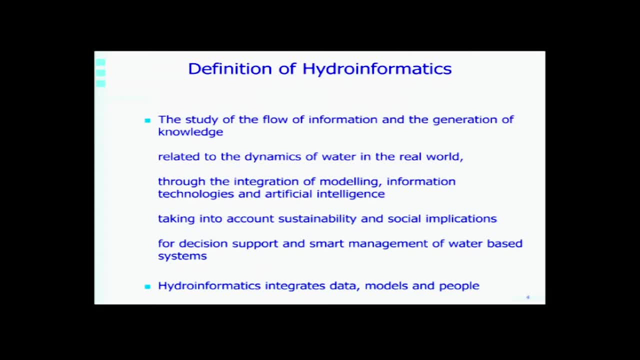 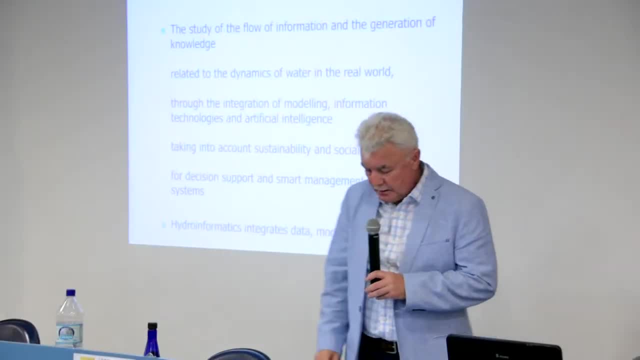 technologies, computer science and artificial intelligence, And we take into account sustainability and social implications, and all for smart management, decision making, for water-based systems. So we try to integrate data, models and people. So we also look at the social component as well. 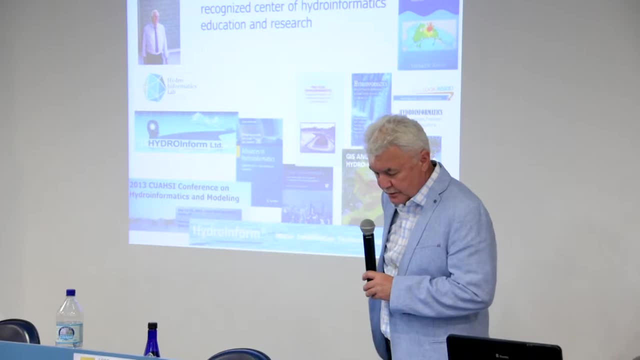 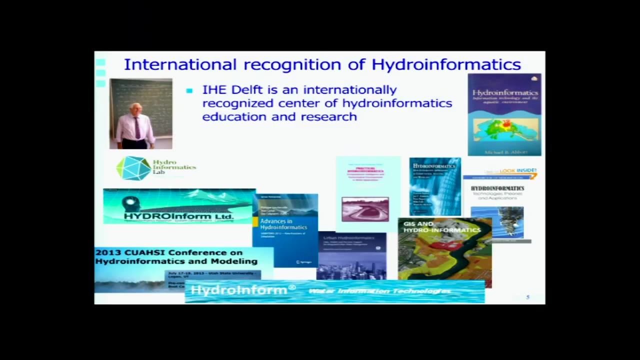 Okay, We could talk about different books published and the special issues of the journals. conferences organized- Some companies have the name hydro-informatics in them or hydro-inform- which were organized by our graduates from IHU. We are proud of this. 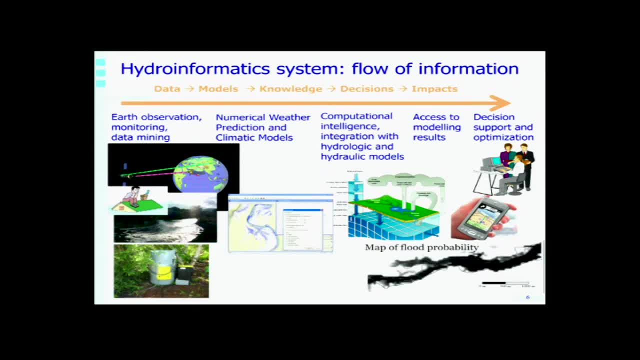 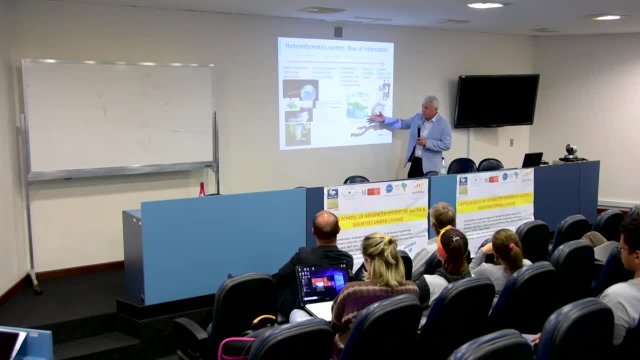 So we look at the world holistically, and at technologies as well. So technologies span from data collection analysis to different types of models being linked, integrated into chain of modeling systems and then leading to better decisions made about water systems, for example, to predict floods or to find out what pipes are. 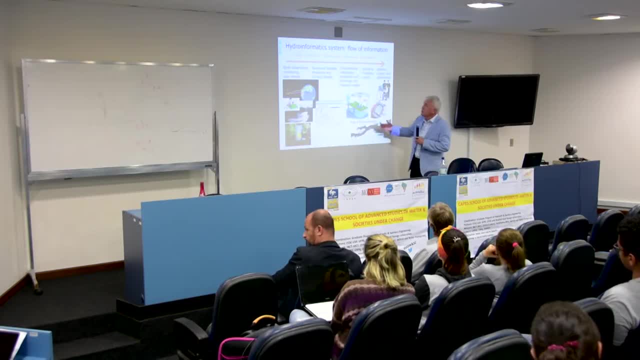 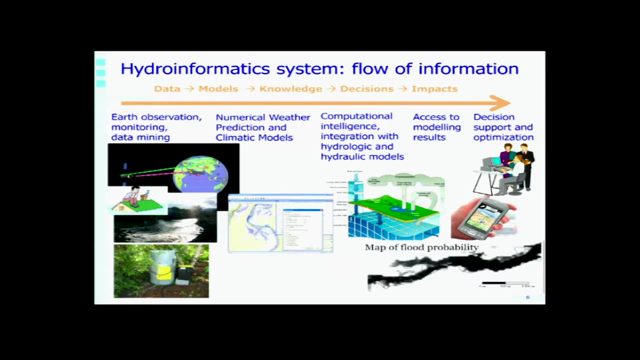 leaking in urban systems, and so on and so on. So we look at data models, knowledge, because we think models generate knowledge. Okay, So not data, but knowledge, because models encapsulate a lot of knowledge and then into decisions and impact. 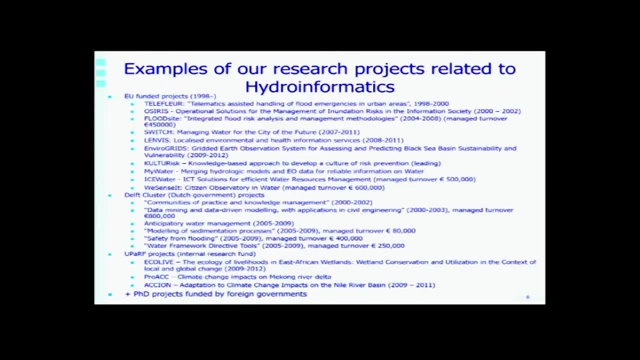 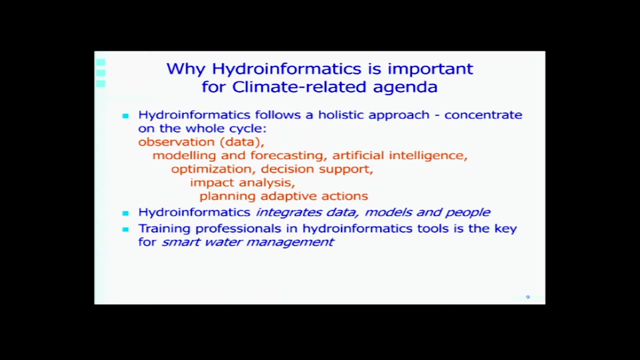 So that's the approach we take. in hydro-informatics Okay Books we talked about this, Some examples of our research projects, but the font is so small you cannot read it, so I go to the next slide. So why hydro-informatics is important, also for climate-related agenda. 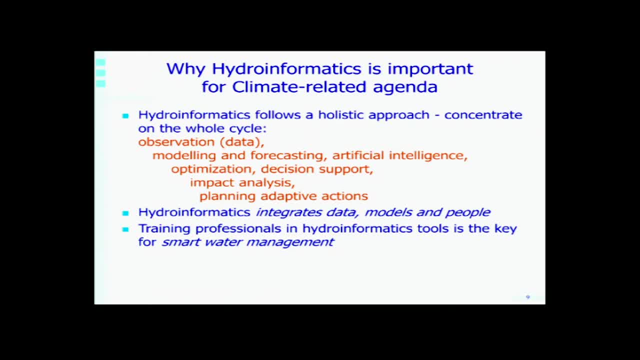 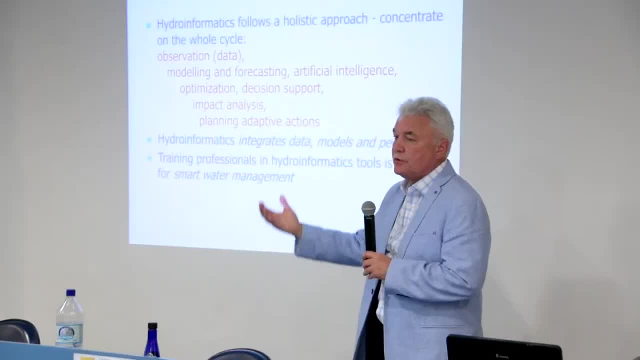 We follow the holistic approach, as I explained. So, using all this technology- And since we use modern technologies, we could better understand the data that we observe in the real world first, and second, to forecast the future state of the world. So that's what we think how most technologies should look like at this holistic approach. 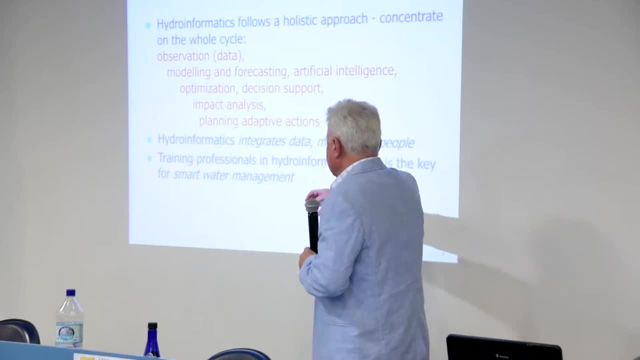 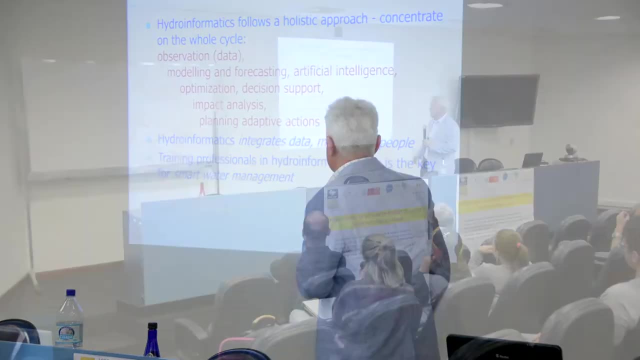 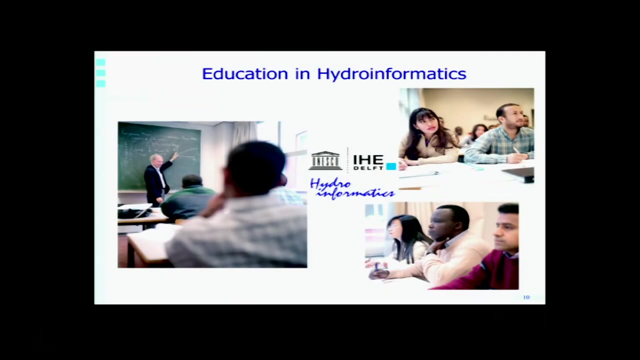 not only in water, in all other fields- to integrate different things into sort of chain of data collection, modeling, decision-making and optimization. That's what we try to do Now. since we're educational institute, we do half at least of our work is in education. 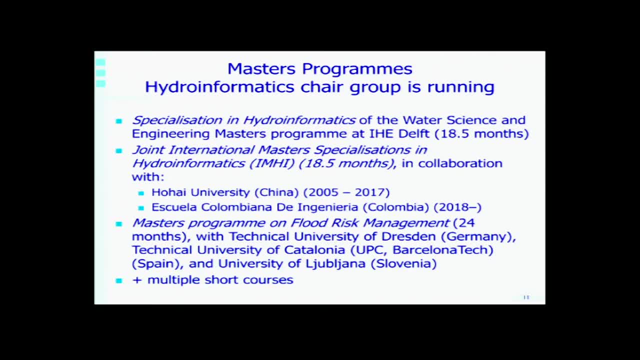 So we in hydro-informatics we run two master, maybe more master programs. So main part of it is indeed specialization of hydro-informatics and part of water science and engineering program, which runs 18 and a half months. 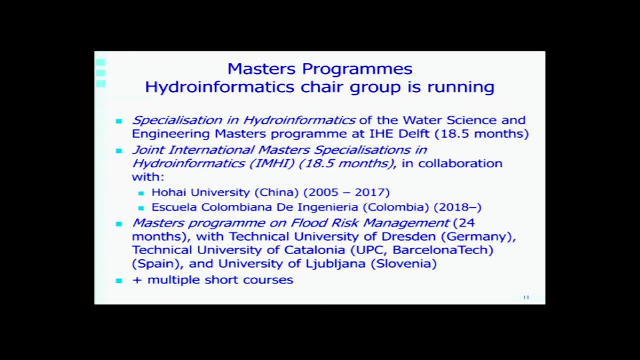 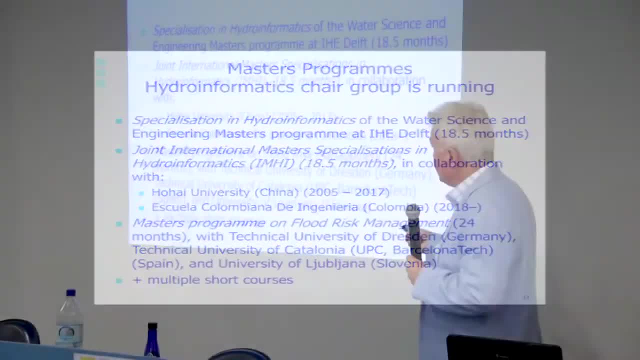 So that's our main focus, That's our main product, so to say. Then we also have versions of this program which are in collaboration with Hohai University in China and the School of Columbia and Engineering in Columbia. So this program has just started. 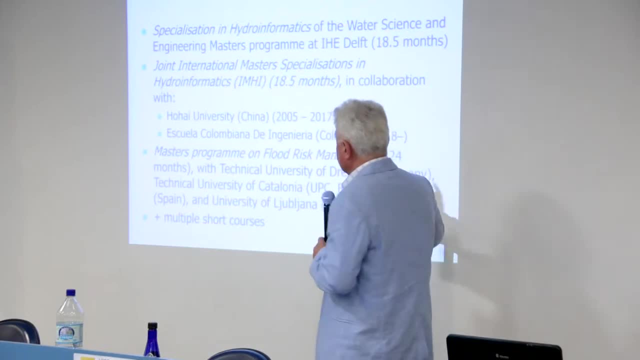 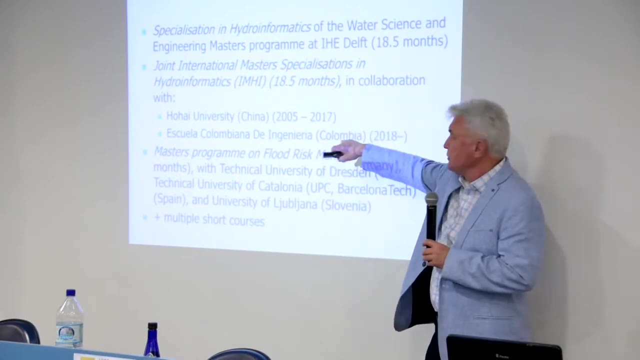 First people registered And, by the way, I forgot to tell you earlier, if you're interested, check their website and maybe you would like to come to IHE through them. So because you would start then first, several months in Bogota. 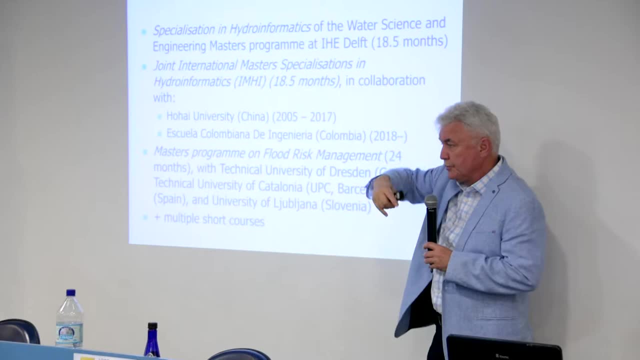 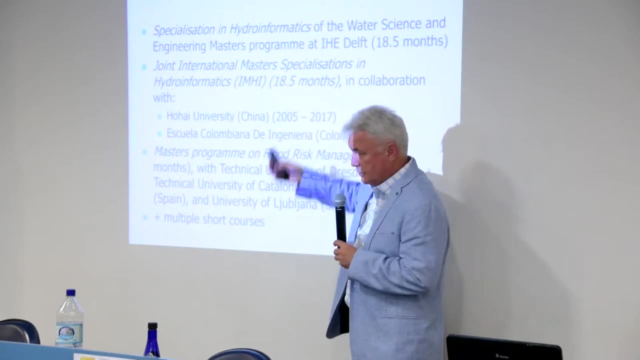 And then this study is in English, And then you come to Delft. So that's what we agreed with them to develop. And for the Colombian students, they have also the funding from and, But in Brazil I think you have similar arrangements. 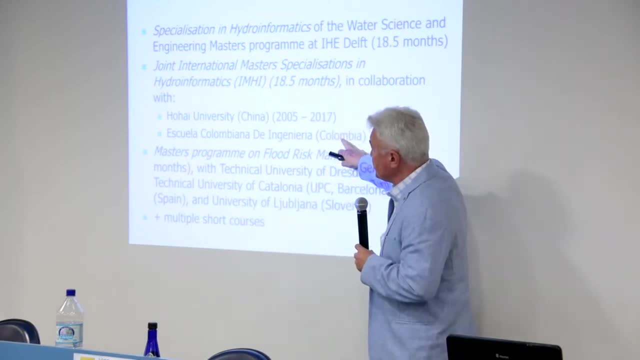 So perhaps it's we're thinking of establishing similar programs for Latin American market, maybe with other universities, maybe with your university. It's not easy to do because of bureaucratic reasons, But okay, we hope it will run. And then another program, master program in flood risk management. 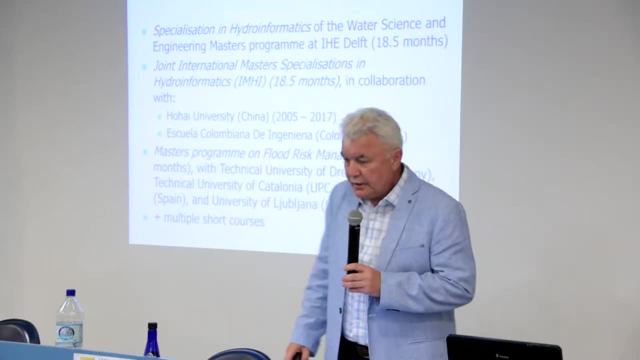 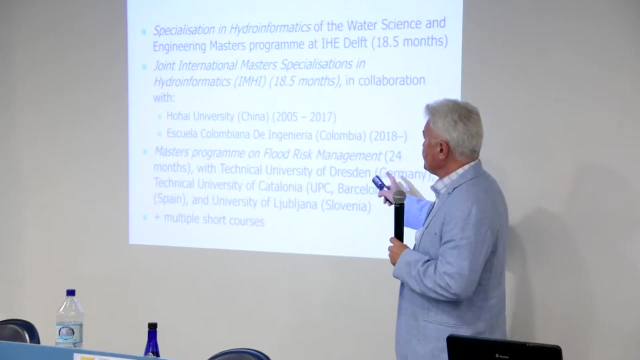 which is funded by European Commission. So every year we have approximately 20, 22 students starting this program And it runs for two years. Start in Dresden for six months, Then six months in Delft, Then three months in Barcelona in Spain. 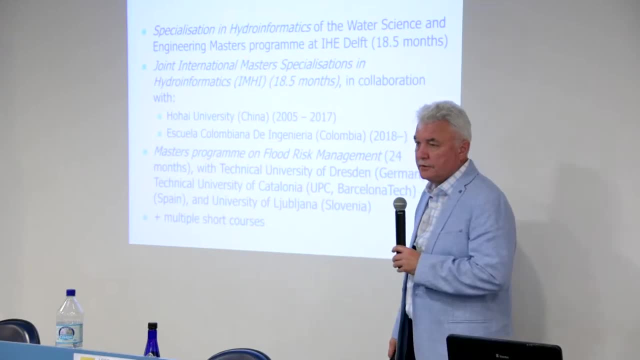 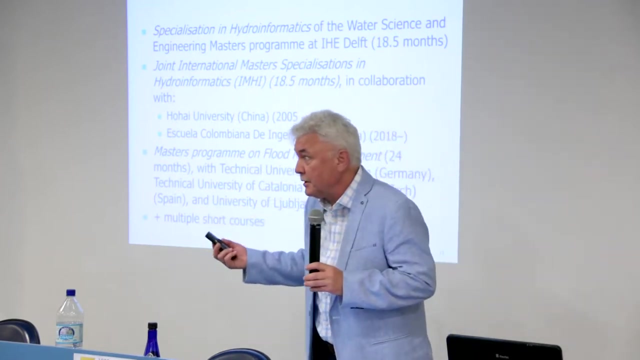 And two months in Ljubljana, in Slovenia. So then after that we have six months MSC, which is done in either of these universities or with industrial partners in Denmark, UK, Brazil maybe. So we think of this. 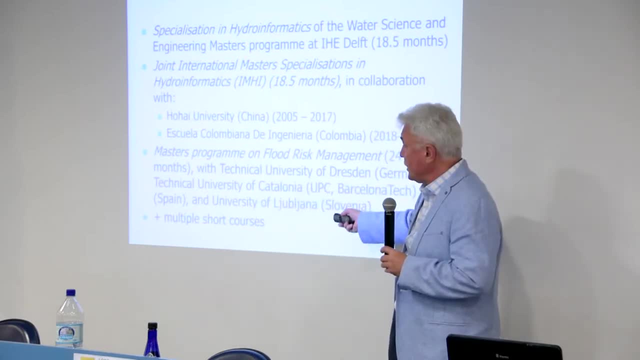 So please, flyers are here. Everybody is welcome to apply. Why? Because we have fellowships. It's expensive program to pay from your own pocket. But if you're a good student, lucky and write a good motivation letter, we'll consider. 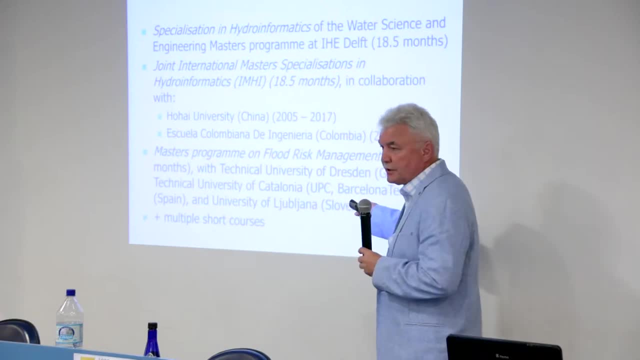 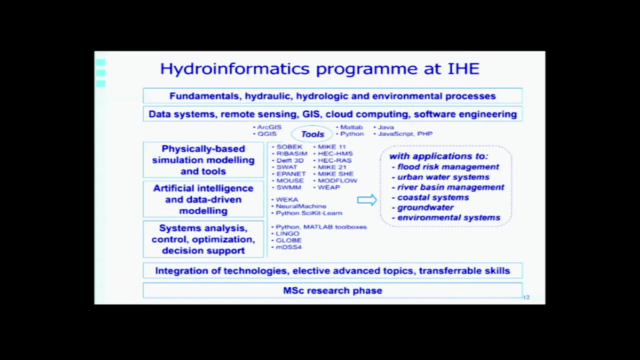 Again, it's a very competitive program. We have 400 applications every year And we give. We give 10 or 15 places for countries, non-European countries. The rest should be Europeans. Welcome to apply Now. hydroinformatics: 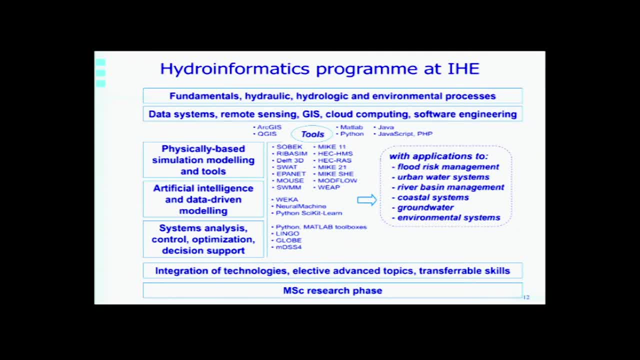 We talked about this already, So in our program we start with fundamentals, Always: hydrology, hydraulics, environmental processes, But also data systems, remote sensing, GIS, cloud computing, software engineering. So these are some basics we do in the first half year. 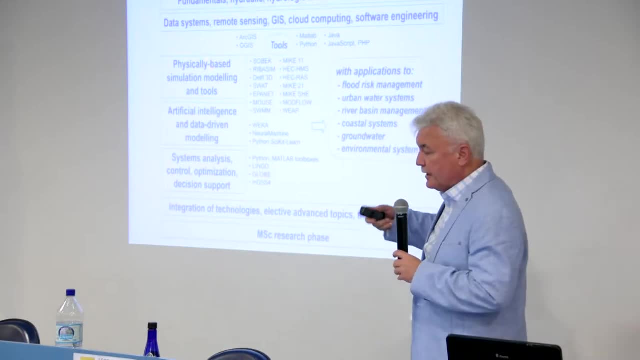 And then we move to modeling tools. So we think modern engineer and manager should be able to use tools because they encapsulate so much knowledge in them. And then we train people in physically-based simulation modeling. So these are list of different modeling tools we use in engineering. 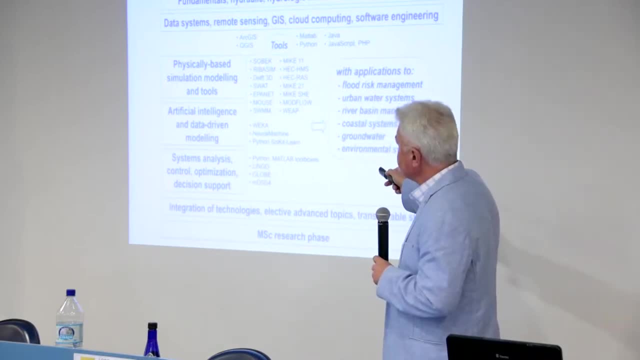 So Sobek from the Deltares, Delf Hydraulics and so on- Sorry, the Danish Hydraulic Institute- and so on. And then artificial intelligence and data-driven modeling. So I was happy to see on the previous slide all these words. 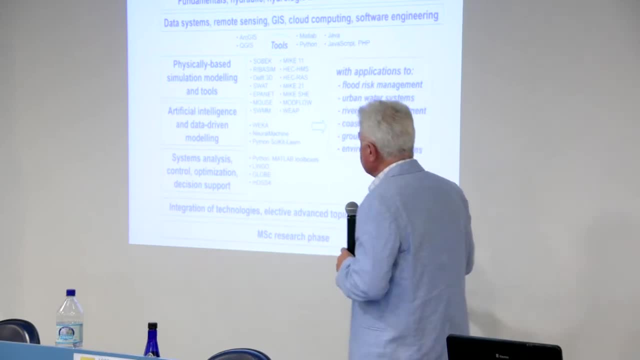 We will be, by the way. you will hear some lectures, some of them at least. So we use Veica, Neural Machine, Python, SkyLearn and so on, And systems analysis, control, optimization, decision support. These are three blocks. 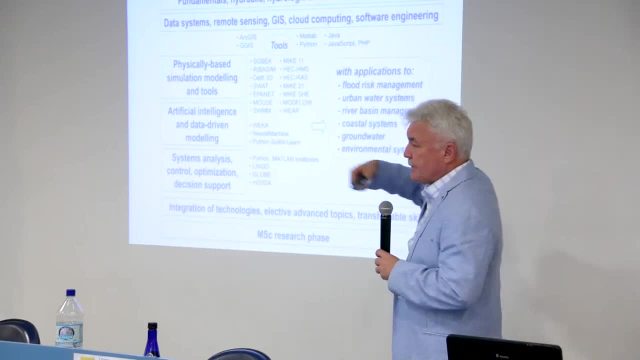 And these are application areas And, as you see, it practically covers all water-related areas. It doesn't mean we do everything deep, deep, very much, because we don't have time, But we concentrate a lot on floods, And urban systems also have specialized modules. 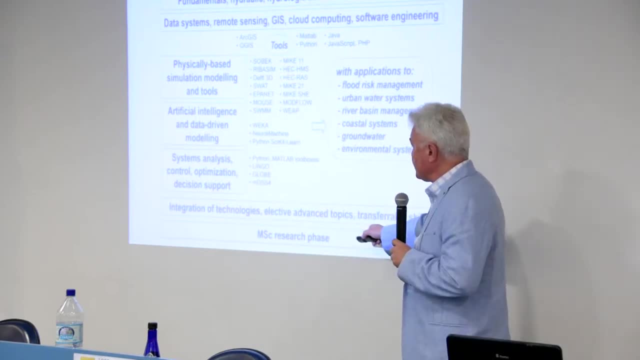 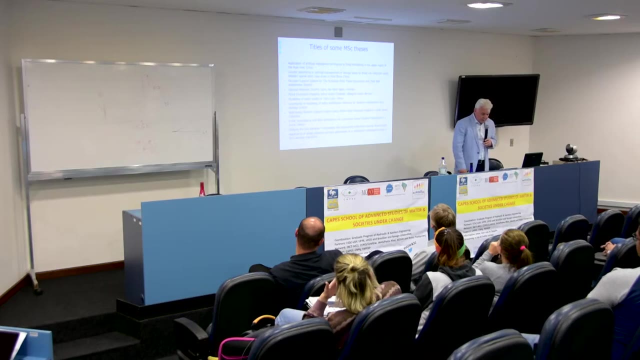 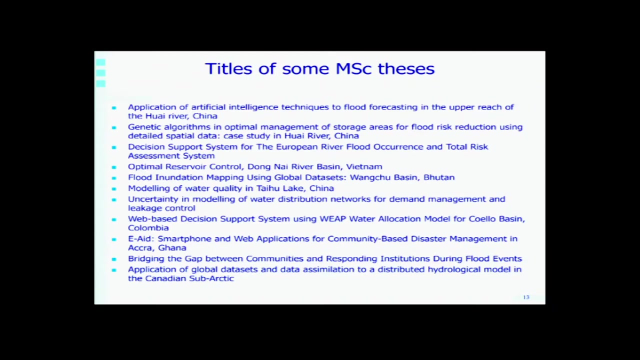 And then we have topics on integration And then last six months MSC research phase. So that's our program of 18 months. Some titles of the MSC thesis- Look, I cannot read it all, But we apply artificial intelligence techniques for flood forecasting in Huaihe River in China. 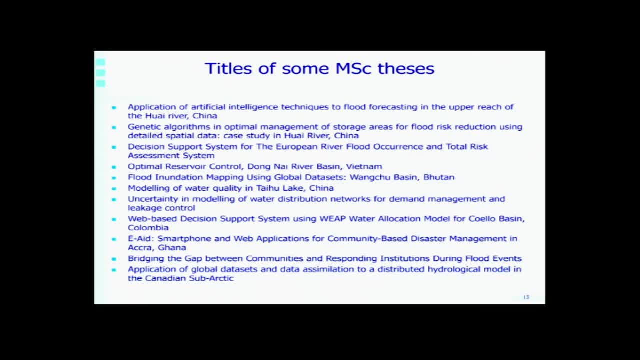 Genetic algorithms, again for management storage areas for flood risk reduction. I'll talk about that. I'll talk about this case in a second Decision. support system for European river flood occurrence and total risk assessment system. Optimal reservoir control in Vietnam. 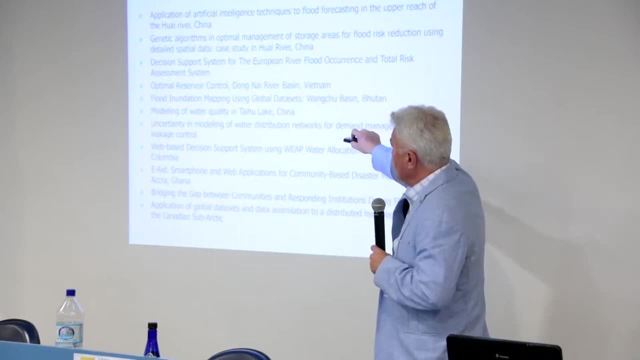 Flood inundation mapping in Bhutan, Modeling of water quality in Taihu Lake in China, Web-based decision support system in Colombia, Smartphone and web applications for community-based disaster management in Ghana, And so on, and so on, and so on. 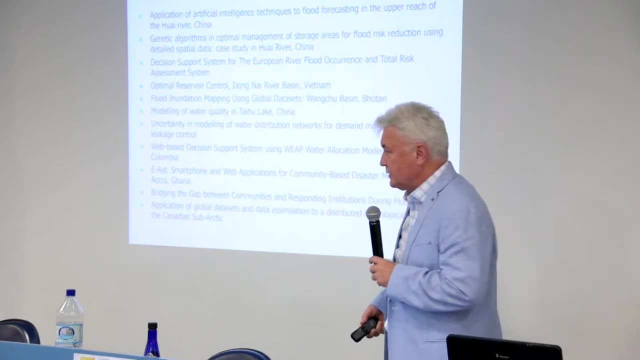 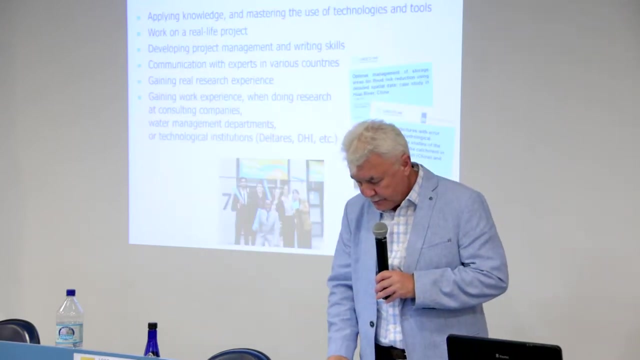 You can read our website, You will find very interesting titles And many MSC thesis are available online And, by the way, all our PhD thesis are available online through repositorytudelftnl. So all PhD thesis for free you can download from Delft University website. 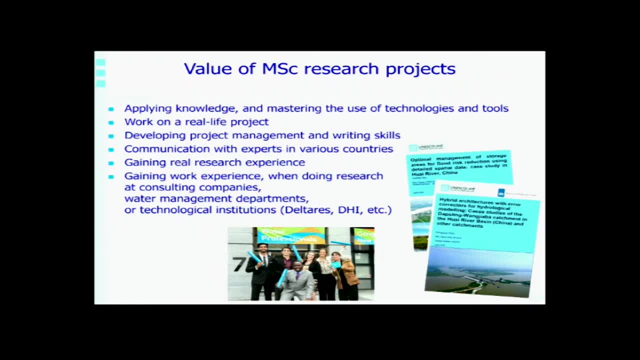 What is the value of this MSC research? We think is applying knowledge and mastering use of technologies and tool. Work on real-life project, Because most of our MSC studies are not theories but very much practical. Developing project management and writing skills. Communication with experts in various countries. 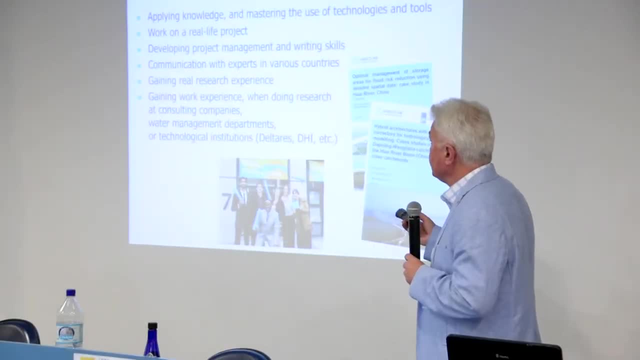 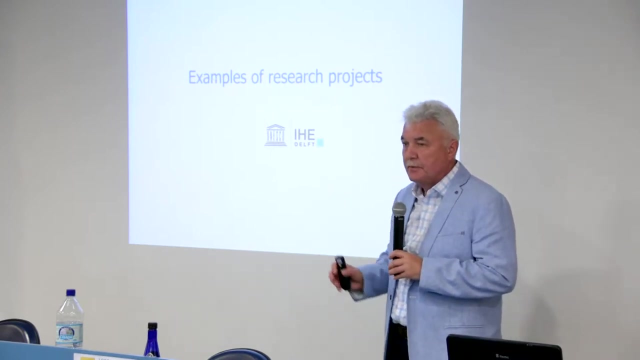 If you go to do MSC elsewhere, but also in Delft, Gaining real research experience, work experience And working with important technological institutions, with their staff. That's really great experience. Now let me spend some time On giving you some flavor of what kind of research projects we did. 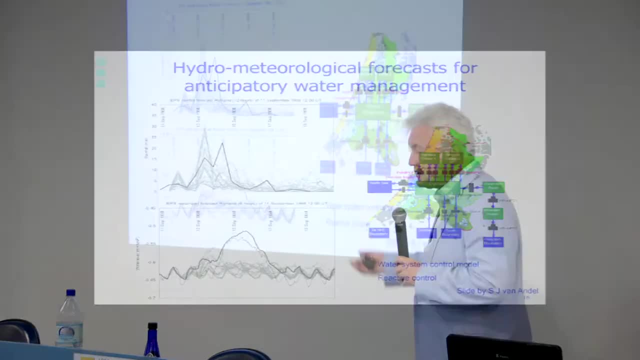 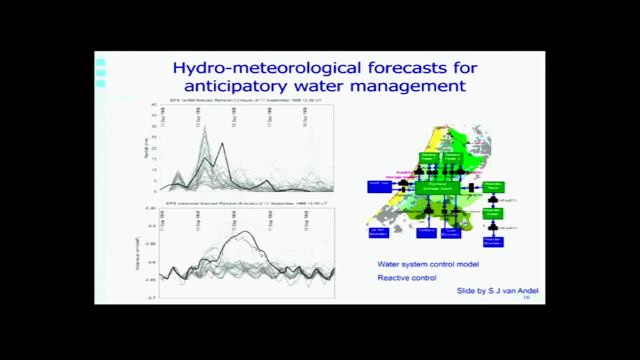 Look, we had in master and PhD studies, dozens And also research project for European Union, Dutch funding and so on, Different projects. So this choice is maybe not optimal, But it will give you a flavor. One thing: This is Delftland. 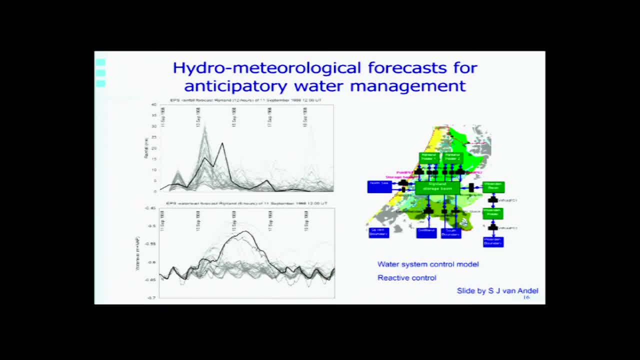 It's an area where water is managed. Delft is somewhere here. Sorry, it's Rhineland. I'm sorry, Delft is here, It's Rhineland system. It's north of Delftland, But it's here. 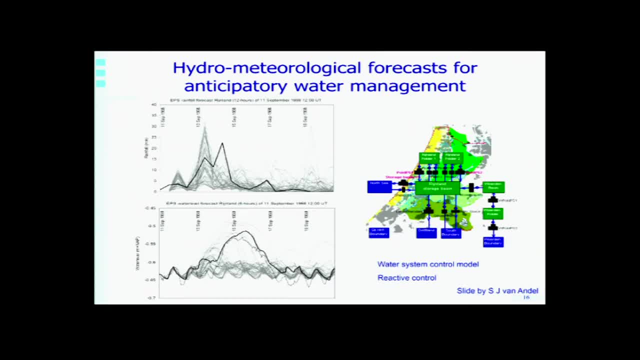 But it's very similar. So problem here is to pump out water. This is lowland, This is the ocean. Okay, Delft is here, Rotterdam is somewhere here, So this is lowland. Water is pumped out from this land by huge pumping stations. 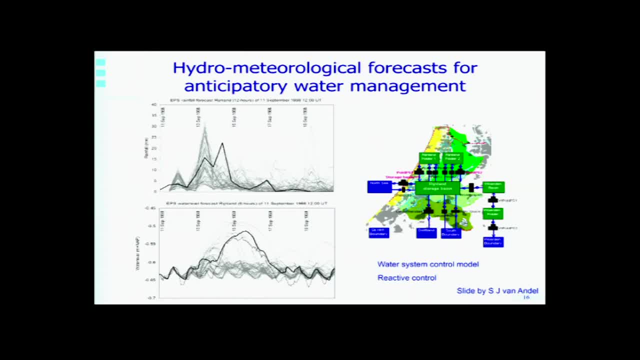 Which are here located Into the sea or into the rivers over here, So to keep water level, water table, low enough, Still there could be a flood. When does it happen? It happens when your forecasts Ensemble forecasts of rainfall. 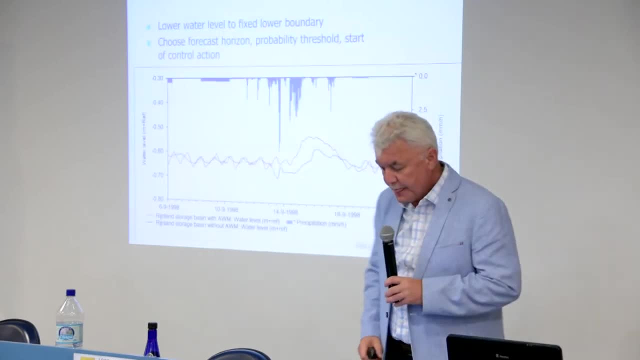 When rainfall is high, then water level goes up. So what we did? we developed anticipatory water management system Which is based on optimal control And what we can show that that's an example of the past. Blue line is water level. 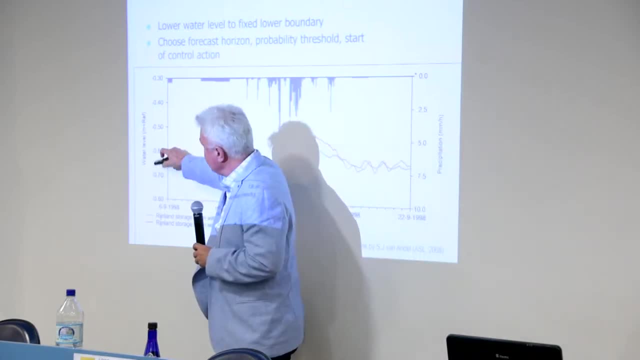 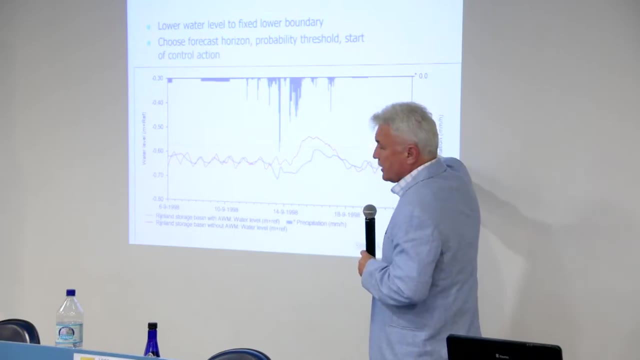 It's below sea level. You see, minus 60 centimeters below sea level. So water level on blue line was what really Sorry? red line was really happening And it exceeded alarm level, So it was flood Actually here. 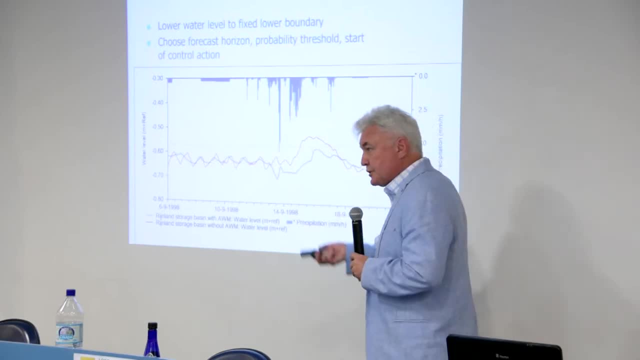 Control was suboptimal. When we introduced our system of optimal control, We can show that our system allows you not to reach alarm level, So it means flood will not happen And it costs not too much to switch from one to another. 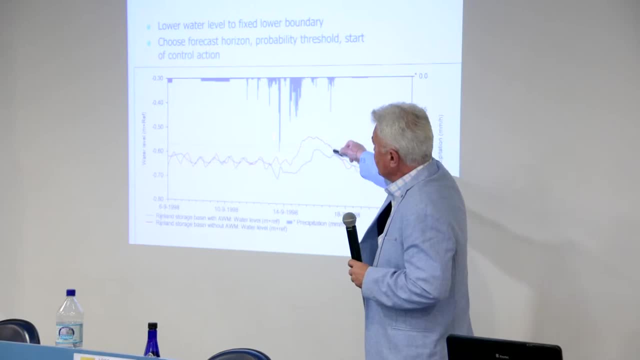 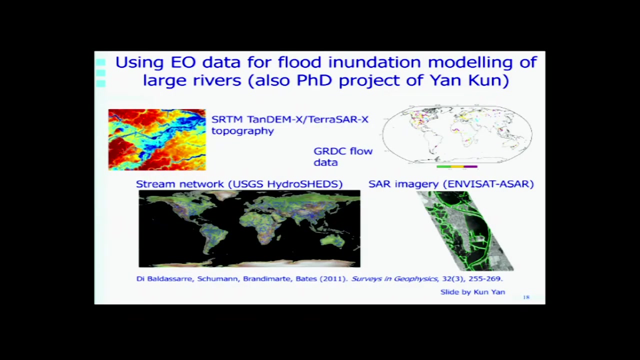 Simply why people were not doing this before It happened. of course, during this flood, rainstorm peaks, So that's what we tried. It's my colleague, Dr Salkian Fanandal, Who did this in his PhD. We also use a lot of Earth observation data to improve our modeling capacity. 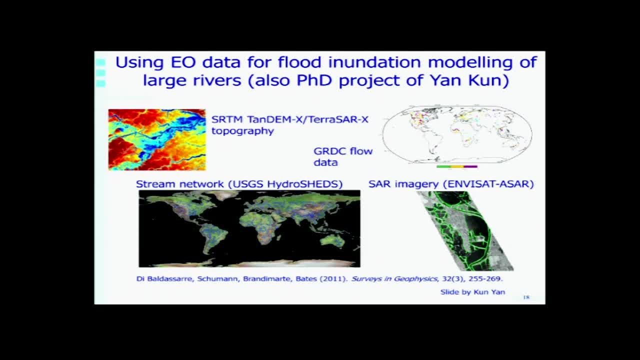 So our student from China, Kun Yan, Now he works for Deltares. actually We were proud. He was hydroinformatics students with PhD title. He was chosen one person from 90 applications from around the world for that position in Deltares. 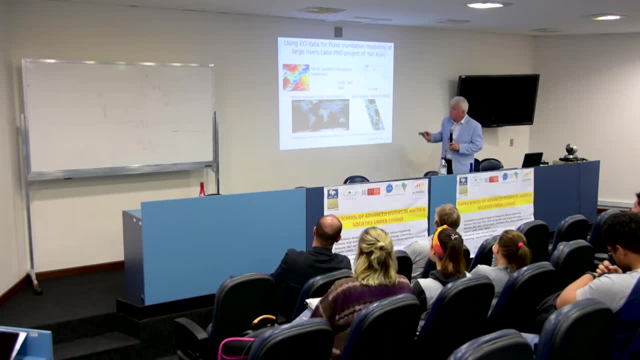 So we're really happy. So our student. So our students work now in Deltares, Several of them hydroinformatics. So we used, So we used freely available Earth observation data to improve flood inundation modeling of large rivers. 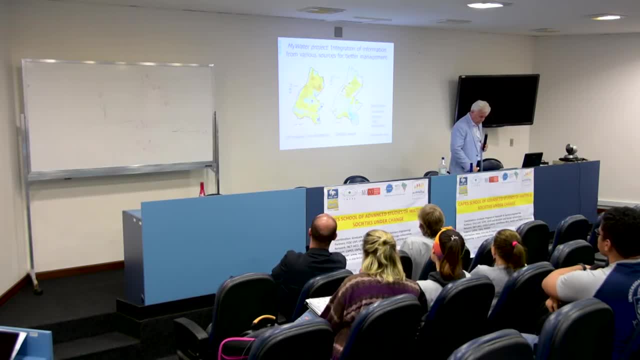 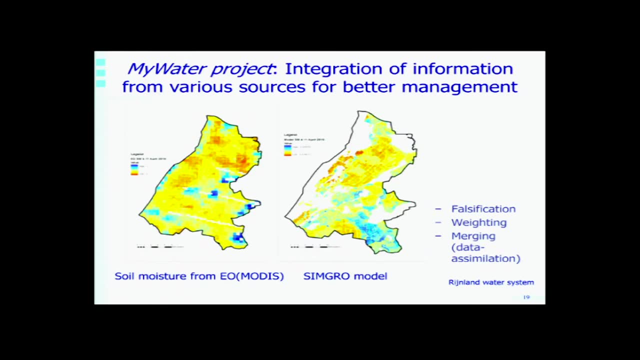 So it's one example. when we connect data to models In my water project, we try to integrate different information sources for better management. So what we did? We looked at soil moisture from different sources, Rainfall and so on- Satellite data. 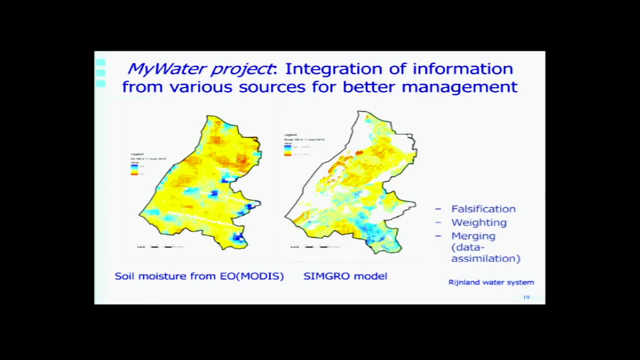 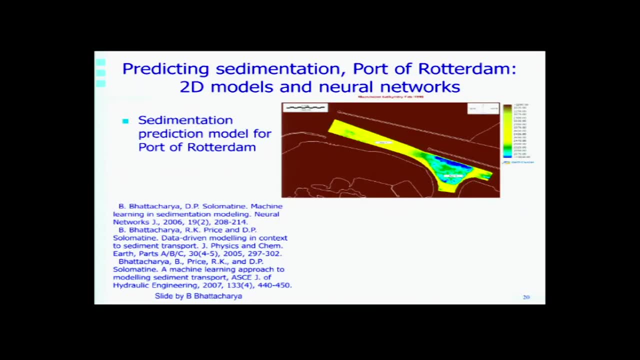 And it would be then integrated for better modeling tools. Yes, Thank you, See you later. Yes, Thank you very much. Now, another project which you may be not dealing with too much is using neural networks to predict sedimentation in Rotterdam Harbor. 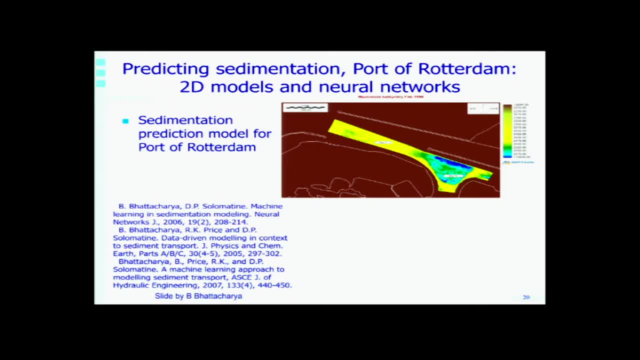 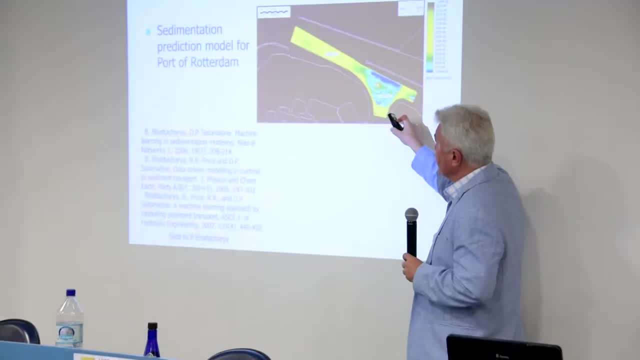 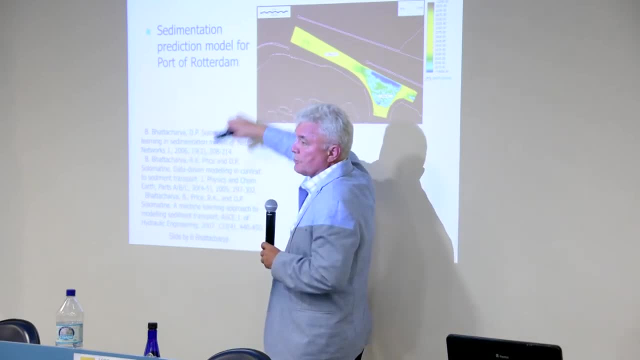 So this is Rotterdam, This is the ocean over here, And water ships come in over here through this entrance. So a lot of sediment happening here. Why? Because there's a dam somewhere here. Erosion of banks, lead sediment move 600 kilometers to the north with the currents and enters Rotterdam Harbor. 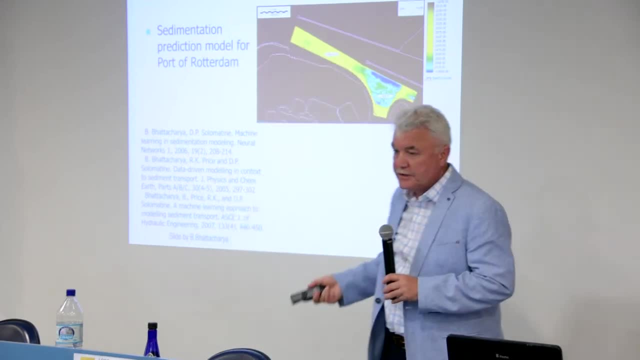 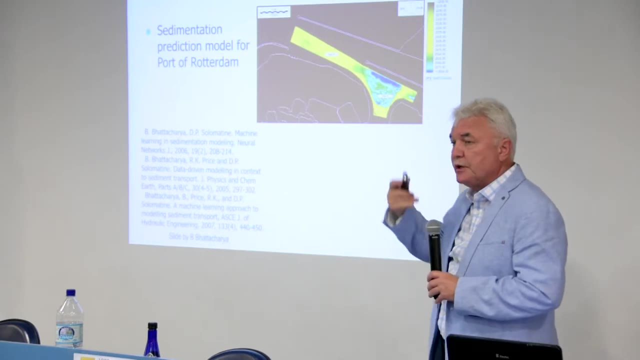 So that's a problem. So I have to dredge here How to predict sediment. We built neural network model, So it's data-driven model to predict sediment three weeks ahead So we can give better schedule for dredgers: when and what to dredge in this area. 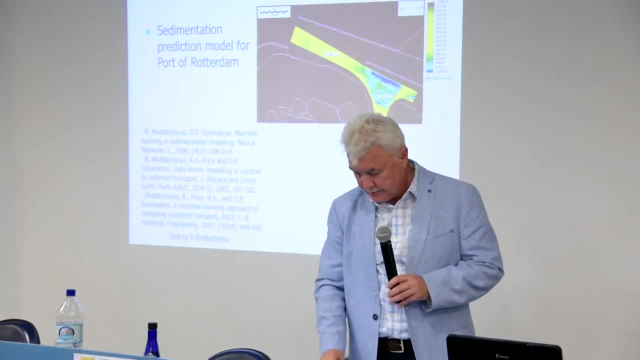 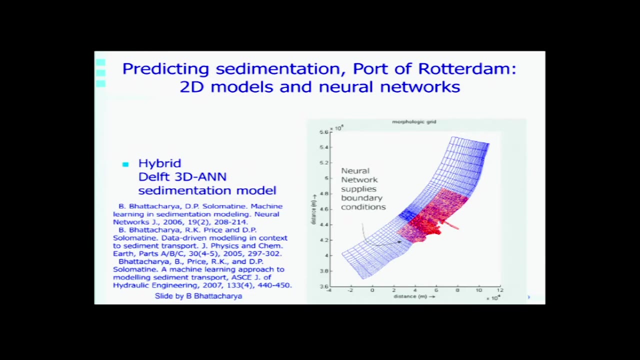 So that's one of the examples and it's published in different papers over here. Another example of linking physically based what we talked about already and neural networks model was to improve ocean modeling. So it's 2D model of sedimentation. port of Rotterdam. 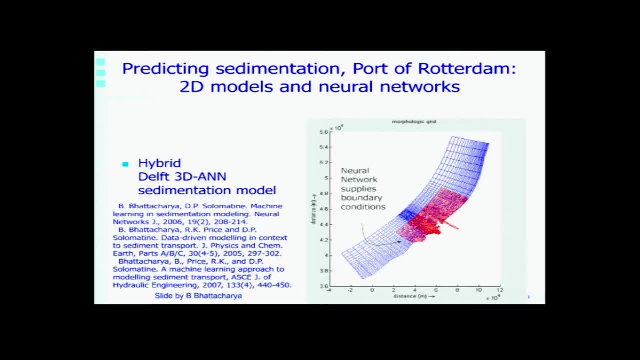 So it's another model. This is the hydrodynamic model of Deltares, built for the North Sea. So this is North Sea here. This is Netherlands coast. Okay, So this is rough grid, here coarse grid, And here you have refined grid. 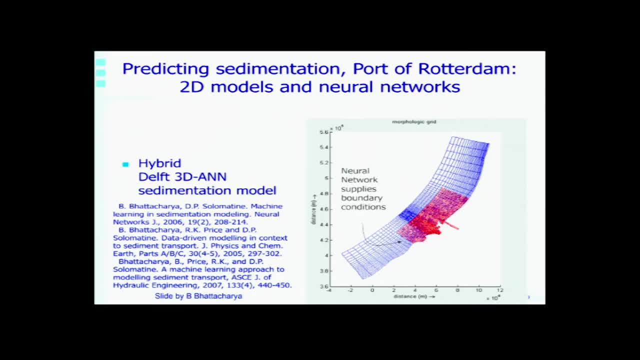 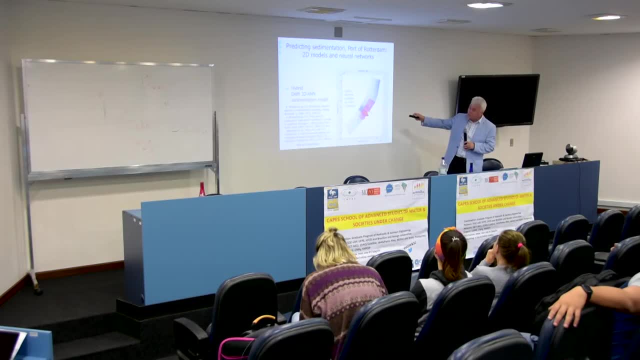 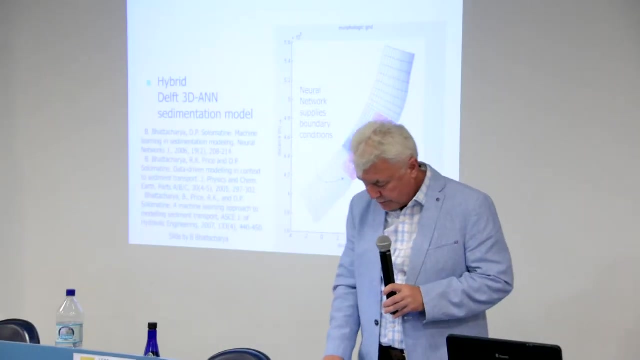 Problem is that you cannot run this block without getting data from here. So what we did? we trained neural network based on previous model runs to supply boundary conditions to this particular model. So it was typical hydrodynamic- sorry- approach of hybrid modeling when we linked hydrodynamic model of Deltares and our neural network. 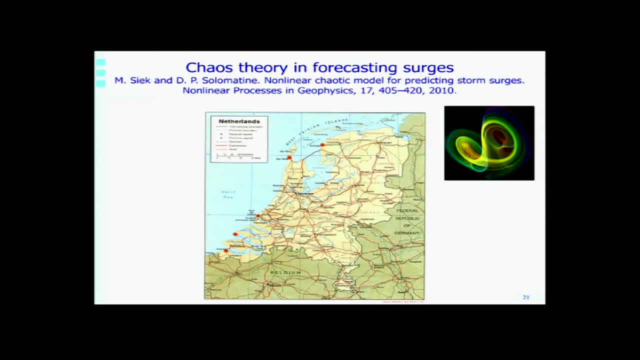 This interesting application of data-driven models, What we did here. so this is Delft over here, This is Rotterdam here, And this is largest port of the world which is located here. Now we want to predict ocean surge during bad weather. 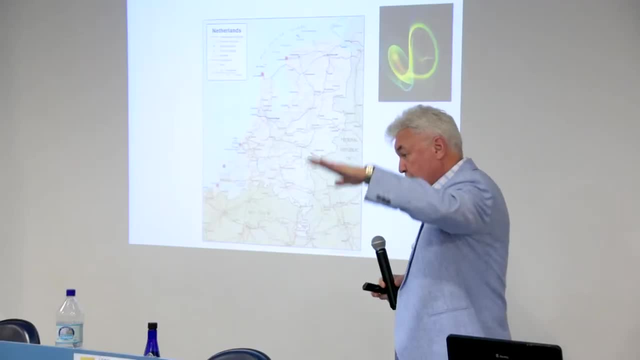 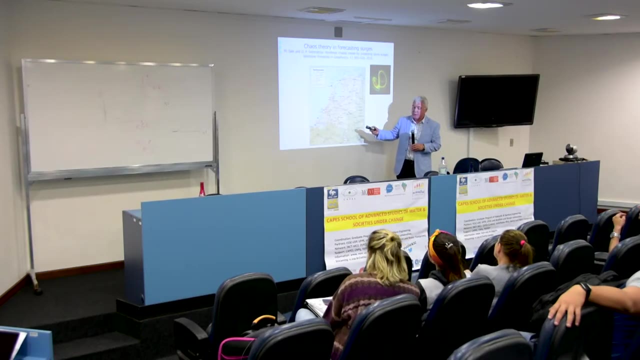 Ocean waters go up and down up to two meters difference. So the thing is that when boat ships come into the Rotterdam harbor, large boats have the draft of 20 meters and depth is 21. So they're close to hit the bottom at this point of entrance. 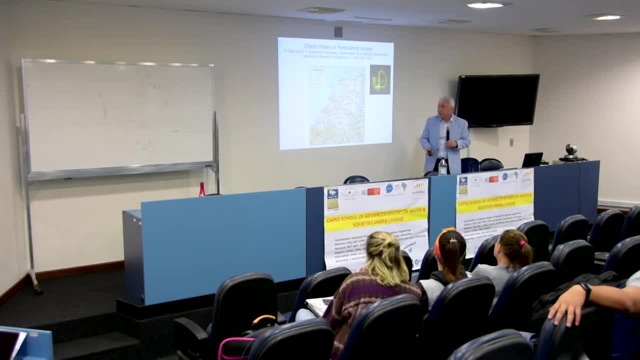 Ships are so big. Why they're building such a big ships, I don't know, But anyway it's at the edge. If they would be 20 meters tall the ships, they could not enter Rotterdam. So if surge is low then the ships cannot enter. 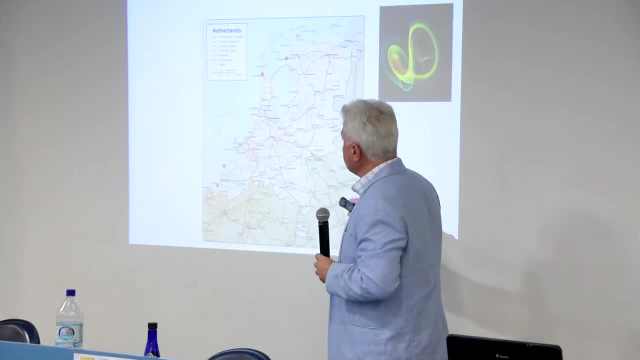 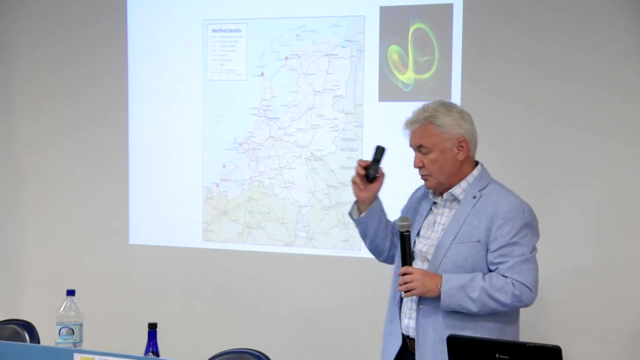 They're too big. So we're running neural network and chaos modeling. nonlinear modeling system to predict surge at this point, using data collected in the ocean every 10 minutes. Every 10 minutes, Dutch measure pressure, temperature, wind and surge. water level in the ocean. 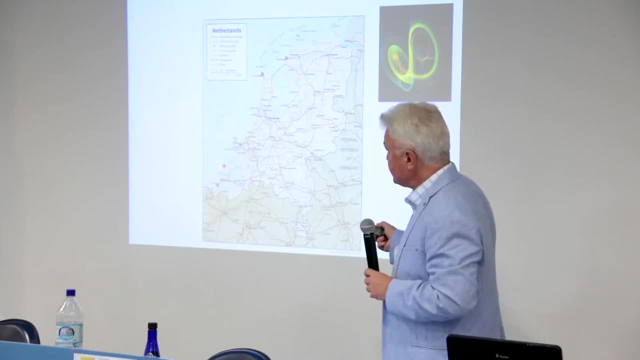 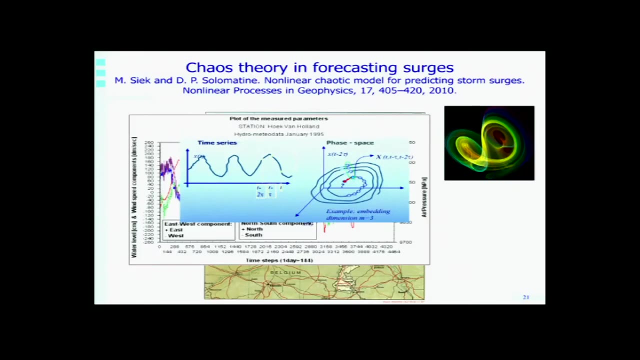 So what we can do, we can predict eight hours in advance the water level at this point. Okay, this is too much, We don't have time to do it. So, actually, what we do, we move time series into phase space domain. 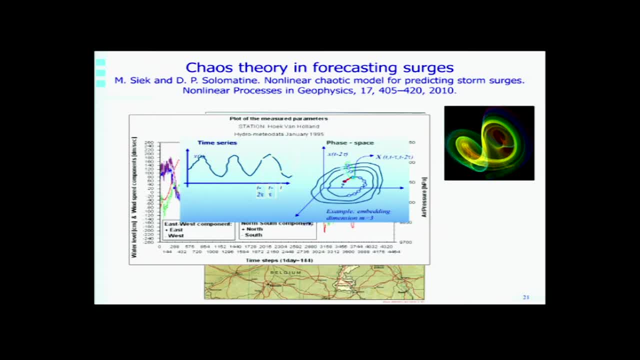 And we build chaotic model over here And then predict not in time domain but in phase domain. So we take neighboring points from the past phase portraits And red line shows you future state of environment here And for us environment is the surge water level. 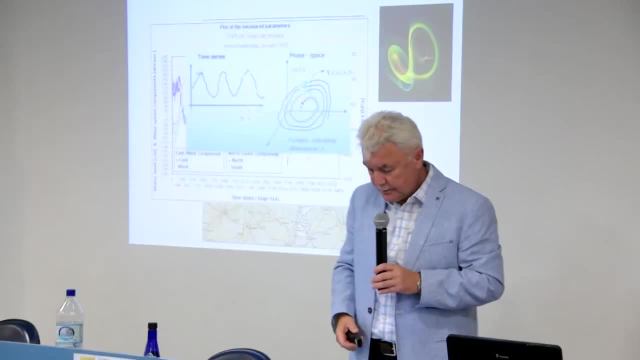 That's what we're able to do. There were two PhD studies in this. It's a pity Deltares didn't pick up this research. We tried to promote this, but somehow I'm not sure. They said we invested so much in numerical models that we cannot switch to different types of models. 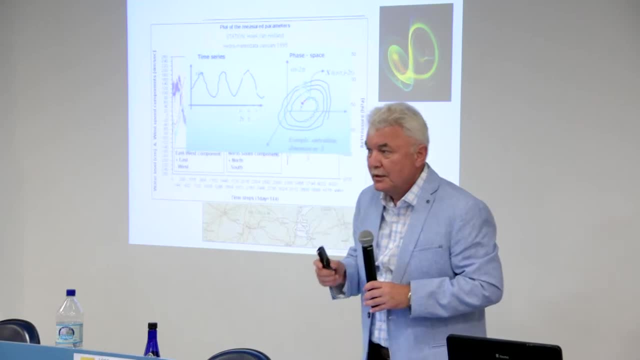 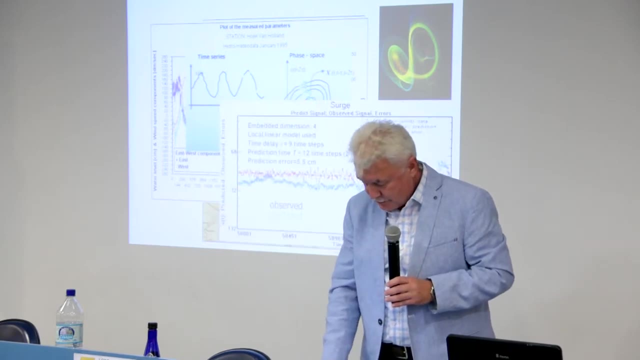 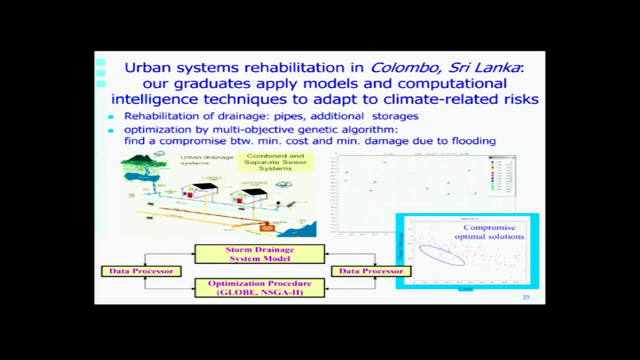 It's a pity. It's an example for me was that the uptake of research is not always easy. So but okay, research was done. Okay, let's skip this Now. Colombo, Sri Lanka, Urban system rehabilitation. So they want to change some pipes to better pipes so that they would have less floods in Colombo. 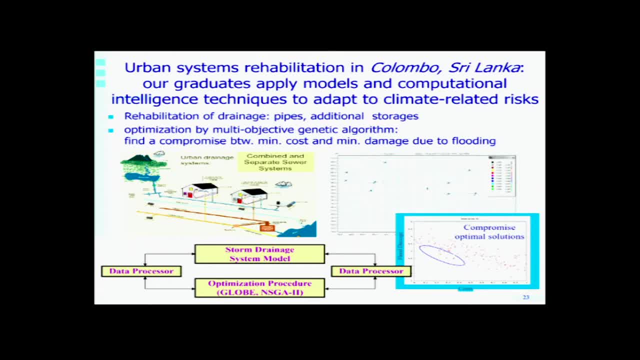 What to do To run optimization tools. So what we do? we run optimization procedure here And we run storm drainage system model And we do it in a loop And then we end up with a better urban system using computational intelligence tools. 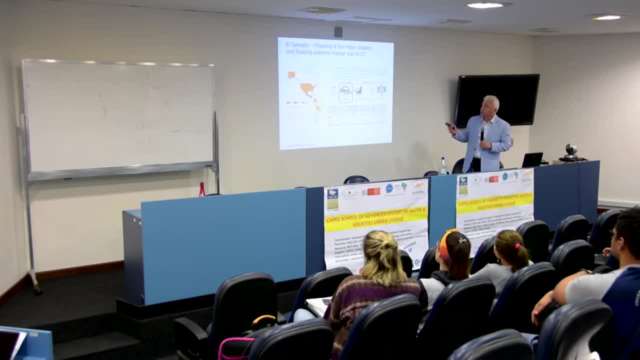 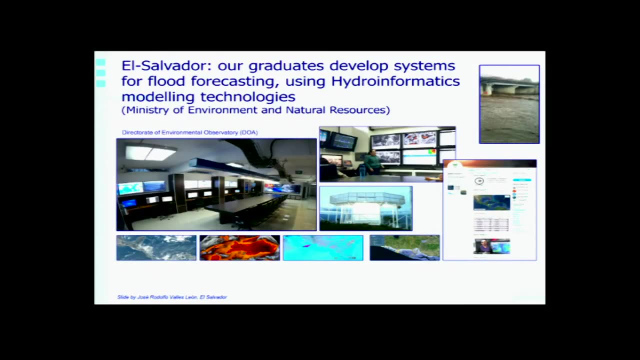 El Salvador, Flooding is a major disaster. So what our graduate did? he developed neural network model to predict flood situation for Ministry of Environment and Natural Resources in El Salvador. So it's not that he built all of it, It's a center. 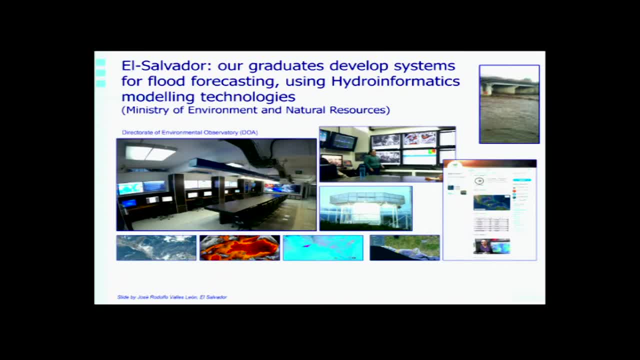 It's a center in El Salvador. It looks like this. It's great. actually It's high tech, Very nice. They run different models, But what he did? he developed neural network model. that they never did And it works. 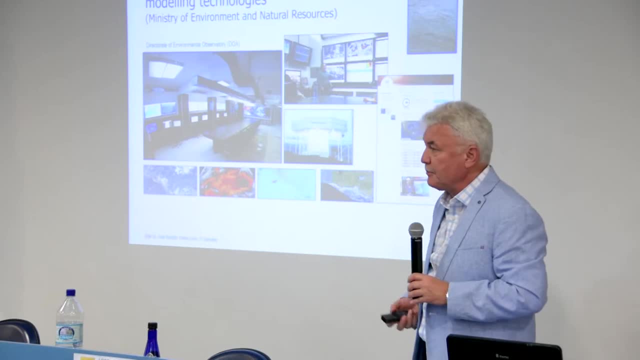 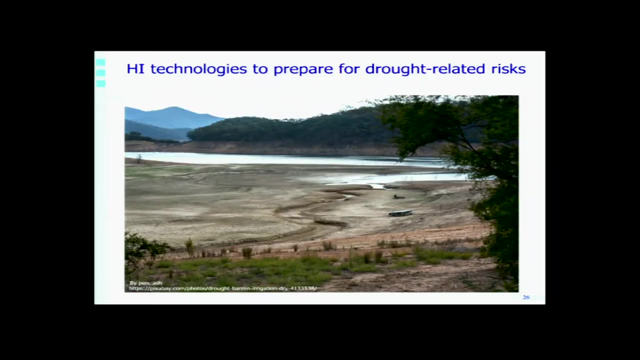 In real time it predicts floods, So I'm really happy to see it. In Holland we don't have it, And they have it in El Salvador, So that's great Droughts. Sometimes there is too much water. 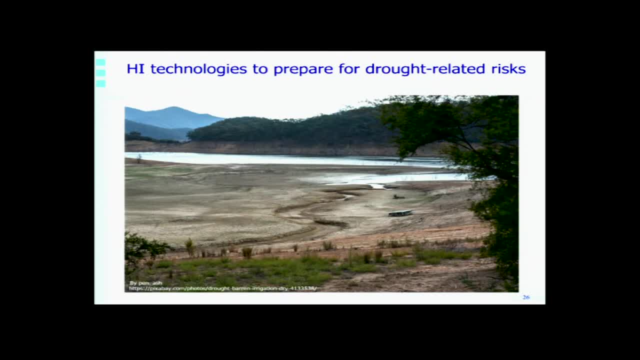 Sometimes there is no water, So we have a drought, Climate change and all this stuff. So droughts is not a result of climate change. Droughts were always like this And we observe them And we can use past data actually to think more about these droughts. 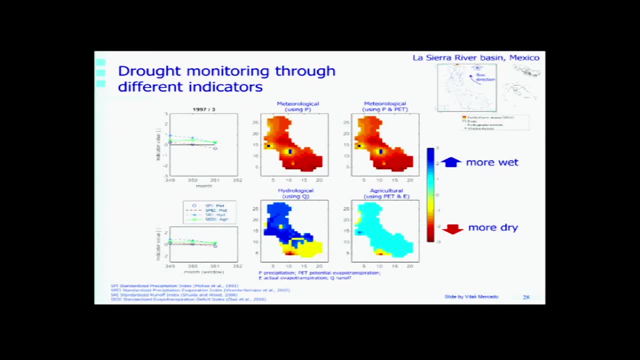 Okay, Let's skip this one. So one of our PhD students doing this, now from Mexico, And we look at different indicators: how to measure meteorological, agricultural and hydrological droughts using the world data. So, because there is a lot of data, 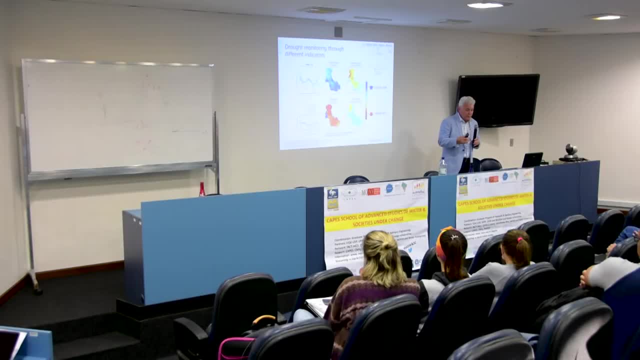 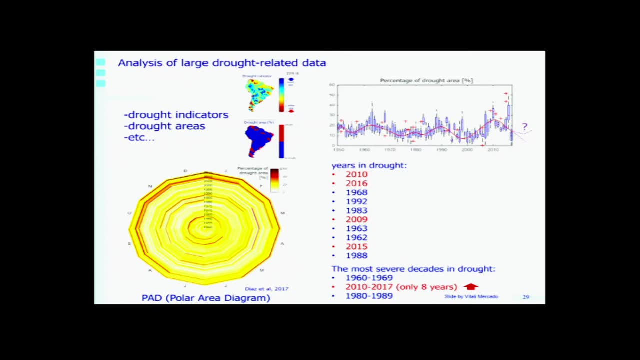 And what he is doing. He is trying to build analytical tools for better representation of droughts and better forecasts. So, for example, this way, if you move from time domain into so-called phase domain, you can see that you know drought system is developing like this. 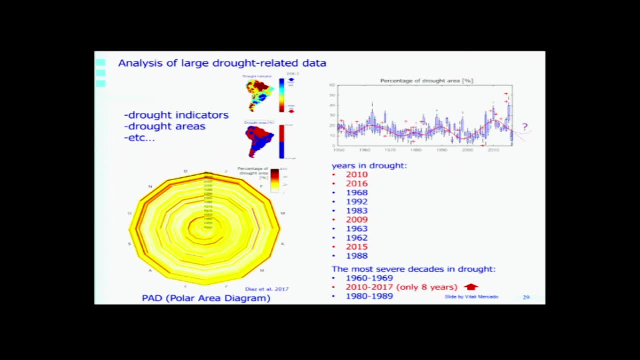 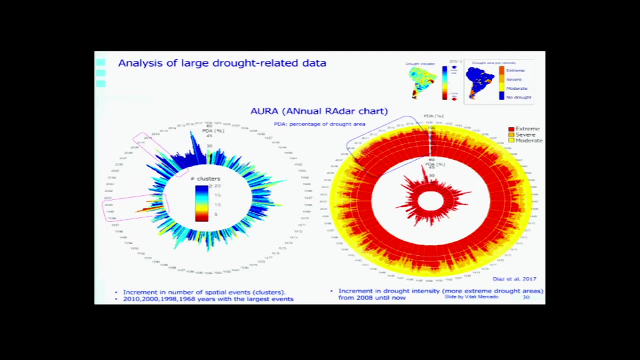 So we have more droughts in the world than in the past, And this visualization tools actually allow you to show that number of areas and areas in total increasing when we think of droughts. Okay, He is using different visualization tools, So that's Vitaly's work. 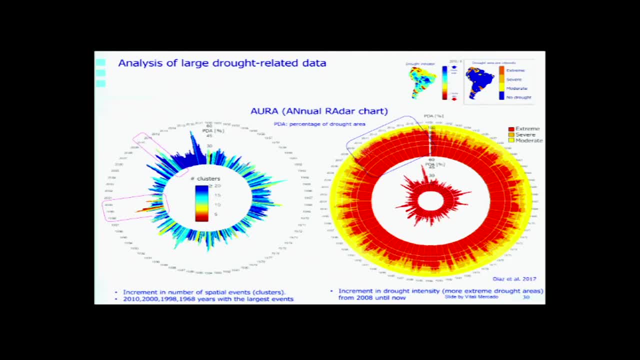 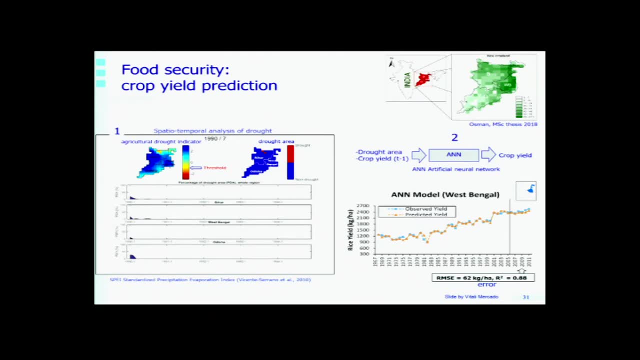 So I will not go into details. I just want to show you that it's a lot of drought Now. also, one of our master students built neural network that is predicting the crop yield. due to drought, Crop yield could go up and down. 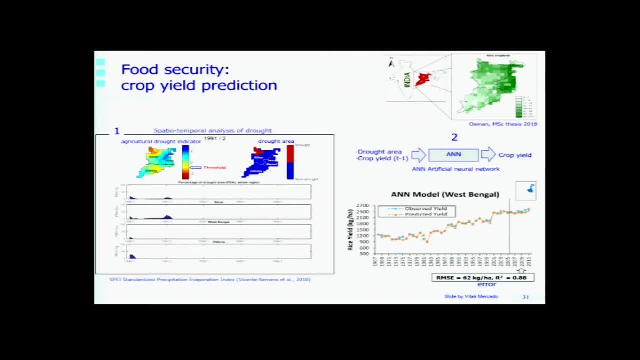 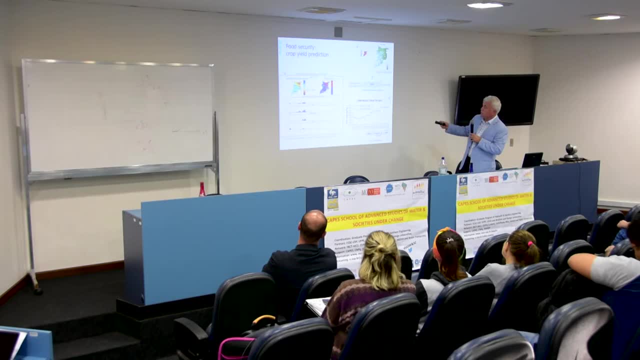 It's in India. You see this area. So, in fact, neural network was able to predict quite accurately the yield And we can see that. We can see the yield in years. So these are years from 1967 to 2011.. 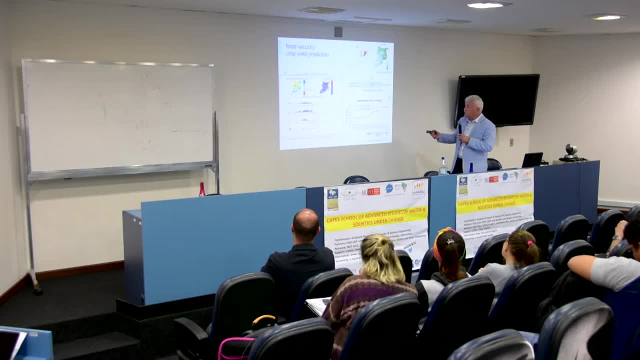 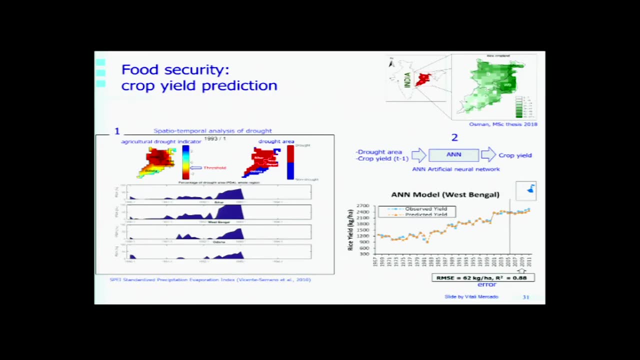 So we're quite surprised to see quite an accurate result. Maybe problem is simple because it's you know it's just to predict one value for the yield for that year, But still it gives you hope that even for more complex problems, data-driven models can be used in drought studies. 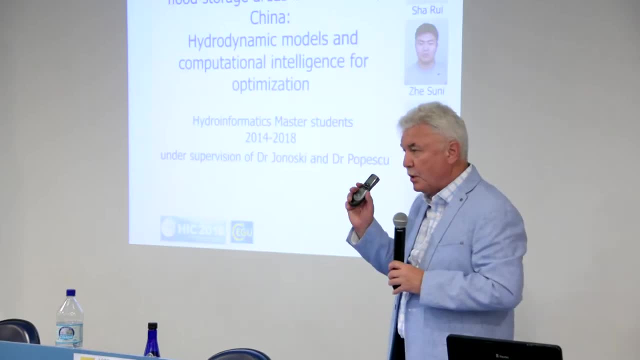 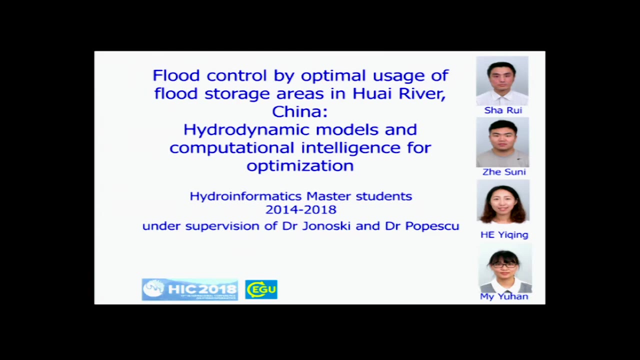 Okay, Let's skip this Now. I would like to show you one example of smart management in reservoir operation. In Brazil, You have a lot of hydropower, Itaipu and so on, So you know better than I do. 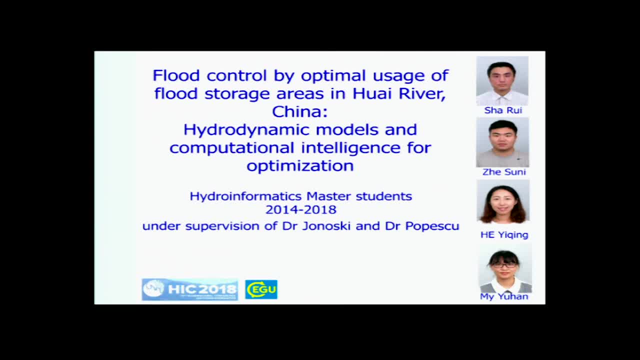 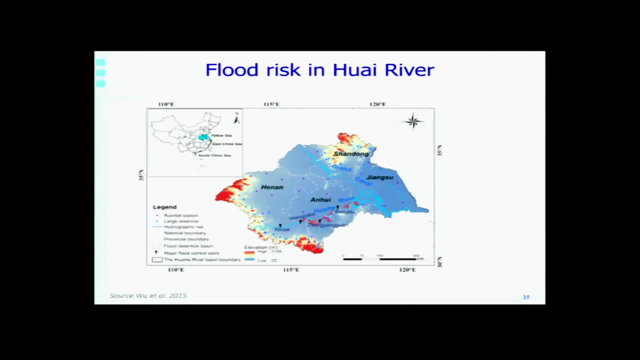 So what we did with these four Chinese students in several years? we're building flood control for optimal use of flood storage areas in Huaihe, using hydrodynamic models and computational intelligence for optimization. So the problem is this: In Huai River, which is a river basin, 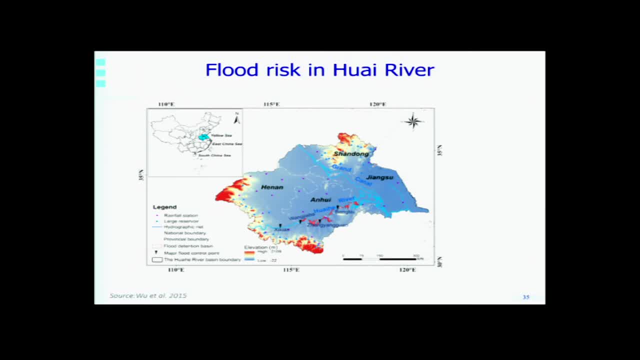 This is China, So this is Huai River basin, And, okay, let's move to a better map so that you can see it here, Right? So here you have upstream, fast flash floods in this area, River flows like this: 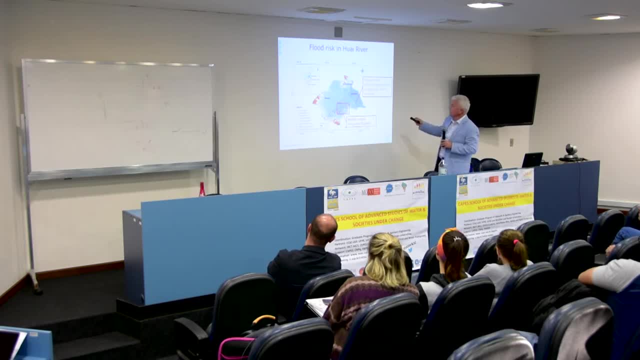 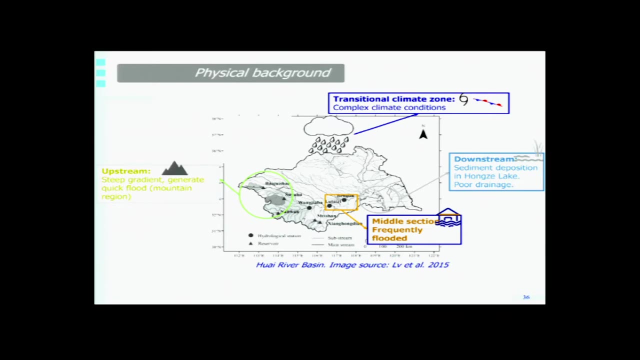 Middle section frequently flooded And downstream there is a sediment deposition in Hongsu Lake- poor drainage, So they have different types of problems along the Huaihe River. We concentrated on this area over here And what happens here. let me see if I have a better map. 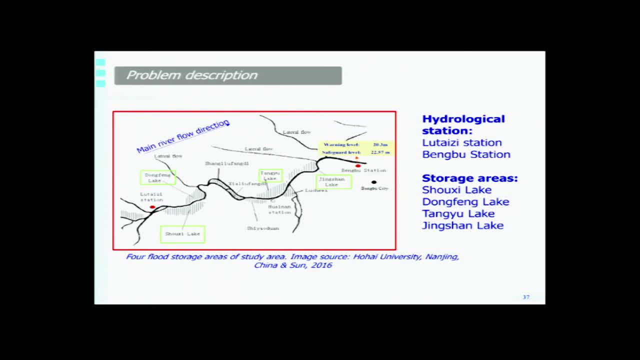 Yes, So in this area. So what we have here is this. So water flow is this way: There is a big city of Bangbu, several million people, And it's frequently flooded. It's flooded because too much water comes from upstream. 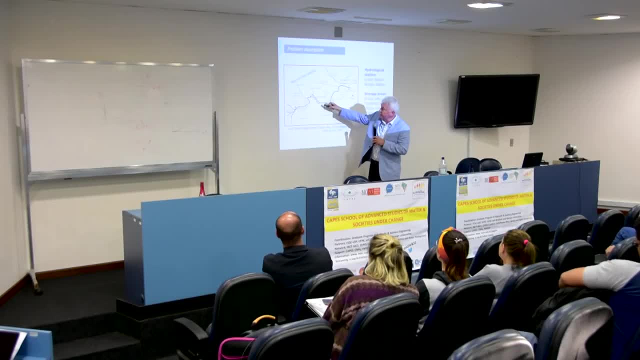 So solution is to flood certain areas here. you know, before this, water volumes would reach Bangbu, So Bangbu flood would be lower. Problem is, of course, there are 200,000 people living in these areas which are flooded. 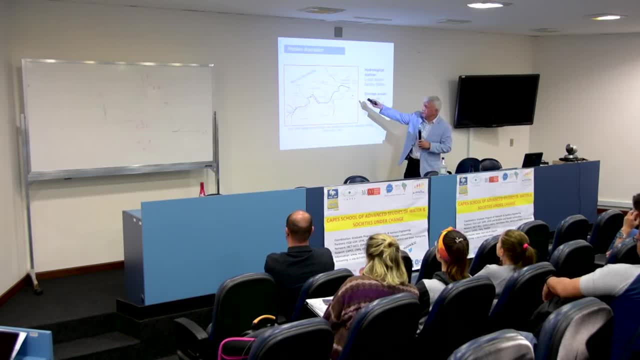 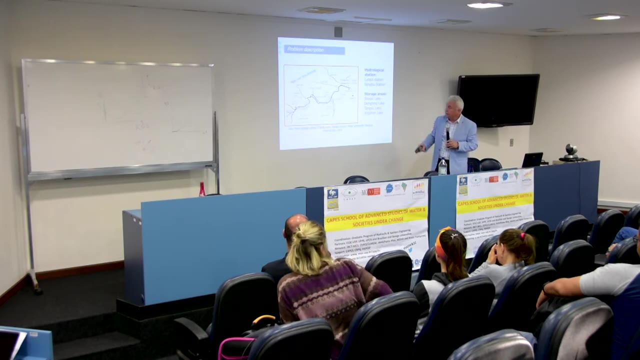 Okay, So it's a compromise. Of course, the officials live here and they want to minimize flooding of their houses, So there should be compromise found. So what we did? we built 1D model of this river. We also built with students 2D model of this river to look at flooding. 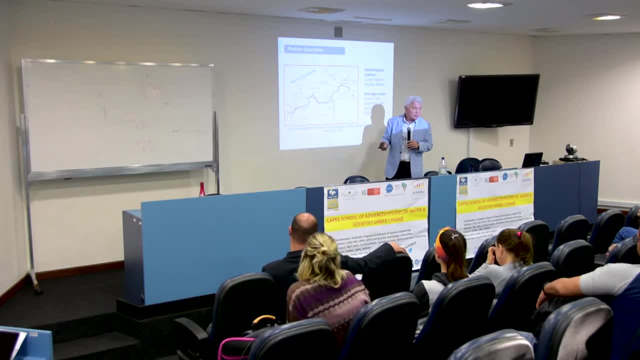 Because we wanted to assess the damage. So for this you need two-dimensional modeling of floods, The damage here and also in Bangbu, And also the main problem of optimization is this: When to open this detention areas and when to close them. 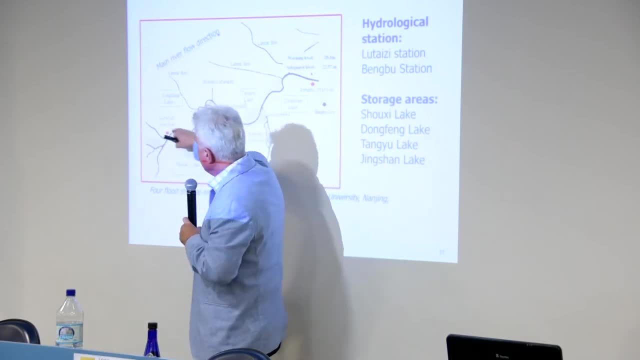 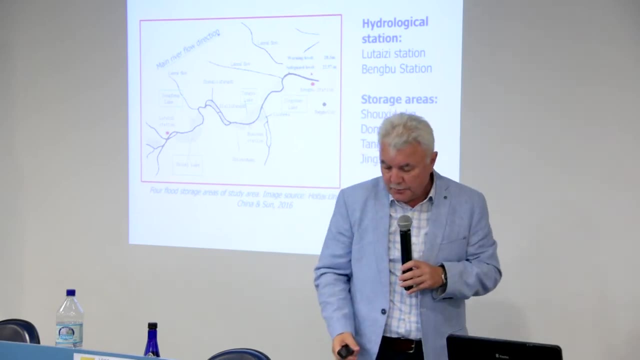 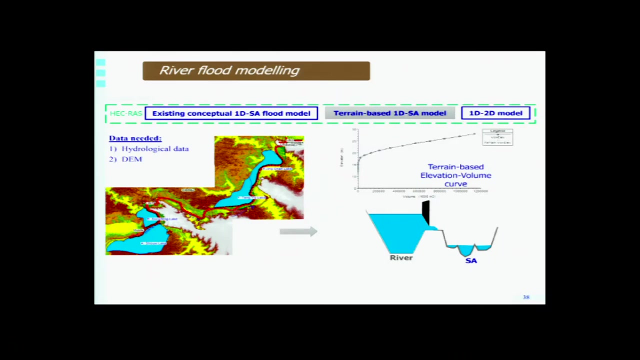 So that for the forecasted inflow of this river, you would have minimum possible damage here and minimum possible damage over here. So it's multi-objective optimization problem. Okay, It shows some inundated areas and so on. I will not go into detail. 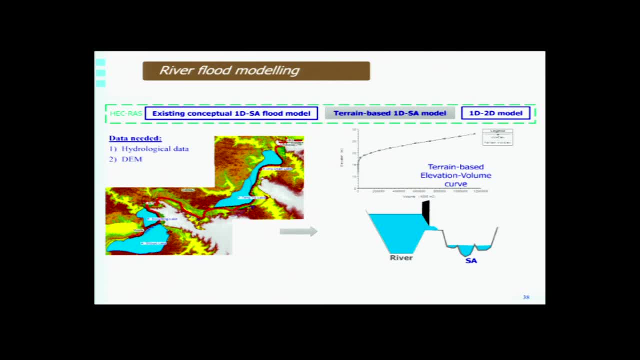 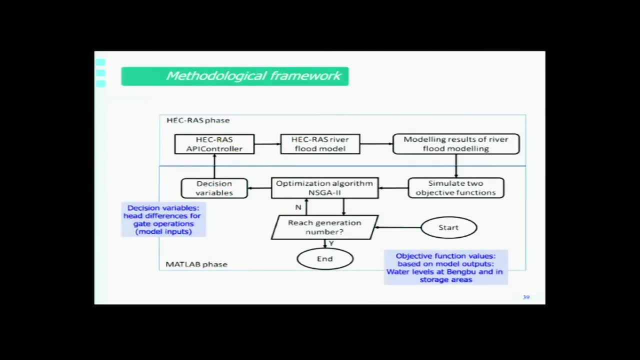 So we used 1D model. We used also 1D- 2D model, So it's 2D model actually, And all of it was integrate, modeled in an integrated fashion, And then we used optimizer over here. 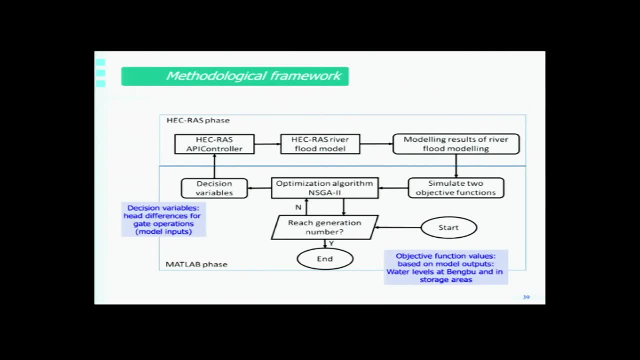 So multi-objective optimization routine and this GA2, but also used other algorithms That would run this model, generating every time different schedules of opening, closing all these gates. So decision variables is this timing of opening, This timing of open, closing? 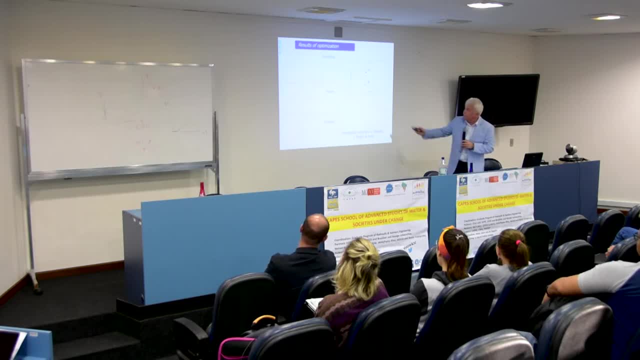 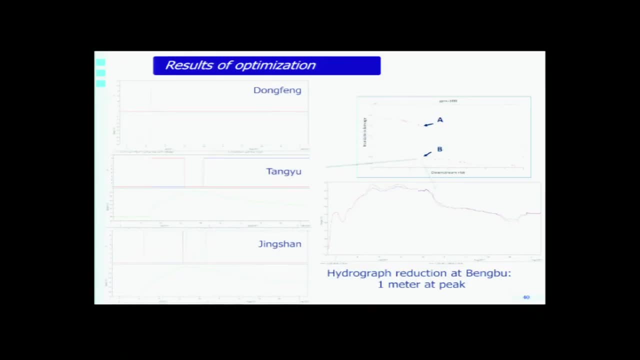 So our objective was to generate then Pareto set. This is the Pareto level. So this is downstream risk In Bangbu risk already including damages, And this is inundated areas damage upstream And we want to find this Pareto set of all solutions generated, with 1,000 solutions generated. 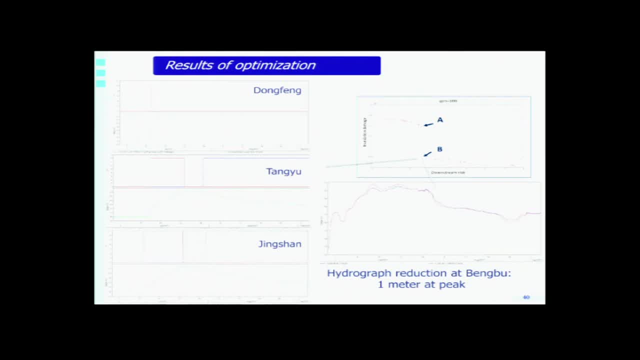 So this one's a lot of damage upstream but no damage downstream, When you open all gates and keep all the water upstream, but then you have a lot of damage upstream And this is almost no damage upstream but a lot of damage in Bangbu downstream. 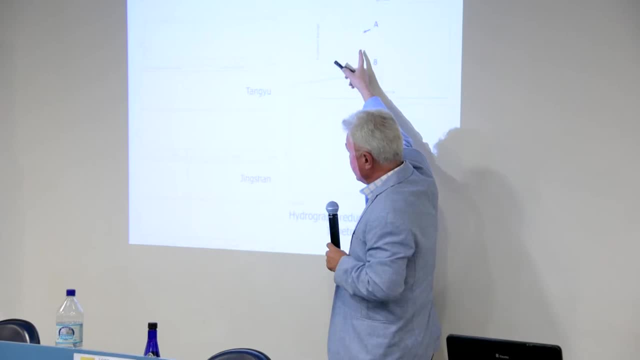 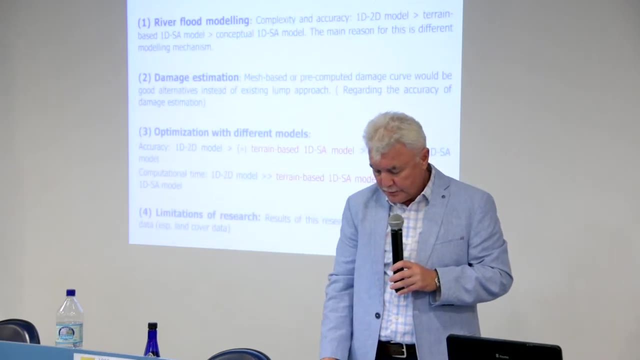 So people are not here, So we have to find some compromised solutions. So analysis was also which one solutions is to choose from this Pareto set of possible options for water control. All right, So it's a nice example. 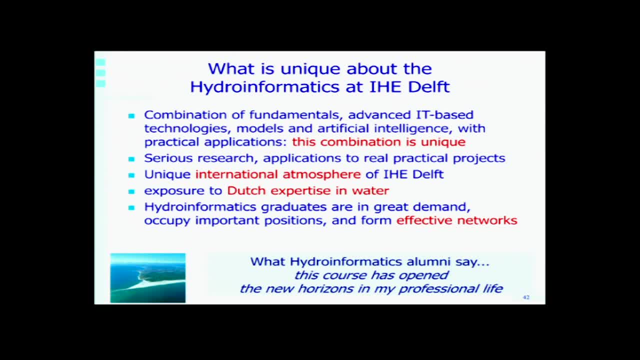 When several students worked And we used quite sophisticated technologies. So what is unique about hydroinformatics and IHE-DELF? So let me get to conclusions. So we think we're able to combine fundamentals, advanced IT-based technologies, models and artificial intelligence with practical applications. 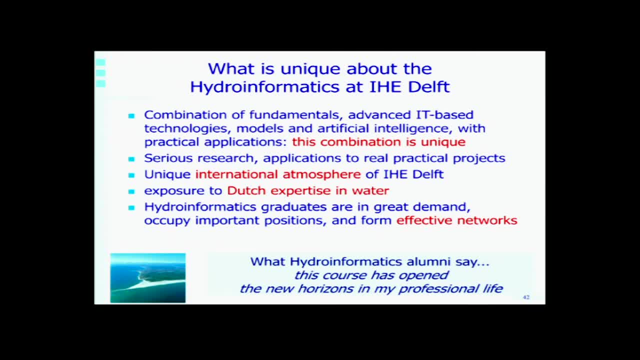 And in my view it's a combination that's unique. We have wonderful courses in theories, very much maybe courses in practical, but we try to combine this. Now. we do quite serious research And we connect through our partners and through our students to practical projects. 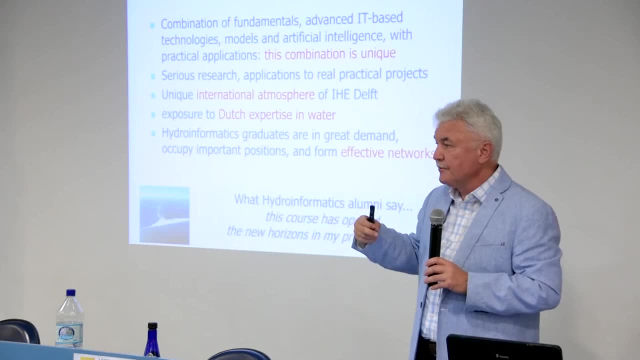 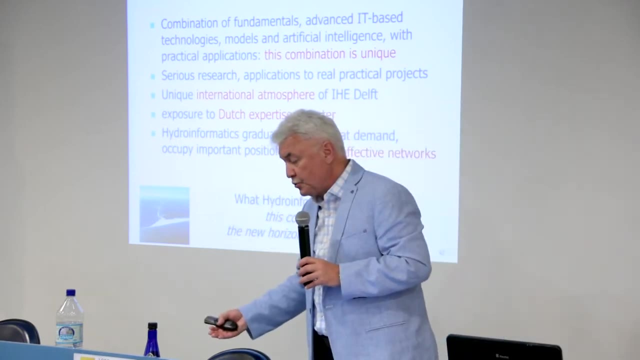 You have to realize that our students are not fresh graduates. All of them- most of them are already experienced engineers or managers, So they bring also problems to us which we want to solve together, And we learn a lot from this, our participants. 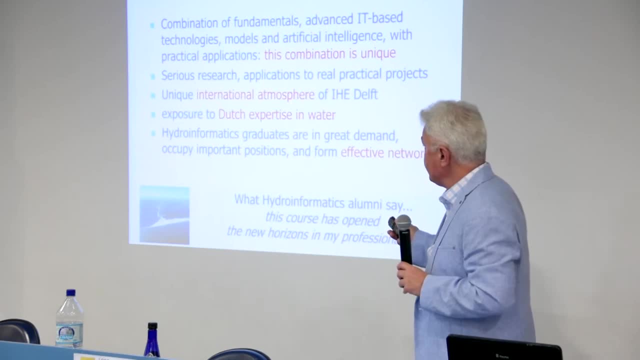 So we have nice international atmosphere. That's great Exposure to Dutch expertise in water. And again, our graduates. Our graduates form the effective networks for the future Because they occupy many of our graduates from IHE in general Now deputy ministers and all this. 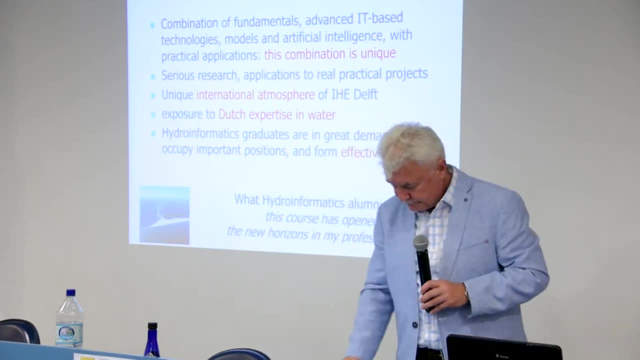 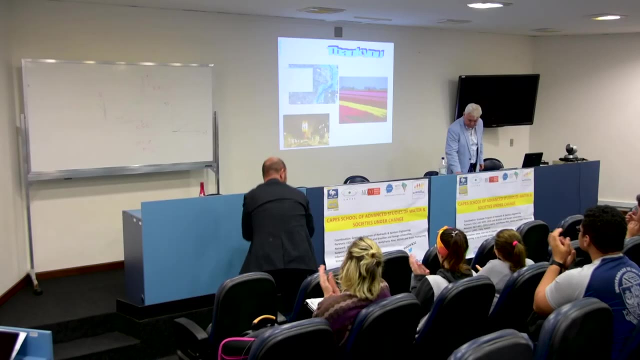 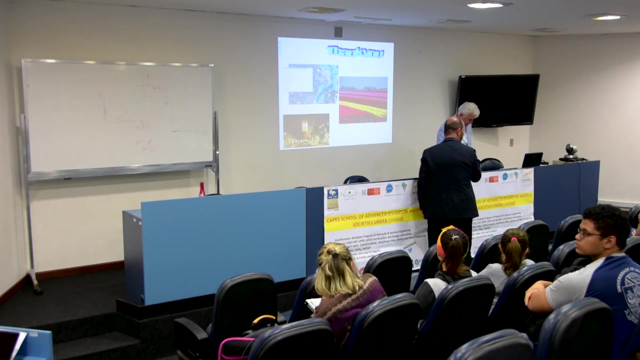 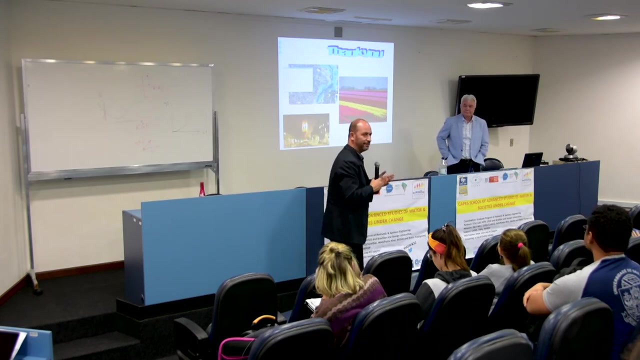 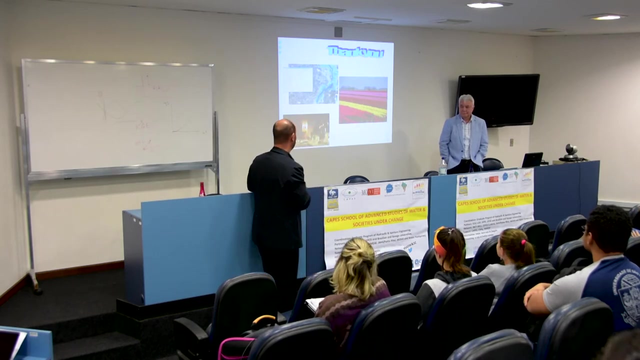 So it's good stuff to do. Thank you, colleagues, for your attention. We are going to take some plenary questions Because it's a motivational lecture with several examples around the world. Also, the Delft flag is in all these examples. 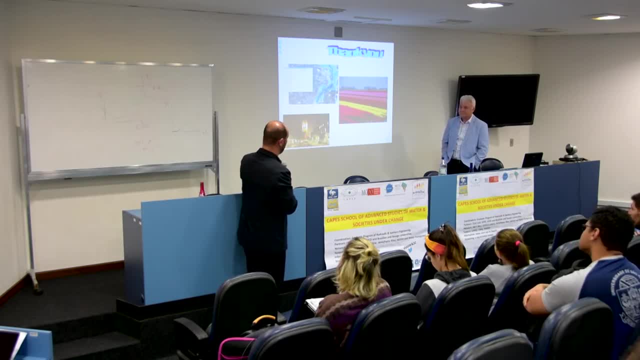 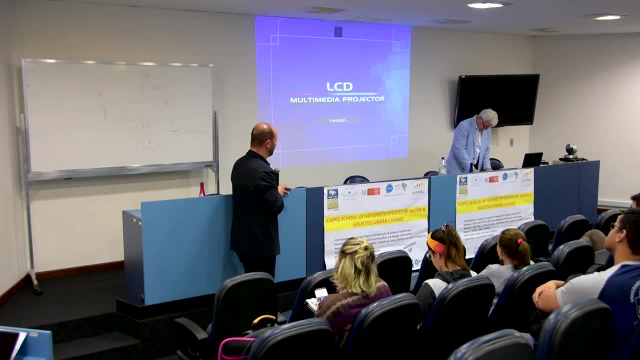 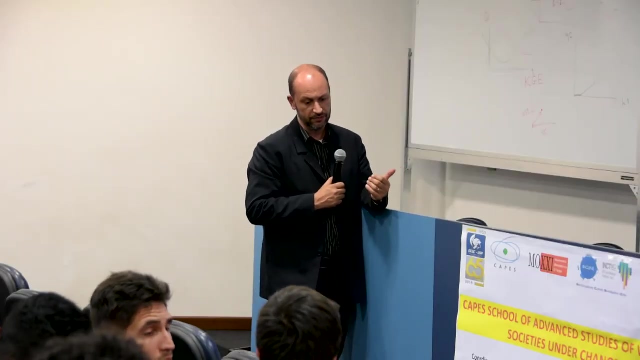 I would like to return to perhaps the first slides, when you mentioned the framework of joint programs. You are just starting with another institutions like South America, the Colombian programs, And also with the European programs, So I try to take the feeling from our graduate students here. 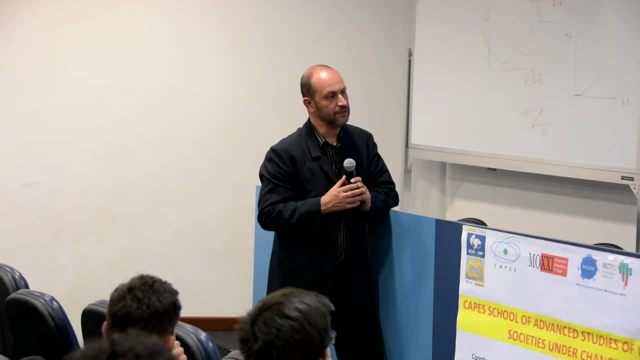 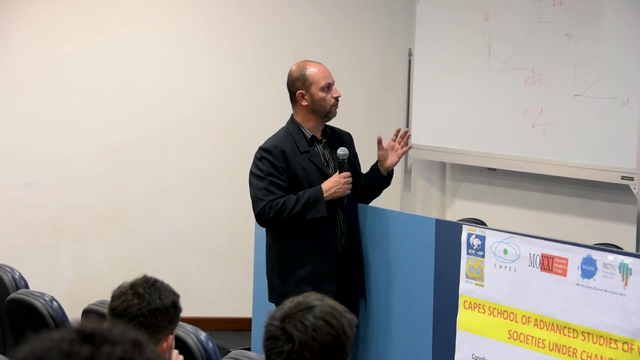 So what are the eligibility criteria you have in this case to select students? of course, This is the normal question: What about the costs? But also, as a researcher and a scholar, I would like to know more. How do you shape and combine to start a joint program? 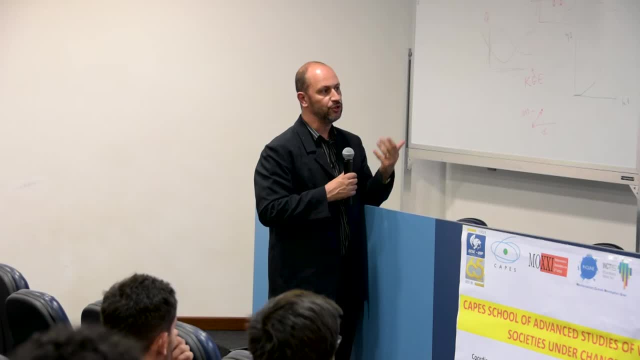 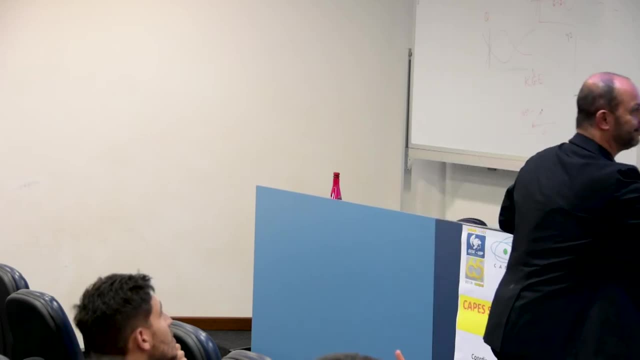 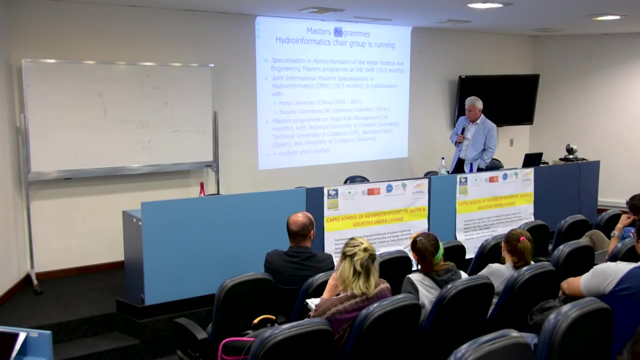 What are the eligibility criteria for new or another graduate programs to join perhaps new joint ventures with you? Thank you, Yes, good question. So there are several, So one: We accept students with bachelor degree in general for all courses at IHE. 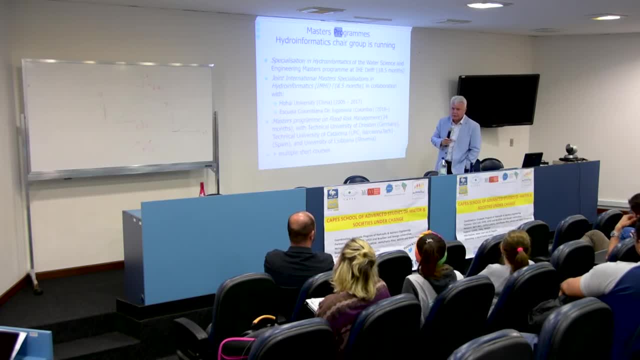 Bachelor degree, ELTS test 6.0, I think. So English of course should be at certain level, And you know, we say diploma from University of good standing. But okay, So it depends what you think of good standing. 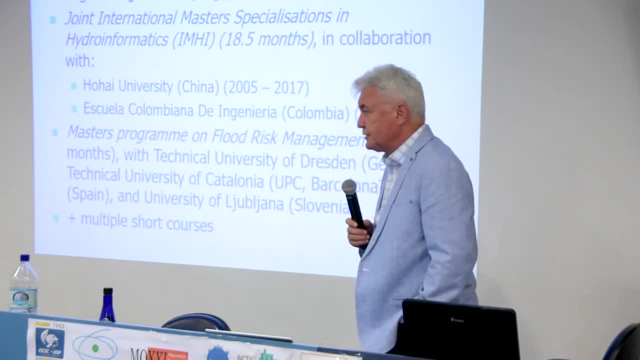 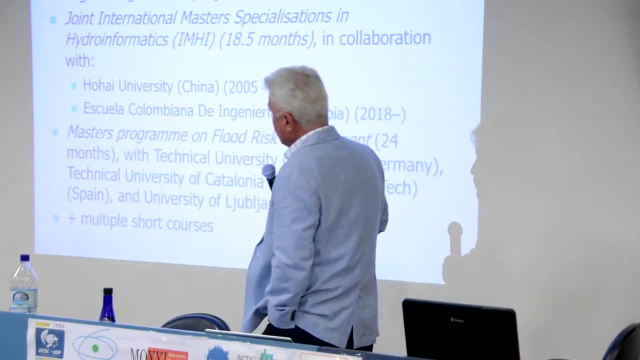 So we have many applications. Also, we look at motivational letters. You know we want to students that would manage this course. This course is not easy And maybe one hour course is one of the most difficult because there's mathematics there and you know numerical methods and so on. 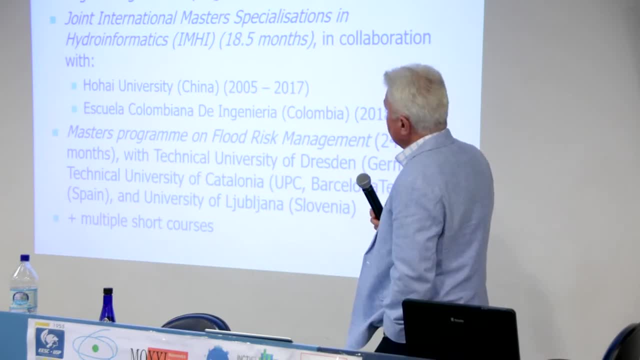 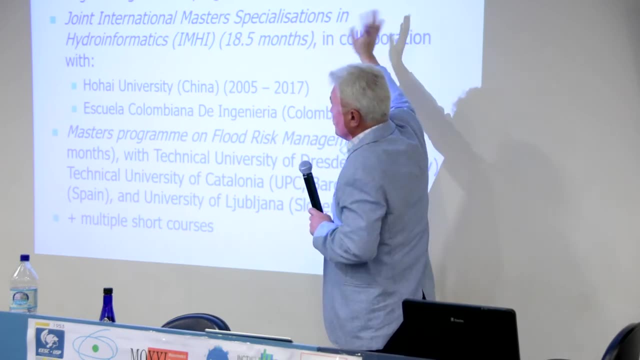 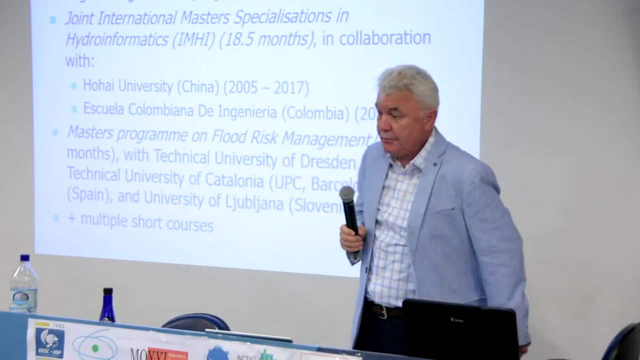 So computer science? Okay, That's one, But it's true for all programs at IHE. So also this normal program of specialization, hydrophilic, which is not joint, It's run only by IHE. Now, joint programs- we look, it's happening that our graduate is professor at Ohio University. 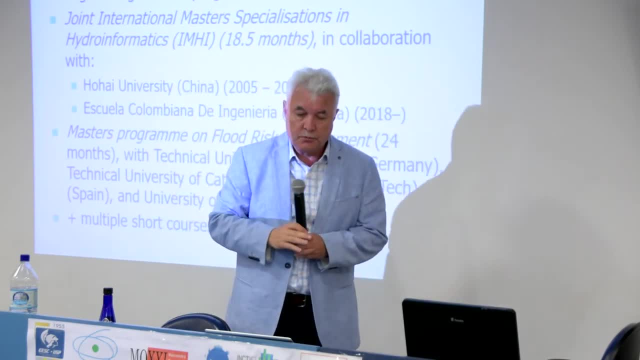 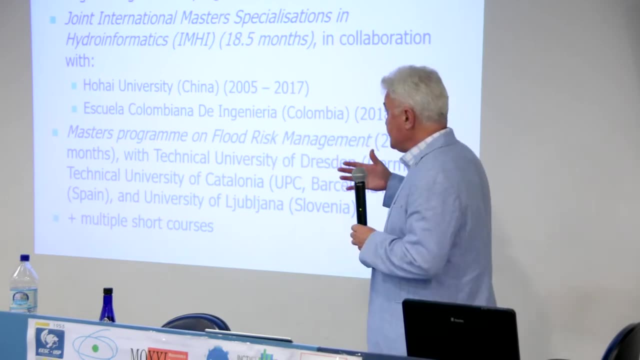 And at a certain moment we thought: why don't we start a program where people would spend some time in their own country, Which is also maybe easier for them because they wouldn't leave the country for one and a half years, So they would spend some time at home still? 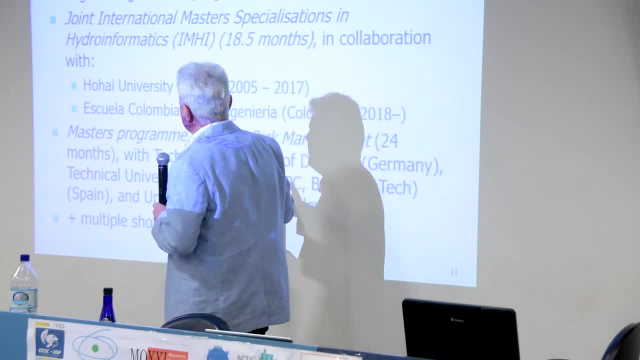 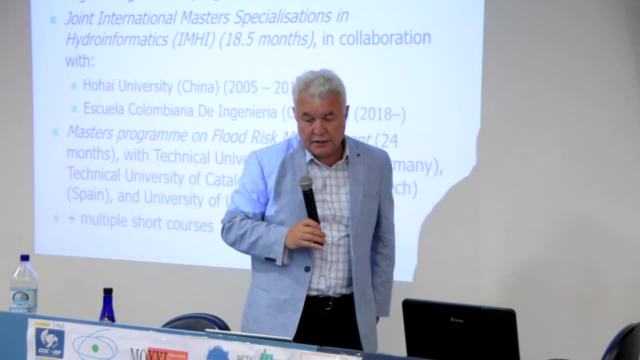 Also it's cheaper, because living there could be cheaper than in Delft. Okay, And why not? So we tried with Ohio. It worked partly, But for ten years we, and still we have ten, sorry, five, seven students. 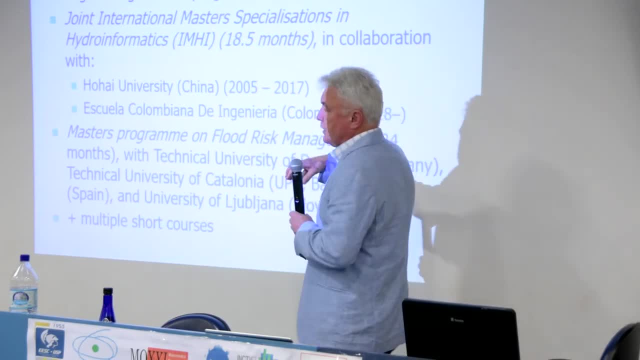 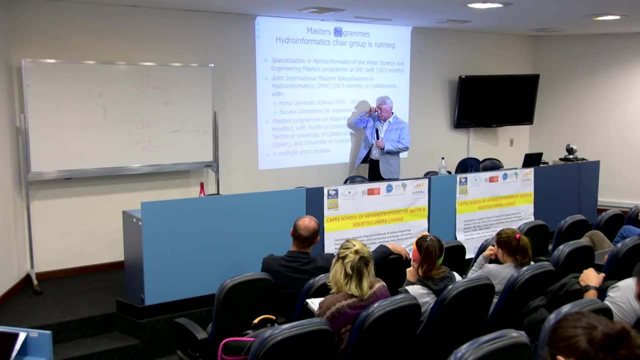 Okay, Five, seven students from Ohio only for hydrometrics course and also some students for other courses. Problem was that to what's the word Accredit? this program in China is not easy because for them it should be a new master program. 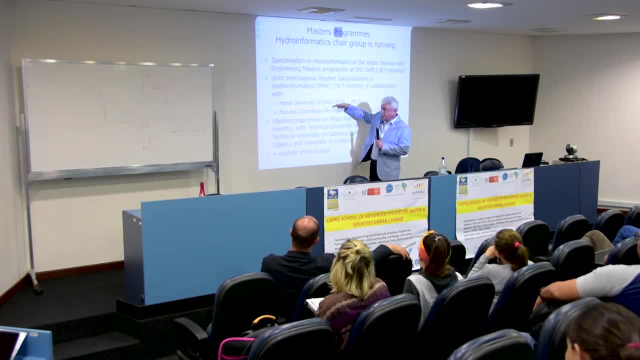 So it didn't work out. So now we stopped this thing. Still, students are coming, But it stopped in 2017 because they didn't manage to accredit the program. People changed, So that was this thing. 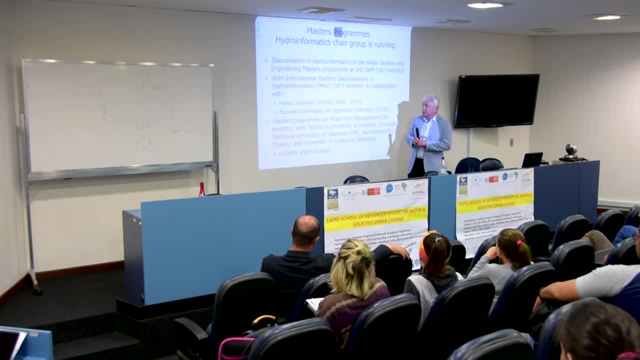 Escuela Colombiana. So Gerald Corso, Okay, Because he graduated from there and he knows people there. Again, it depends on the people there who are enthusiastic And they wanted to have this joint program for two years so that people would start in. 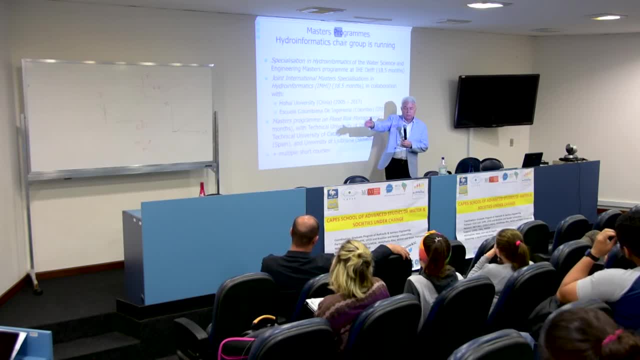 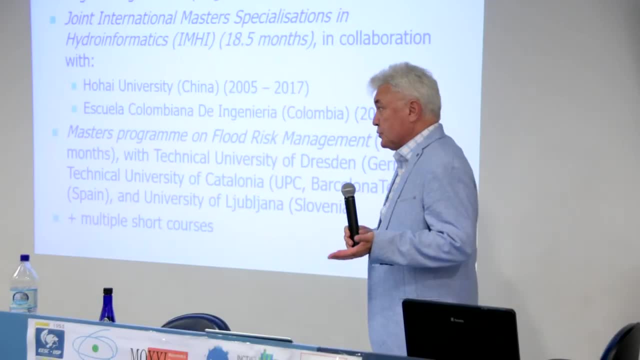 Escuela and then come to Delft and then either do MSC in Delft or in Bogota. So that's So. how do we choose this partner? Because we trust these people. That's most important: the trust. 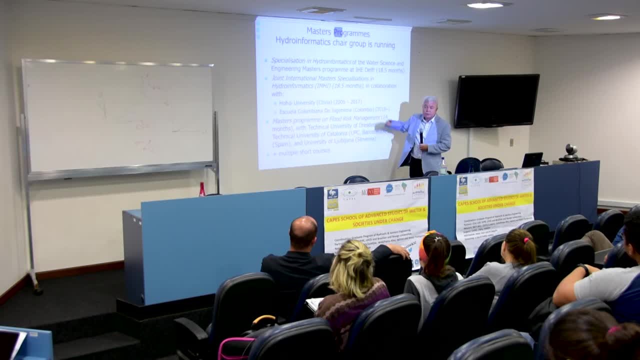 And also enthusiasm and interest of them to do it. And about this thing And about the fees: Fees is a difficult issue. So cost of our program right now only tuition fee is around 21,000 euros for one and a half. 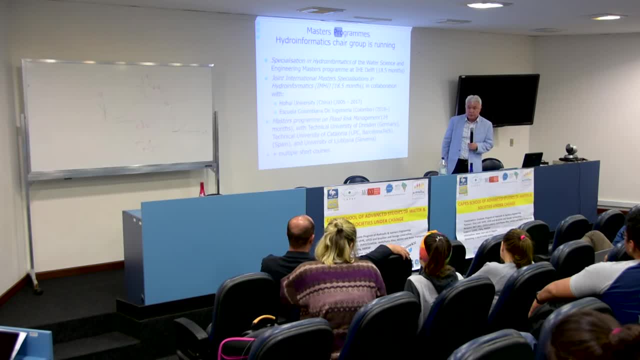 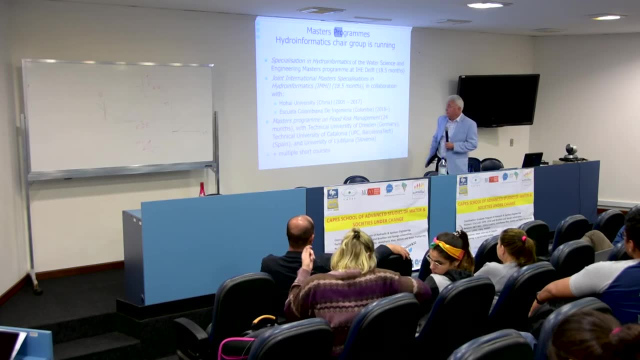 months plus living expenses, which is 1,000 euros a month. So that's You can add up, It ends up almost for 40,000 euros. So it's a lot of money. Now, fees then here, when they're in Colombia, are lower. 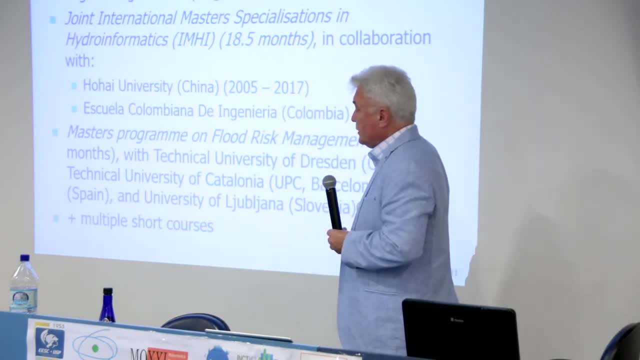 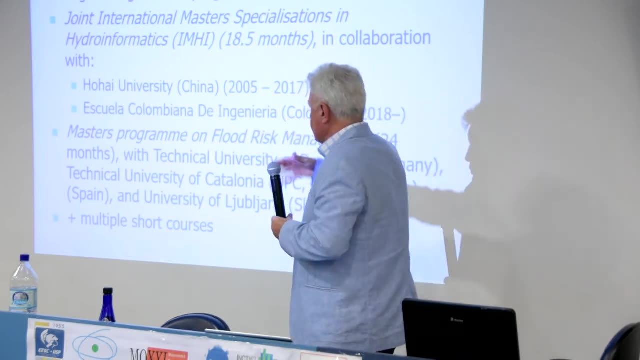 So then there is an equation to calculate total fees: Partly in Colombia, partly at IHE, but diploma would be from IHE, So IHE handles all this. So somehow it's becoming a bit lower. Yes, indeed, 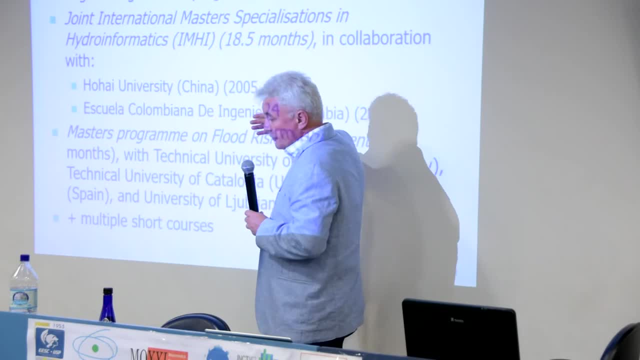 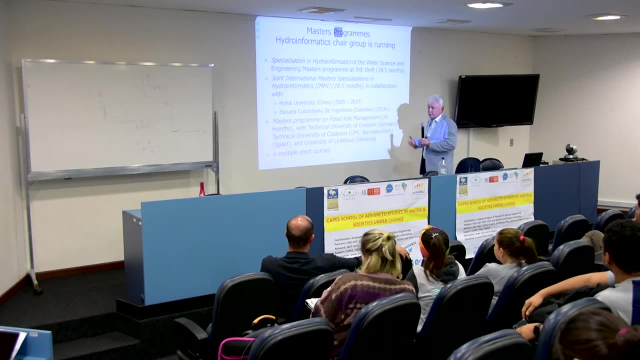 But in Colombia they got call sciences and call futura, who are able to provide students with money to study in good universities. Somehow they're funding their studies well. Strangely enough, fee was not a problem at that moment. Problem was organizational. 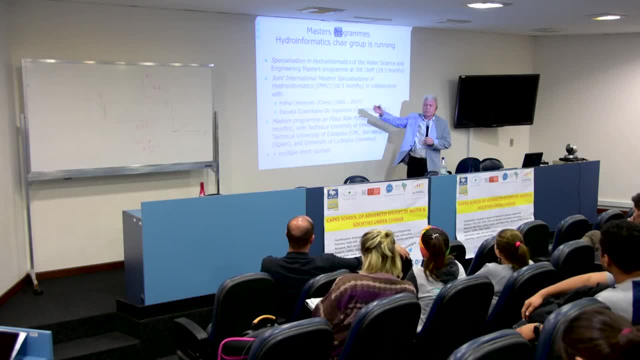 How to organize all this. It's not easy because staff should be there. It's not easy because staff should come from computer science department. They don't know how, and all this. So it wasn't easy, But now it's moving on. 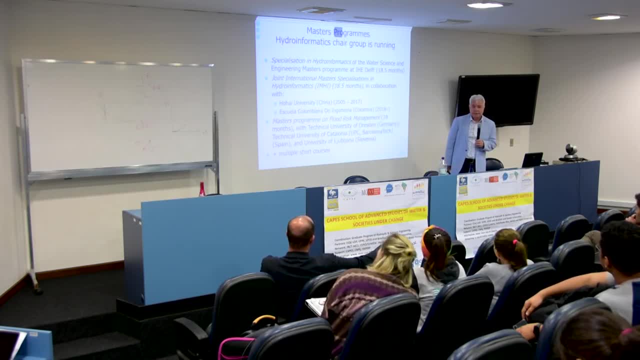 So first students would be coming to Delft next year, No, this year already Yes. And the diploma is that double diploma? We used two options. This one would be two diplomas given: One Bogota, one Delft. 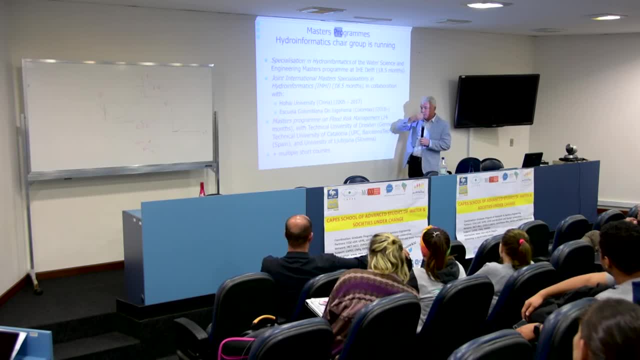 So we trust they give good education, They trust us, We give good education, So we credit, cross-accredit our programs And we give two diplomas. In this place we give three diplomas: One Dresden, one Delft and one UPC Catalonia. 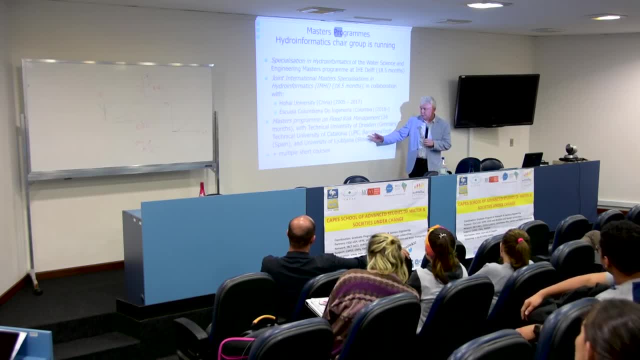 Ljubljana, not because it's only two months there, But maybe also, And the master thesis presentation is unique once, Once, of course. So some do it in Dresden, some in Delft, some in UPC, Some in Ljubljana even. 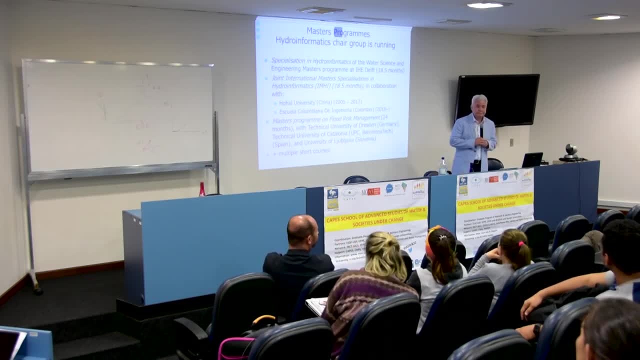 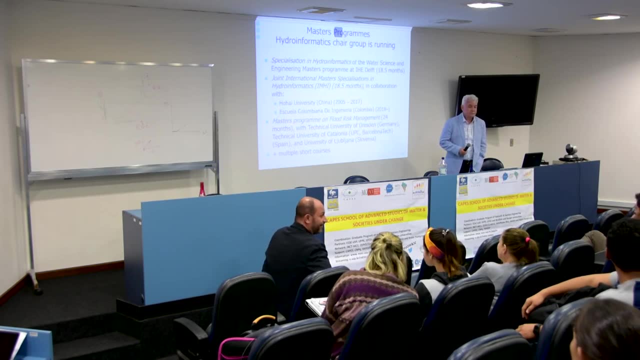 Yeah, Thank you. So quite complex arrangement. Any other questions? End of the day question is: when do we stop? Yes, I know People are tired. I tortured them. You're very, very tired, I'm not. 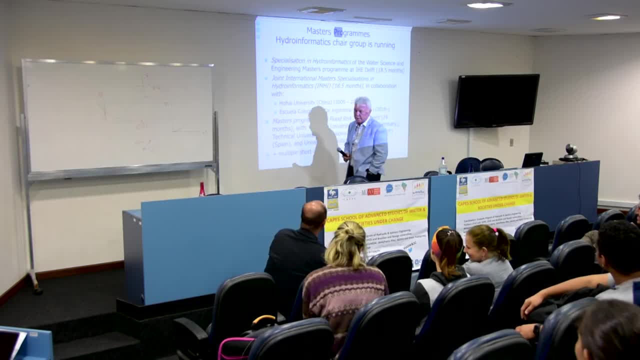 I could continue to. Really you are. You are Bottle of vodka. and I could continue forever. But I see on the faces of students: they're, you know, good. I tortured them and they're good. Really, thank you for standing all this. 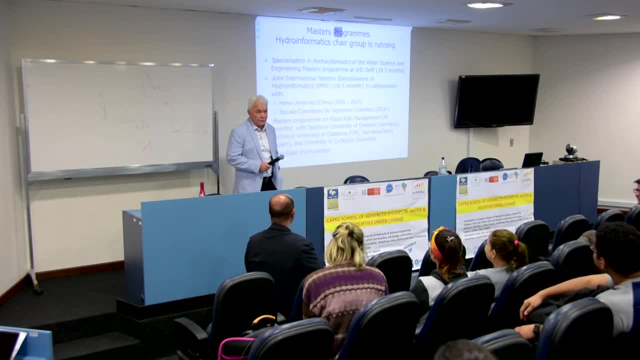 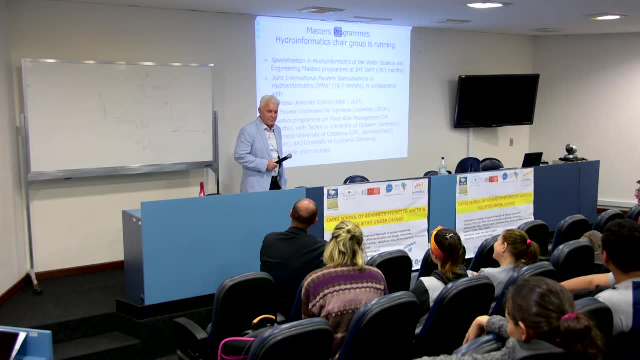 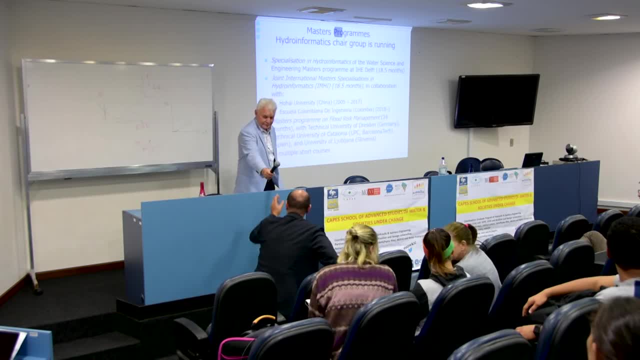 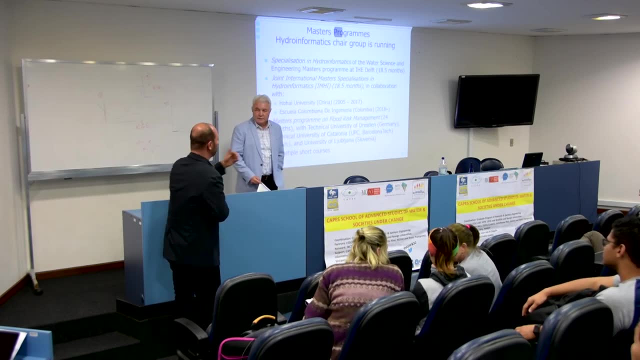 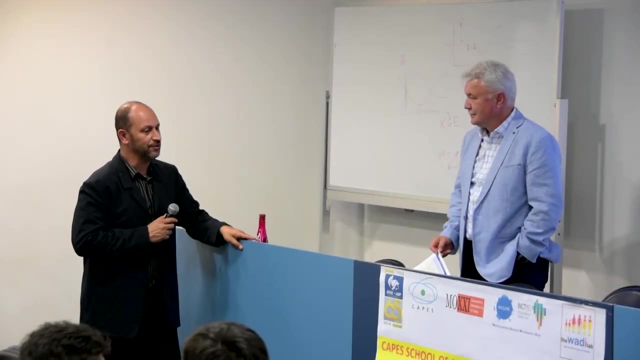 Only last question. This is a final, final question: What is your opinion of the challenge that you you presented? the microapp suivance, Yes, 30,, 50 years beyond, in the front, in the future, For the future? what's your expectation about integrating data, hydro, informatics and society? 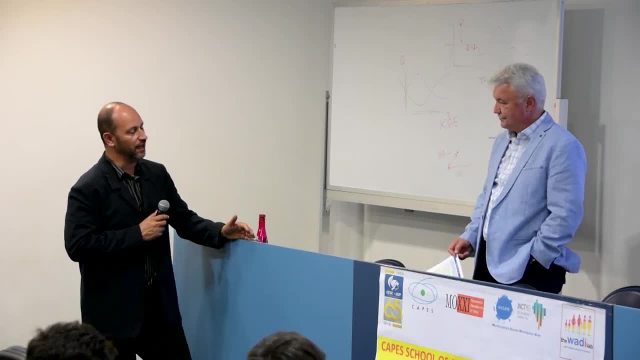 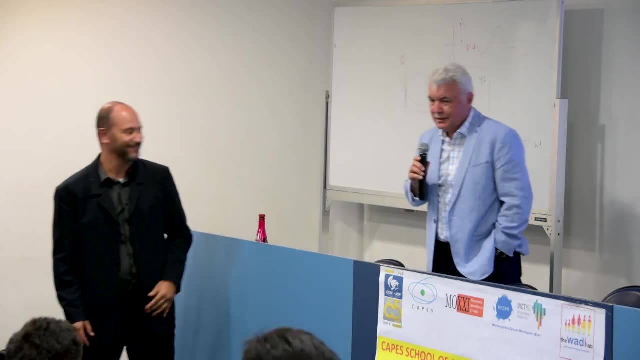 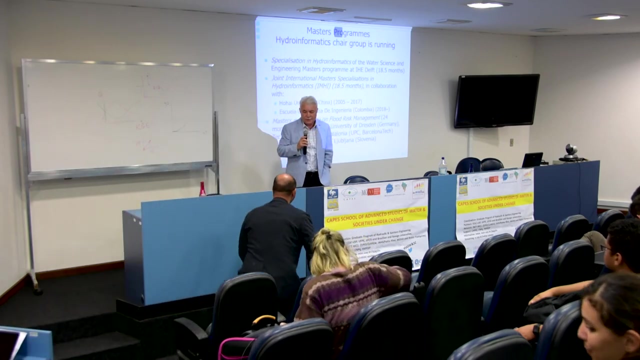 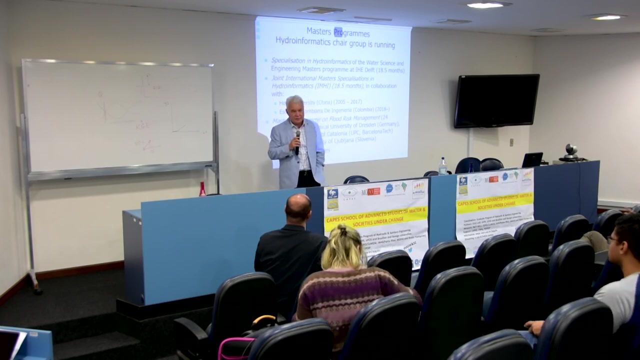 perspective perception, trying to help in measuring this is in a good direction of science, or perhaps it's only a wave. Yes, no, look, I think. I think society and science should connect better, because often science is done for, because we're curious in something and society doesn't accept it. 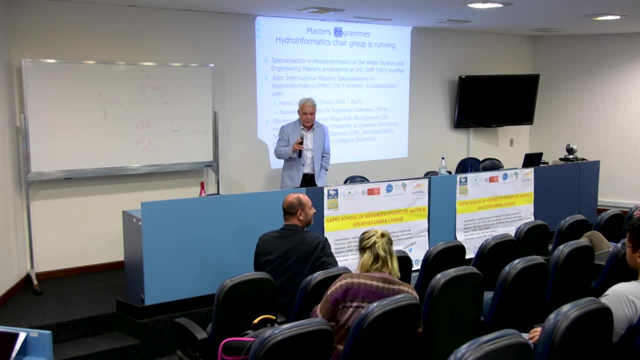 So this interface between science and society should develop much deeper, that's for sure. And it's not easy, because society doesn't understand science and science often doesn't care about society. That's a problem. But I think, look, science often does things which are not immediately used by society. 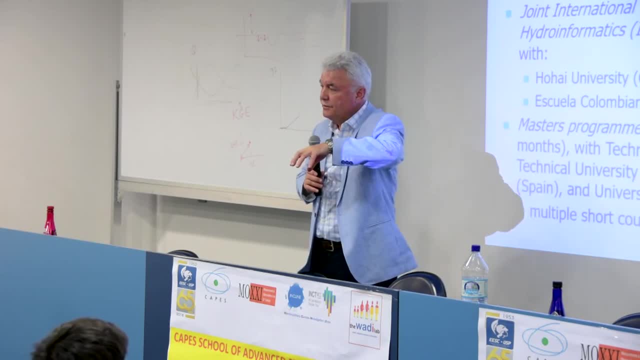 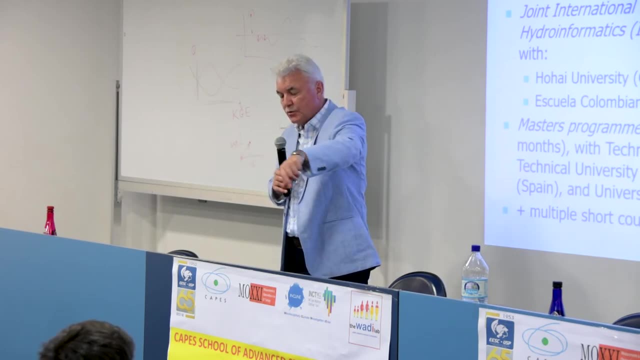 And I'm afraid it's inevitable. But however, if one-tenth of the science would do something that society would make a quantum leap. That's enough. So you can allow science to do things which are not necessarily used by, like mathematics.